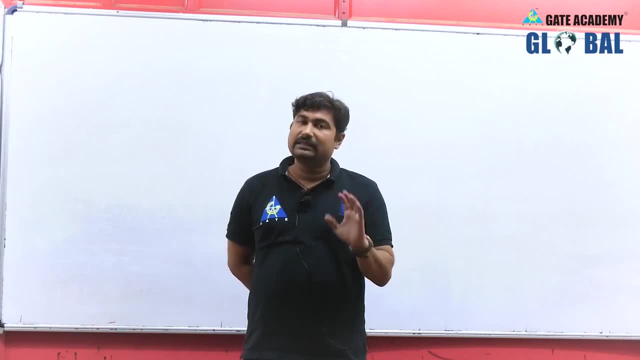 throughout. that is entire subject knowledge in this video, So it will be very helpful to you. You have to just follow the sequences as I have delivered and it will be very beneficial to you. If you found any difficulties with the lectures, you may post onto the comment box and I will try. 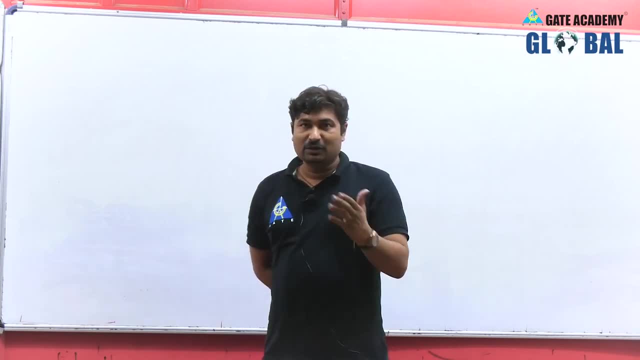 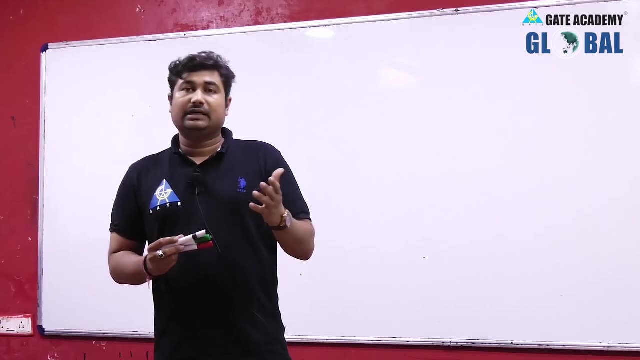 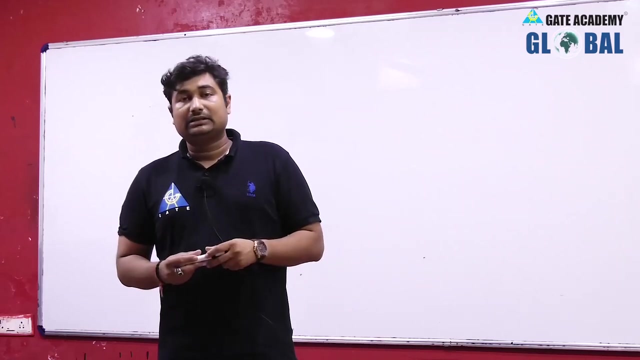 to improve on my later on lectures. So I am going to start with a transformer. First of all, I will take the concept of transformers. This is the most important concept for the electrical machines because most of the power, whatever we consume nowadays, are electrical powers and these all electrical powers are generated far away from our consumption. 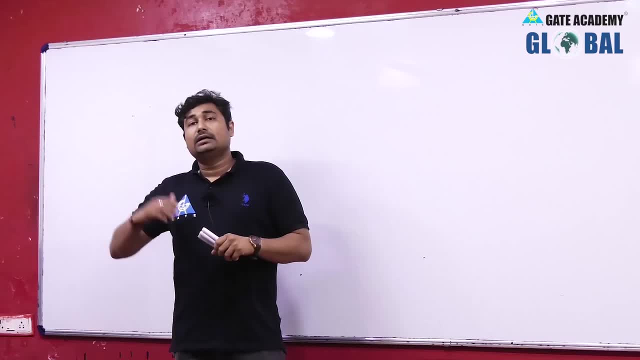 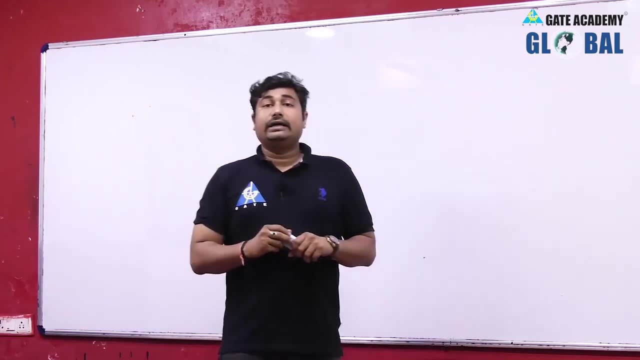 end. So let us suppose for a moment that the generation is done somewhere in Madhya Pradesh and then it is going to deliver in Bhopal. the distance is almost, say, 200 or 250 kilometers. then we have to choose the things. 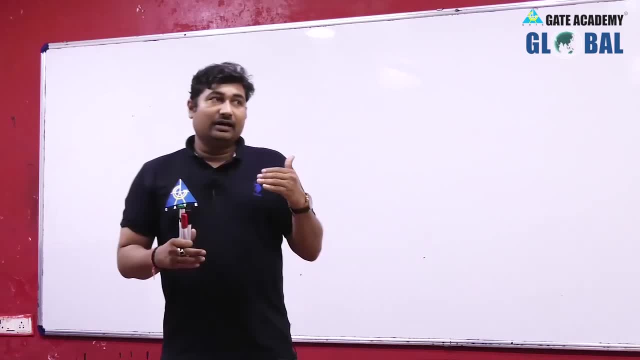 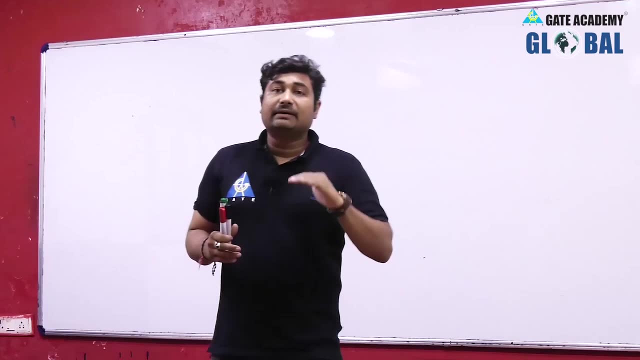 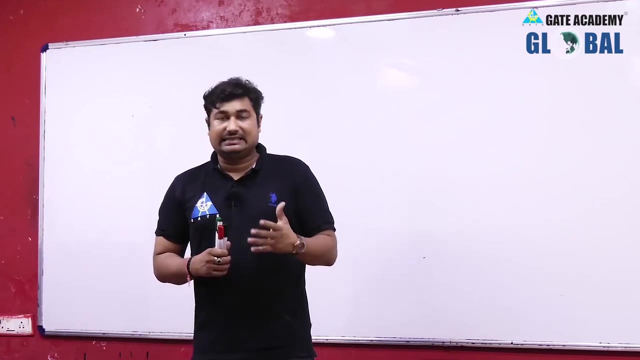 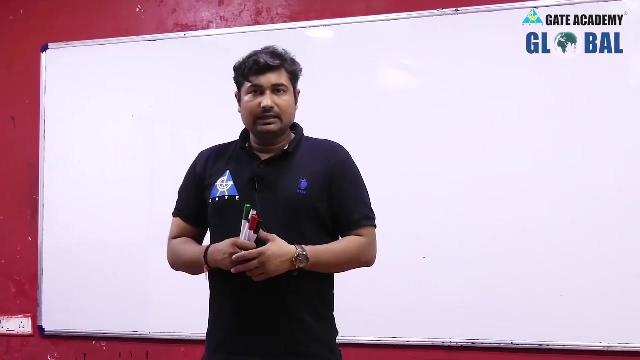 That is called as transformer, For without losing the power, we can effectively deliver the power to the user. So in my language I can say: transformer is just a device. Transformer is a device. you can note down this. Transformer is a device that transfers electrical energy. 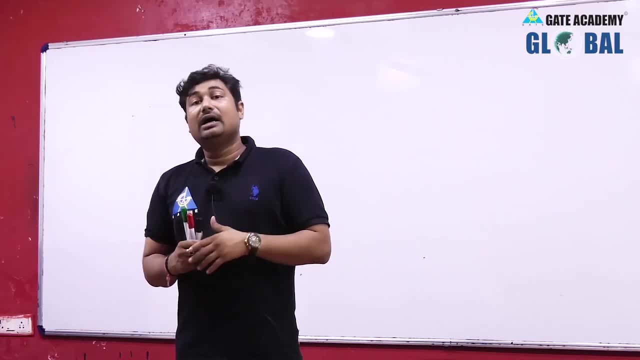 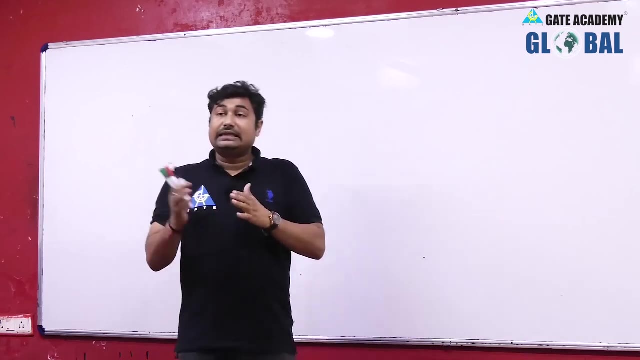 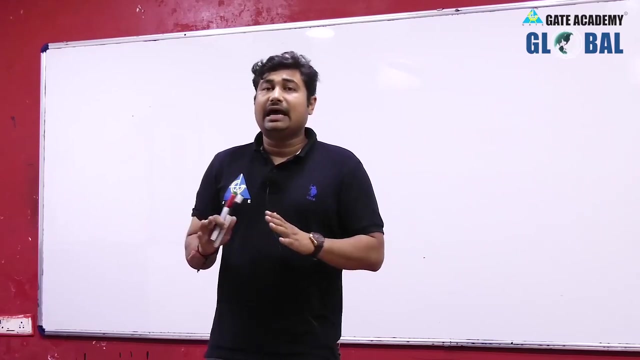 from one electrical circuit to another electrical circuit through magnetic fields, without change in frequency. So first of all the thing comes in. the mind is key. what, sir, why we are saying just a device, why we are not saying it as a machine? Because machine is something which contains some rotating part and transformer will have 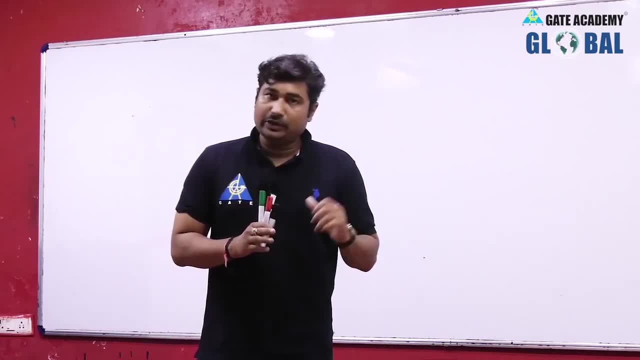 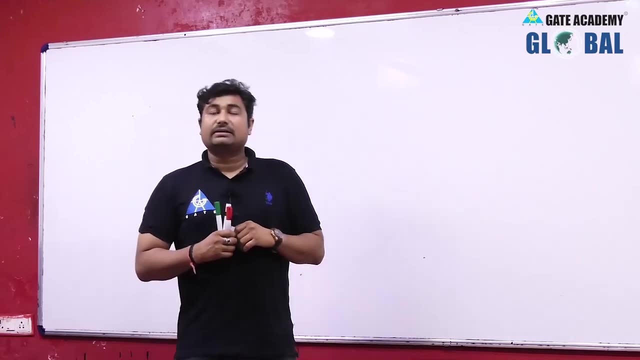 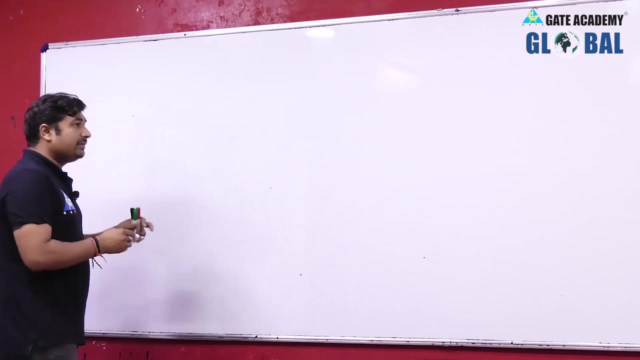 no rotating part. So we just say it is as a device. If I ask you what is the use of transformer So one can say to step up the voltage level or step down the voltage level, why we are using this step up or step down voltage level. please try to understand. So again I am repeating the 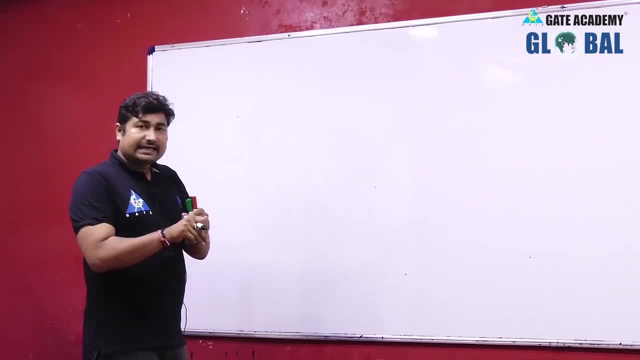 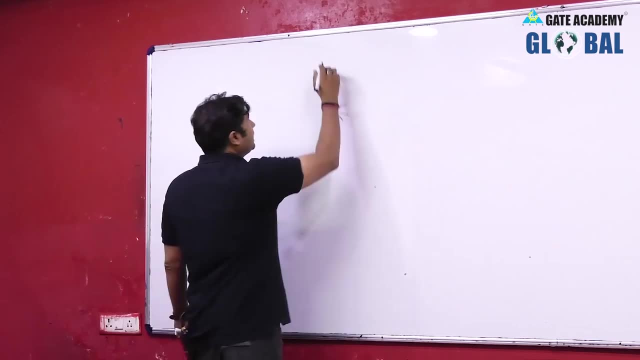 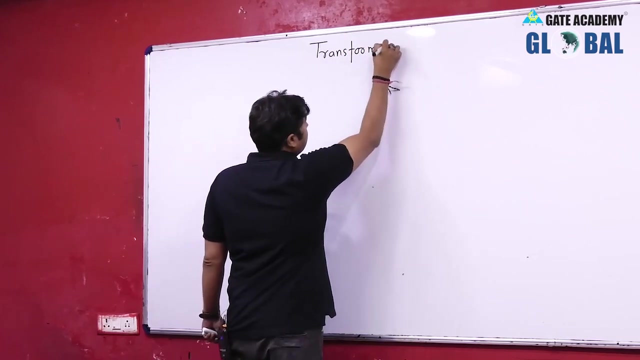 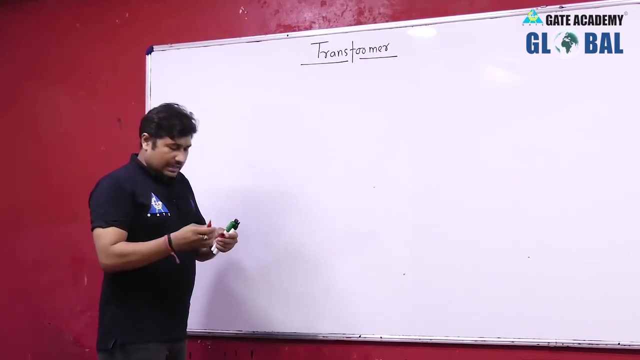 definition of the transformer. Transformer is a static device that transfers electrical energy from one electrical circuit to another electrical circuit through magnetic field. ok, So why we need a transformer? one can say, sir, to step up or step down the voltage or current levels. So let us suppose we have some. we have a generating station. 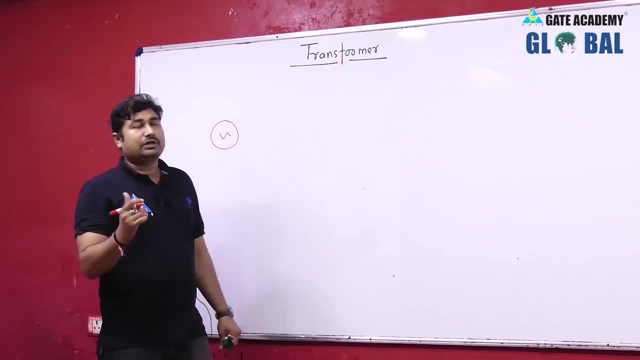 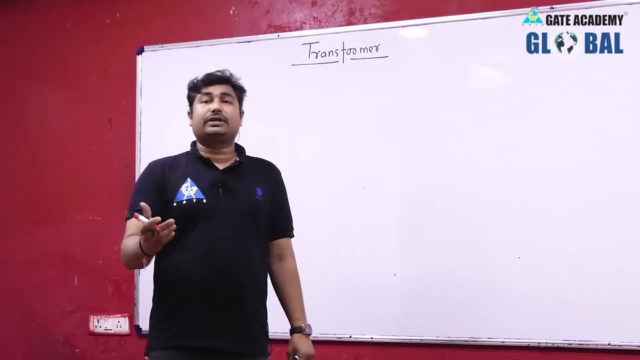 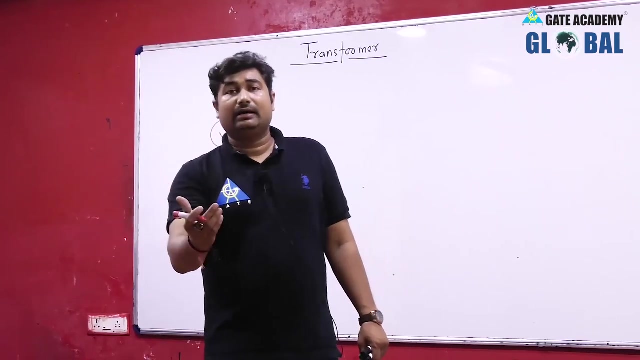 definitely all the generating stations. I am talking for a base generating station, not for your diesel engine. ok, So for a base plants. base plants are thermal, or you can say nuclear, or you can say hydro. If we talk about the maximum power comes from the base and base power plant. So 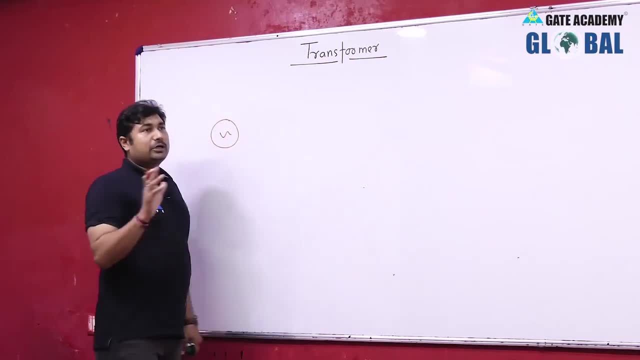 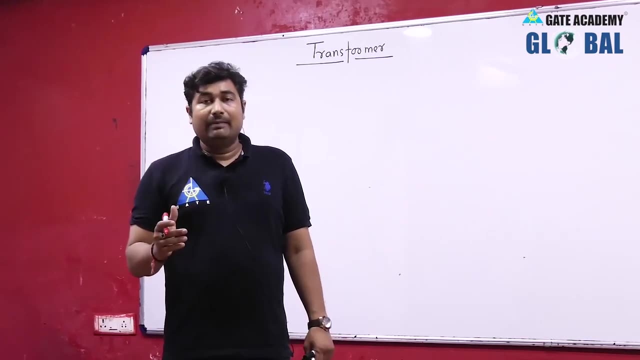 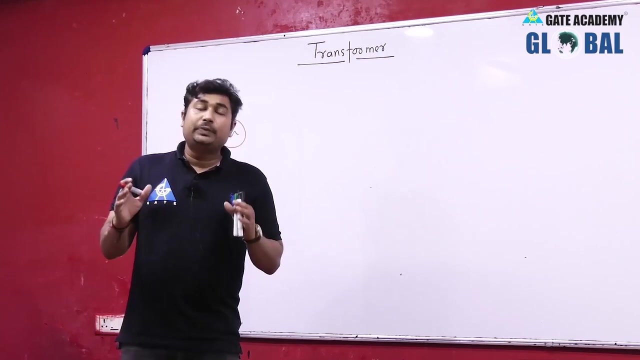 base power plant. let us suppose a hydro power plant. For hydro power plant, what we need? We need water and we have to give the potential energy to that water by providing some dam arrangement. So for dam arrangement we have to, we are bounded to be in that area, to develop the dam in that area where natural boundaries are present. So 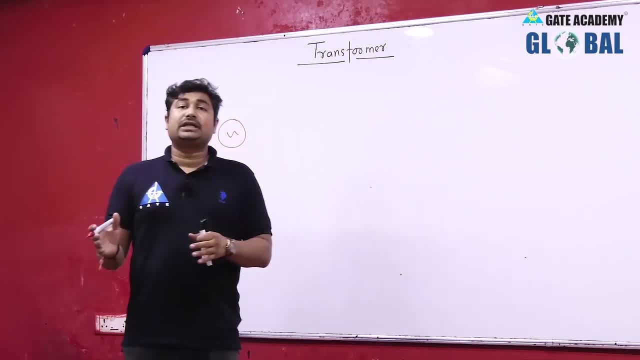 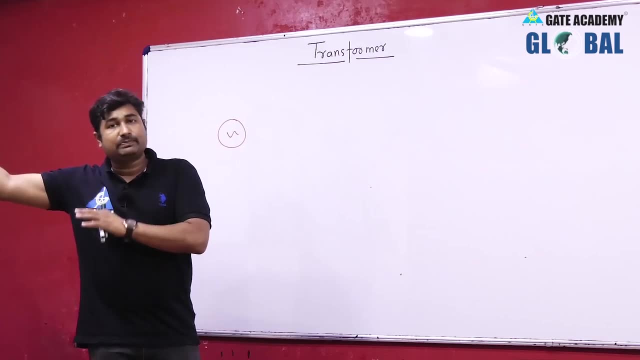 you can say that must be a heli areas and most of the population lives in the plain area. So we have to take that power from heli areas, that is, from the base power plant, hydro power plant, to the load end, consumer end. Let us suppose we have. 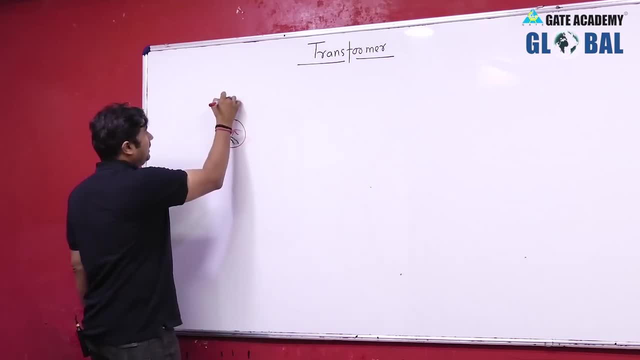 a generator and that generator is of 11 kV. ok, and let us suppose this generator is generating 1 KV, 500 mega Watt. Let us suppose this generator is of 11 KV and 500.. So you can say, sir, line to line voltage generated by the generator is 11 kV and the total three. 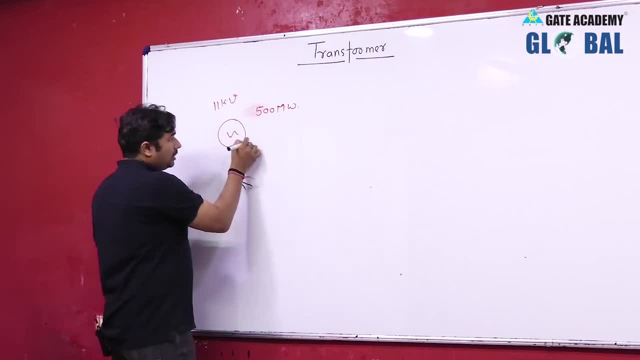 phase power is 500 megawatt, So you can represent this in terms of a three wires as a three phase line. Let us suppose we take one line. if we go with the one line, then total current in one line, that is per phase current in case of. in this case you can say, sir, 500 into 10 to. 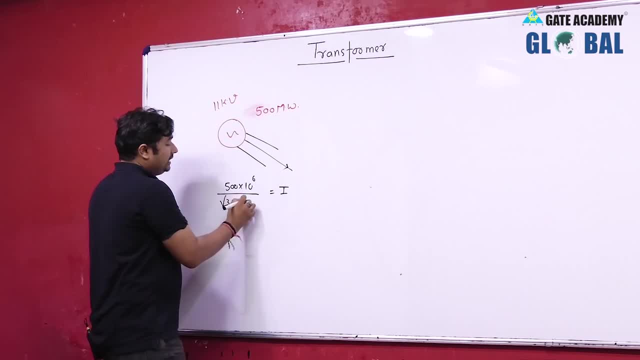 the power of 6 divided by root 3 into 11, into 10, to the power of 3.. So you can say, sir, this current is in kilo amperes. So this kilo ampere currents are going to flow from one hydro station to some load station. 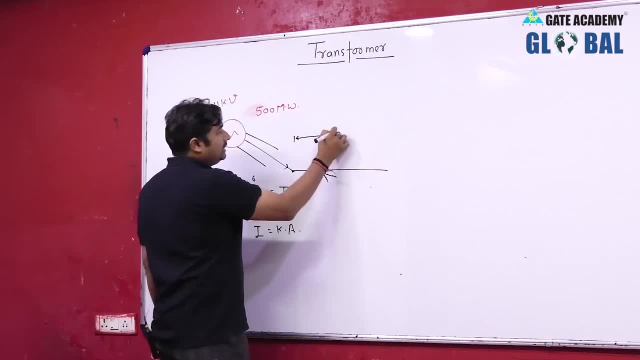 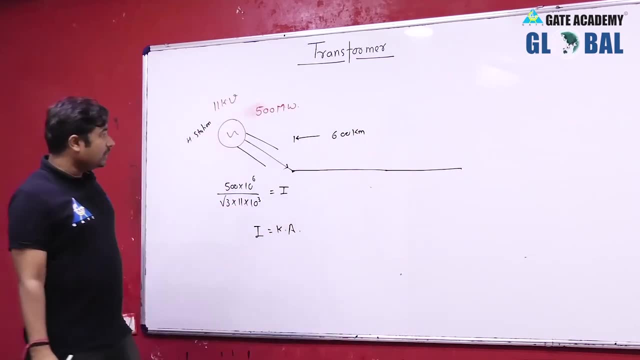 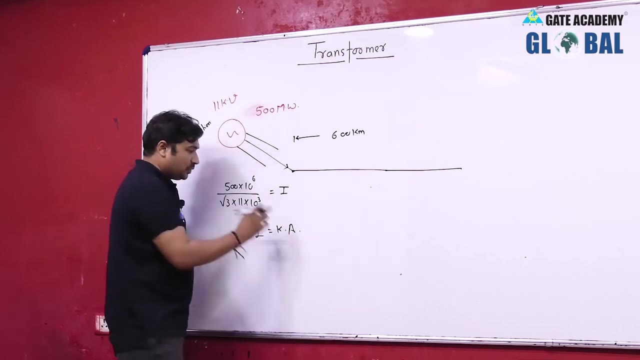 and you can say that if the distance between them is nearly, you can say 600 kilometers. So if we have to transmit the power to 600 kilometers, Then what we need? We need this wire thickness of this kilo amperes. why every wire whenever you are going to purchase. 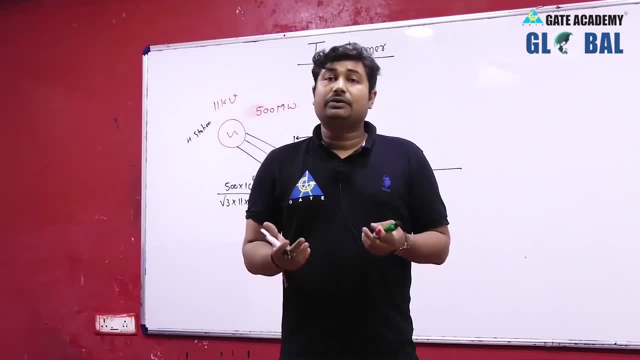 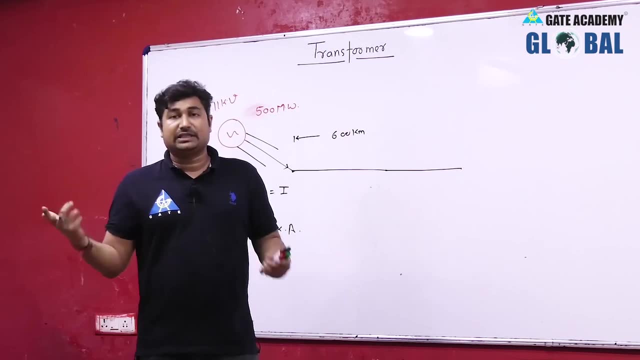 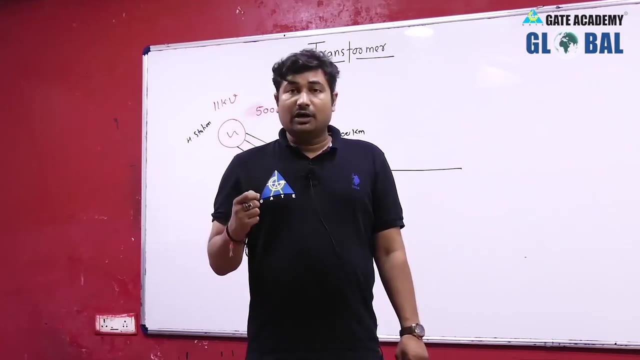 some wire. that wire must be in terms of a current rating or you can say thickness of wire. Whenever you buy a wire you can ask that give me 5 mm thickness wire. or you can say 5 ampere wire. So why we are defining the wire in terms of amperes? this is because we all know that. 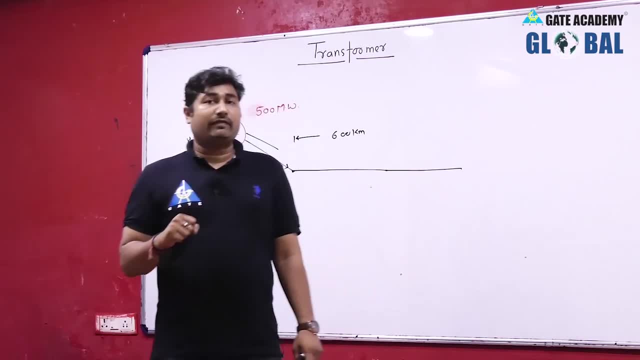 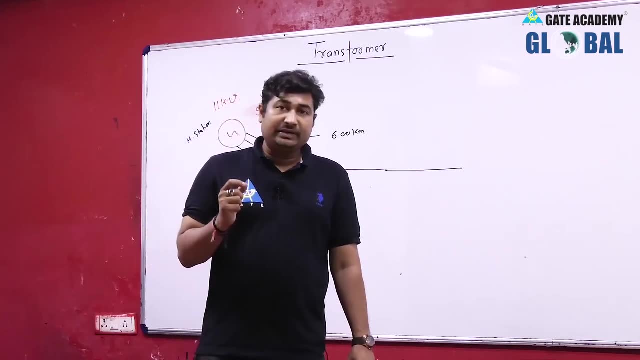 the resistance of a wire. The resistance of a wire depends upon the area of cross section of a wire and that is R is equals to L by A. So if we reduce the area of cross section it means if I am going to use a thin wire then definitely its current carrying capacity is lower as the resistance. 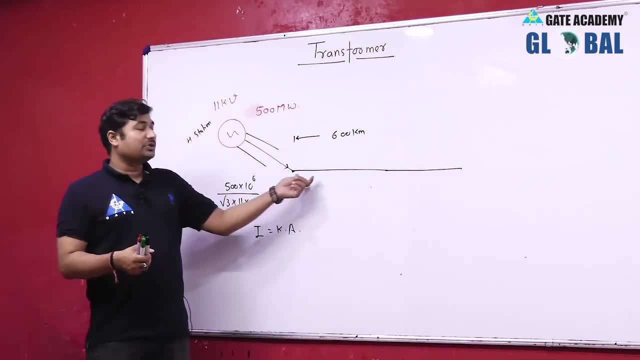 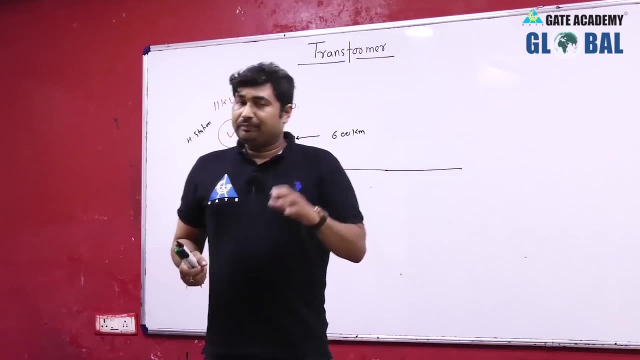 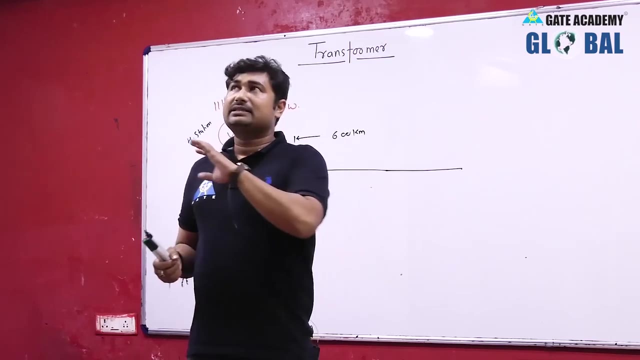 is high, Since this current is independent upon the resistance. so you can say: if that current flows through the wire, it will produces I square R loss. Let us take an example. I am using a fan. ok, So the fan is supplied, the fan is connected by a thin wire, that is, of 5 ampere wire. 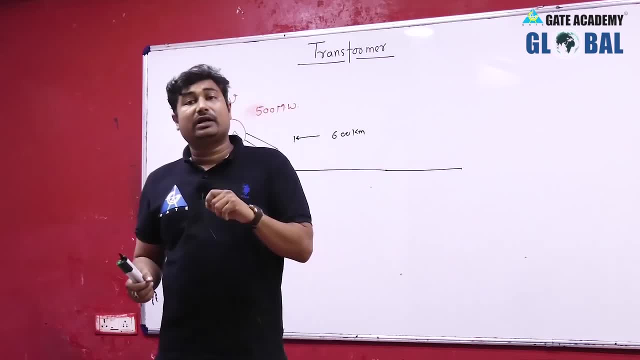 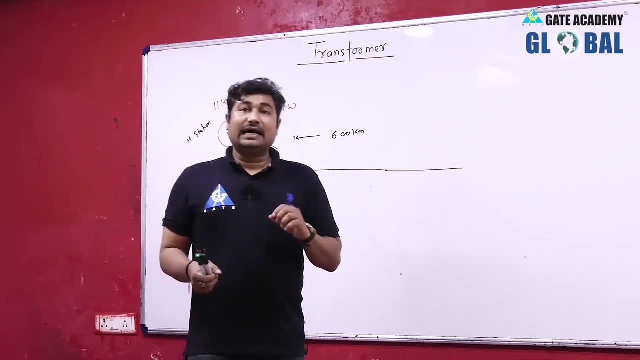 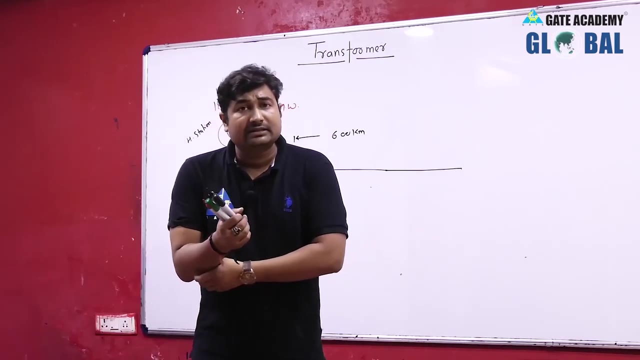 However, if the same wire is used for supplying power to AC, that is, air conditioner, then what happens? you can say, sir, that wire will be melt out. Why that wire is melting out? Because, sir, the current flowing in the wire is independent of the wire resistance and 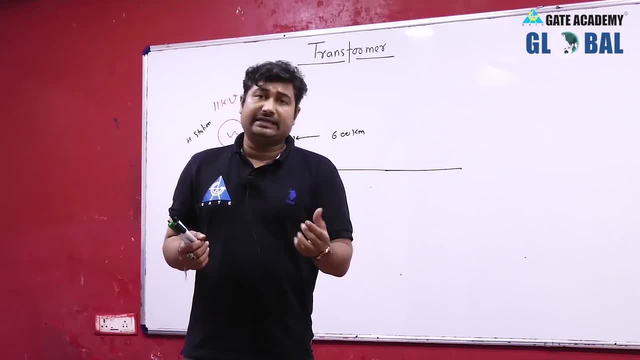 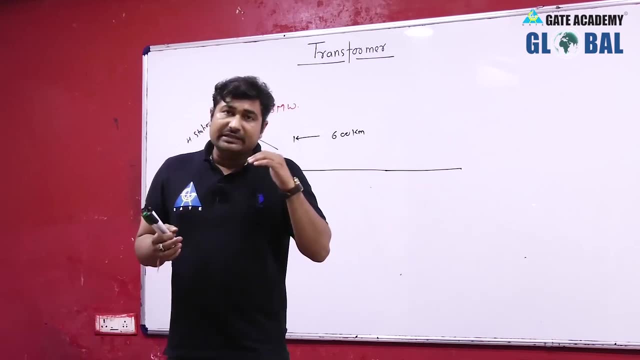 since the current is very high, So I square R loss is very high, since the wire is thin, So the electron collision is more and you can say temperature increases. ok, So this temperature increases is a cumulative process. as temperature increases, you can say: 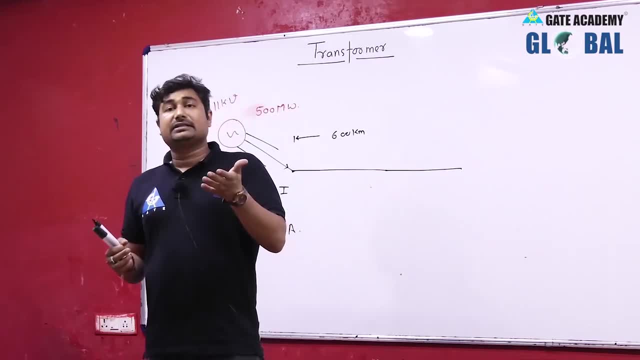 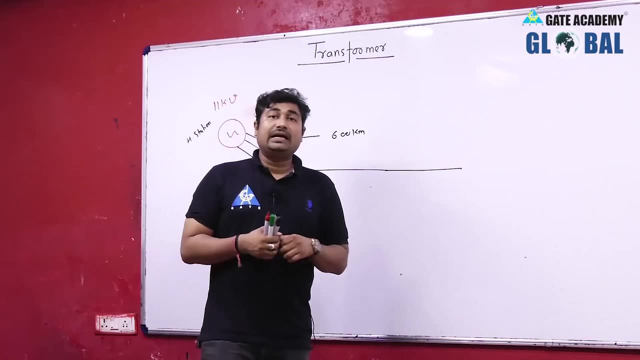 resistivity of the conductor increases and again temperature increases. This temperature increases till the wire melting point reaches and you can say, sir, finally the wire will get melt out. ok, So whenever we take a wire and we say that 5 ampere wire or a 10 ampere wire, 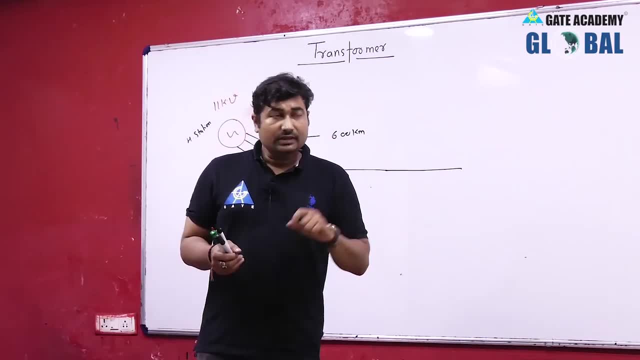 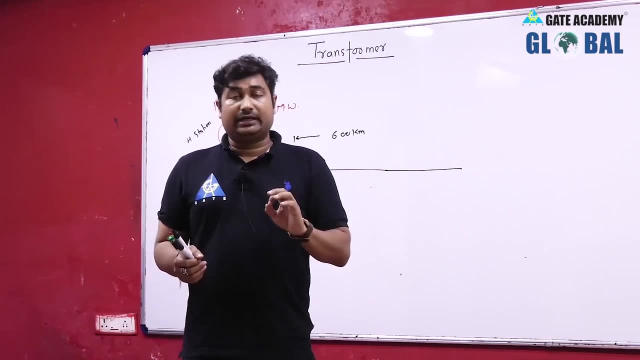 Whatever, you can say very simple: Yes, ampere wire. it means what It means. from 5 ampere wire you can flow 5 ampere current throughout the day, throughout a year. it will not affect the performance of the wire. 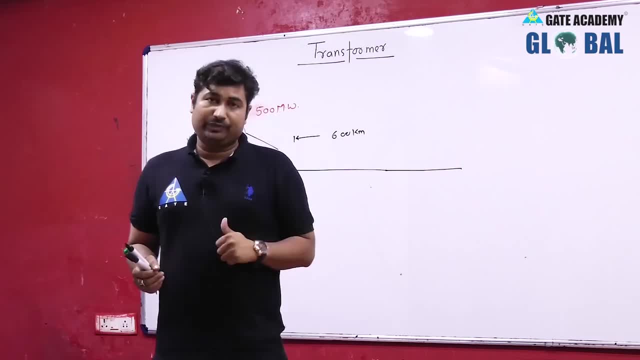 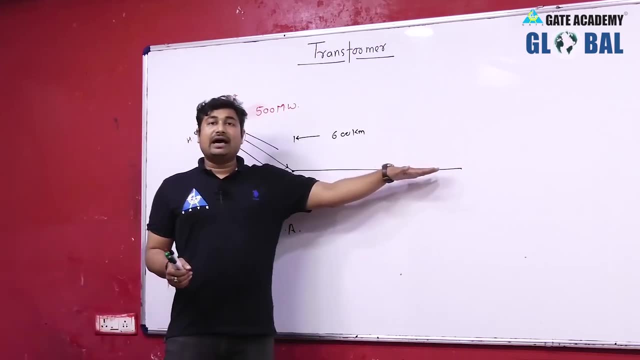 it will not produces the heat that much which melts the wire. So if I am saying I have to flow the kilo amperes current from this wire, it means the wire needed will be very thick. you can say it will be thicker than you, sir. yes, it will. 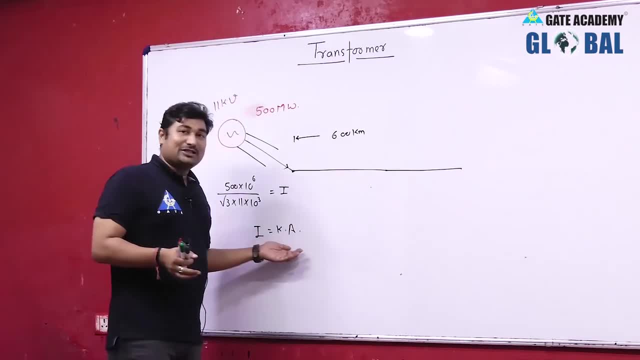 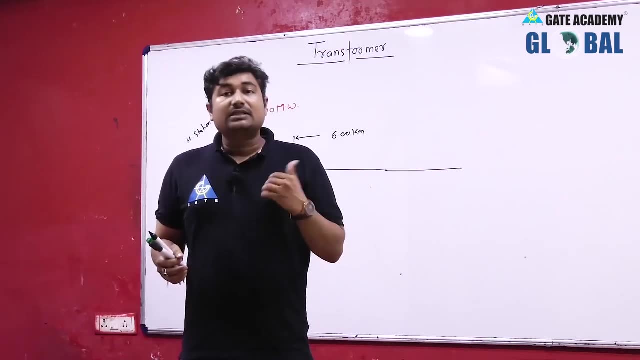 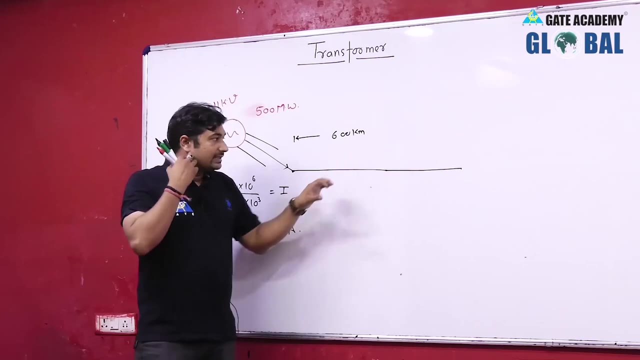 be thicker than me. also, if the wire carries kilo amperes of current, then it will be needed thicker than me. And you can say, sir, how we can handle such a thick wire. Such a thick wire means very high amount of material is needed to transfer this power. You can say: 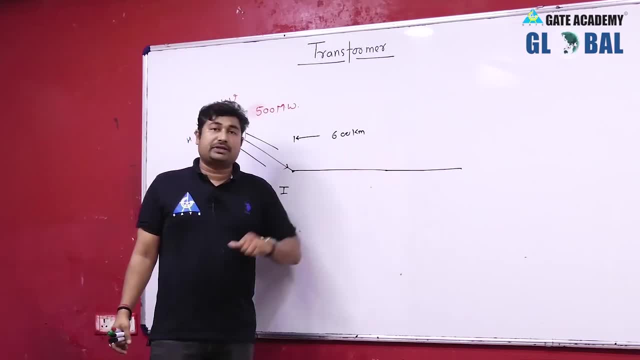 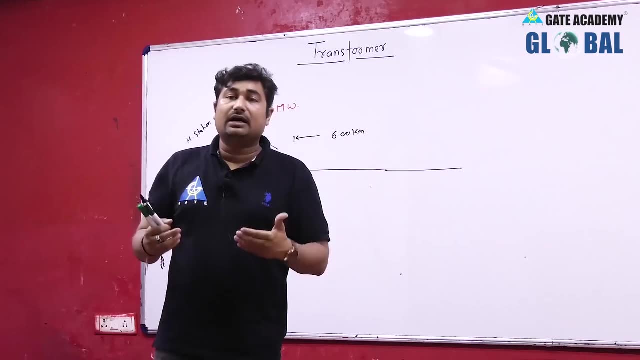 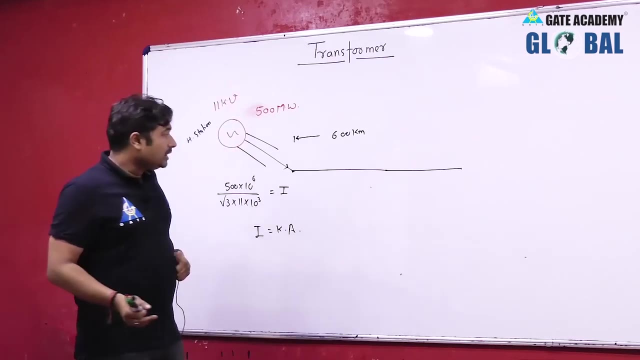 sir, it is also very difficult for overhead transmission because we cannot hang the very heavy weight wire, The wire to such a height which is needed for a ground as a which is needed for a potential difference from ground to wire. ok, So the safe height from the ground, So you can say: 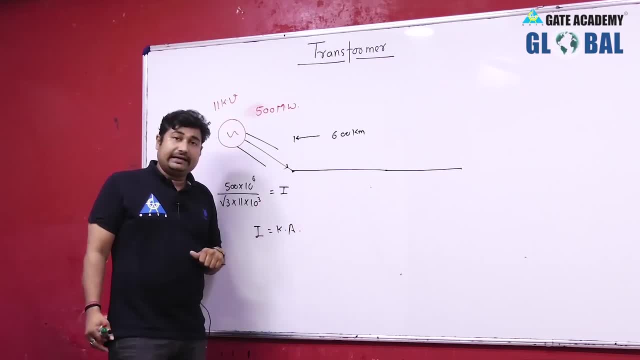 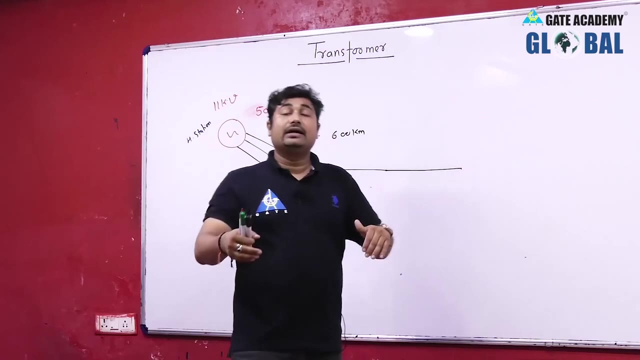 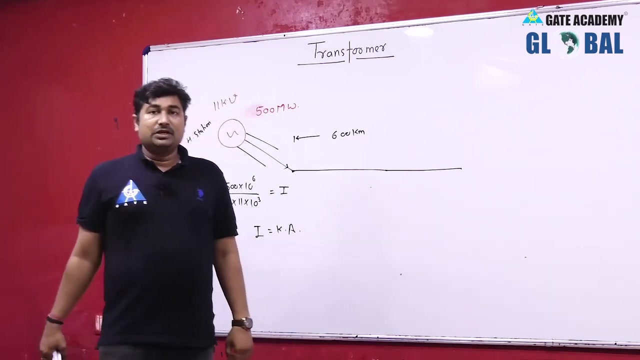 sir, the wire thickness is very high needed, So the material cost increases very high. the material cost increases that high that you can transmit the power from this end to the load end will take that much of cost, which is cheaper than installation And installing a diesel engine within, outside or outside of our home. ok, So in order to 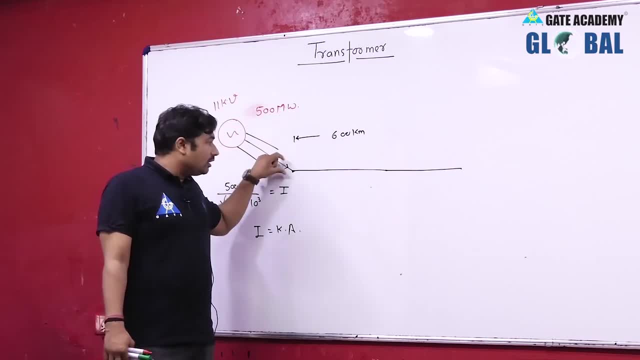 reduce the thickness of wire in order to reduce the loss that occurs in terms of I square R. while the power is spread from source to load, we are using the transformers, And the transformers are ones which make us able to deliver power from long distance. ok, And 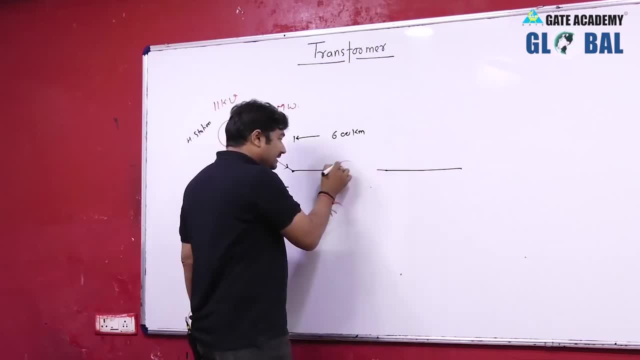 handle power from long distance. So the power is from the source to load. we are using the from long distance transmission line. You can say, sir, if I use one transformer here, let us suppose this transformer increases the per phase voltage. I am just representing. 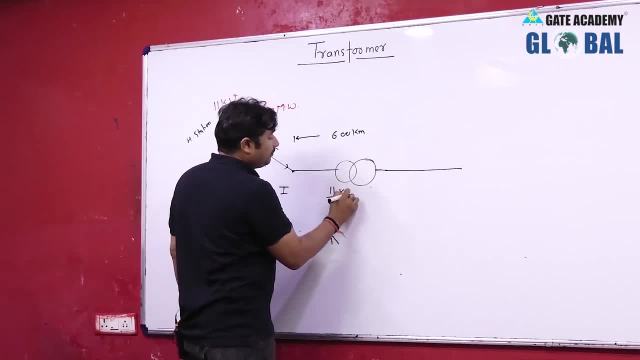 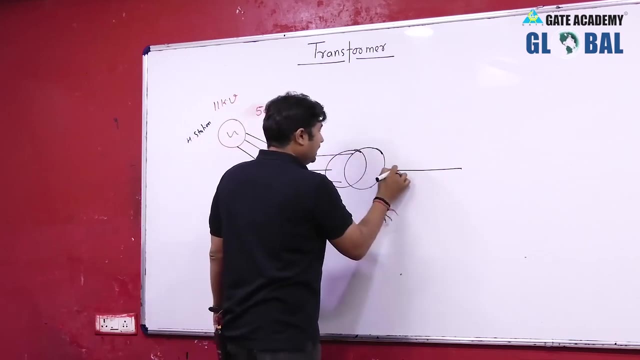 Let us suppose this is the per phase voltage is 11 kV by root 3 into. you can say, sir, it increases the voltage level to, or I am using all the three phase wires. it is better to understand in this way. So you can say, sir, we have this three phase transformer and this: 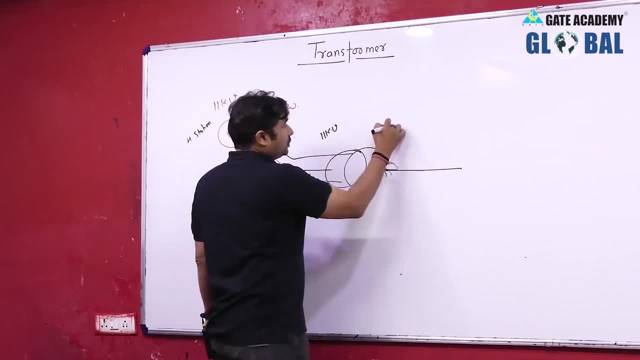 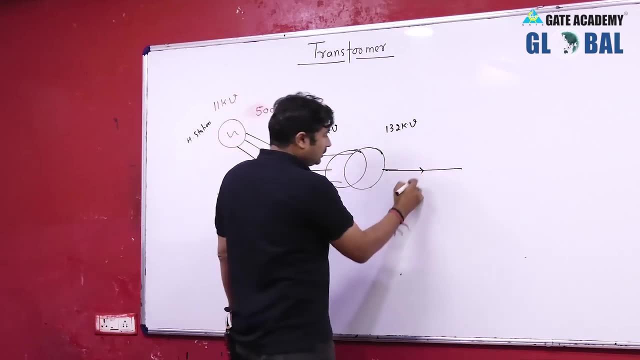 three phase transformer converts 11 kV to 132 kV. So if we increase the voltage level, then what happens to the current? You can say, sir, now the current here will become, the power will remain same. Now the current will become. 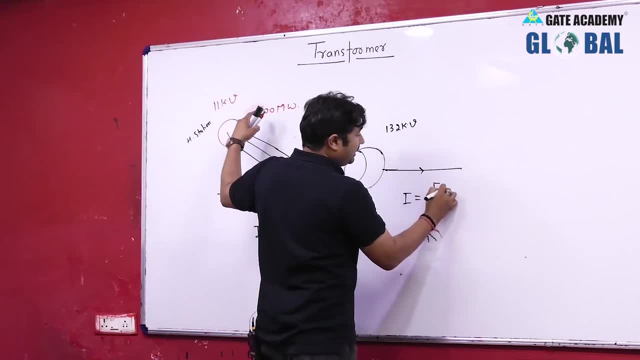 you can say, sir, power will become 500 megawatt, that is, 10 to the power of 6 upon 132 into root 3, root 3 into 132 into 10 key power 3.. So you can say, sir, now the current will. 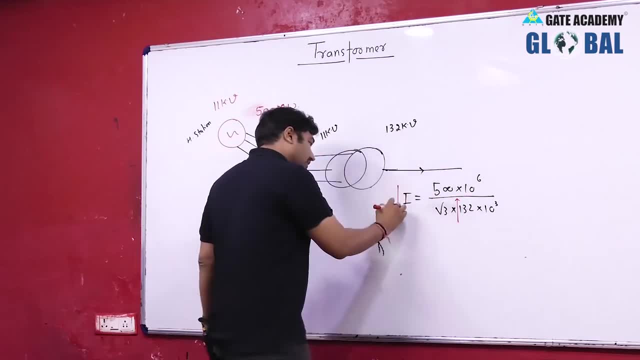 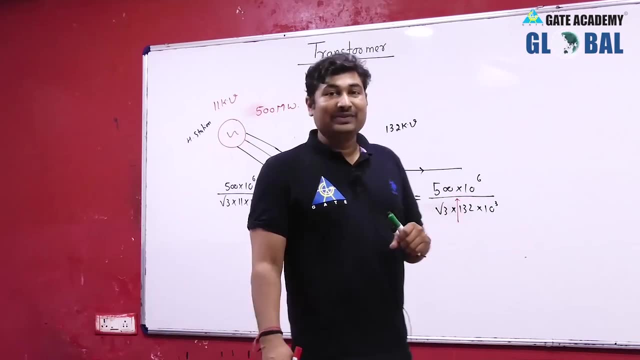 is decreasing as we are increasing the voltage, so the current is decreasing and now the thickness of wire needed will be lower so the thinner wire can perform if we further increase from 132 kV to 444 kV, you can say, sir, 440 kV, so you can say: 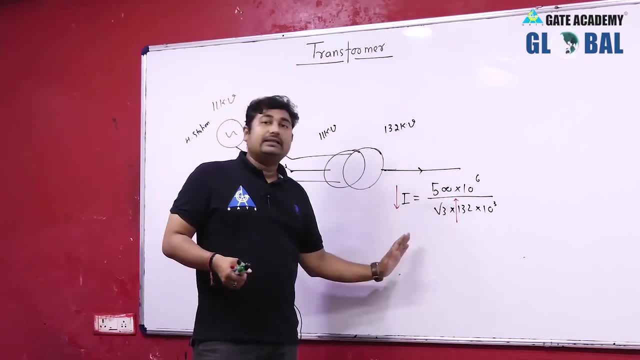 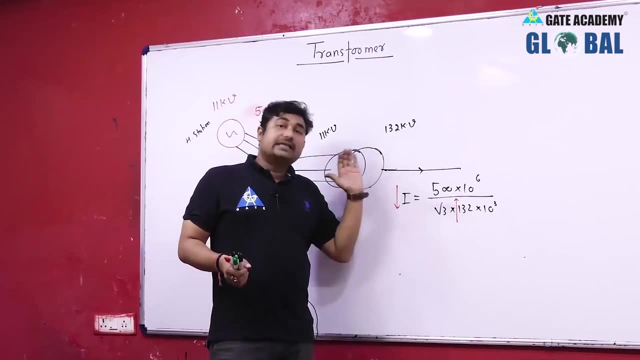 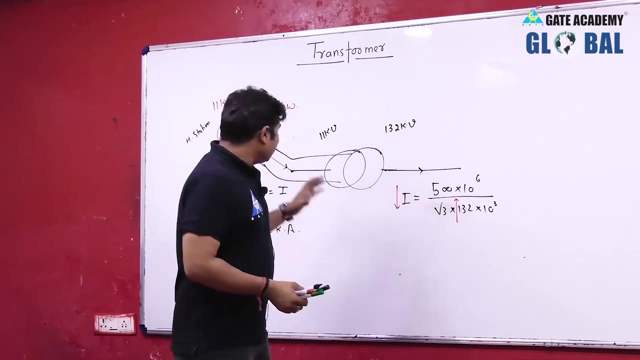 sir, as we are increasing the voltage level, the current level in the other side will going lowering down, and the decrease in current make us able to use a thin wire for a very long transmission. is it okay? so, sir, this is okay, sir. we can generate the power now and we can transmit the power to a very 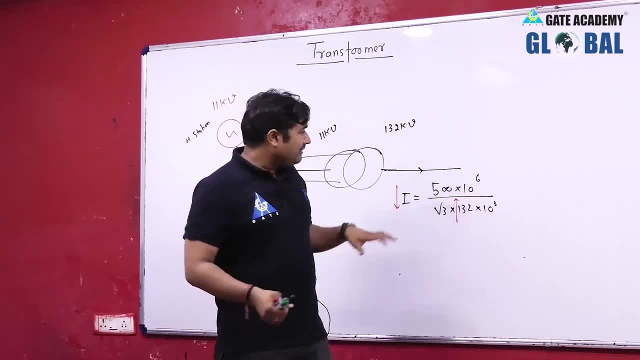 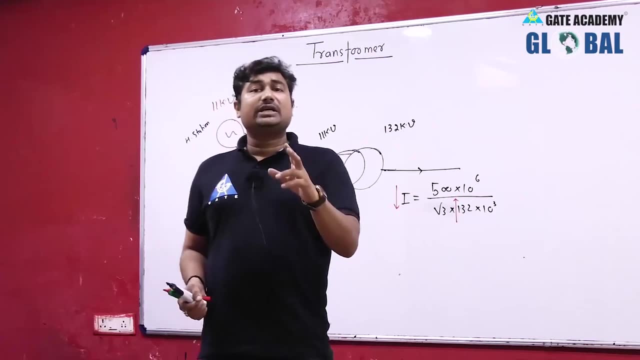 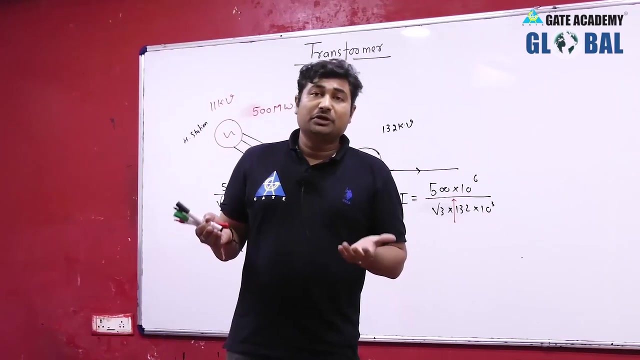 high voltage. okay, sir, why we are not consuming the same voltage level at our home? the second question arises, and that is because of the insulation. what is insulation, sir? if the potential is very high, then we must have to provide the suitable insulation from ground, or you can say from metallic parts of the 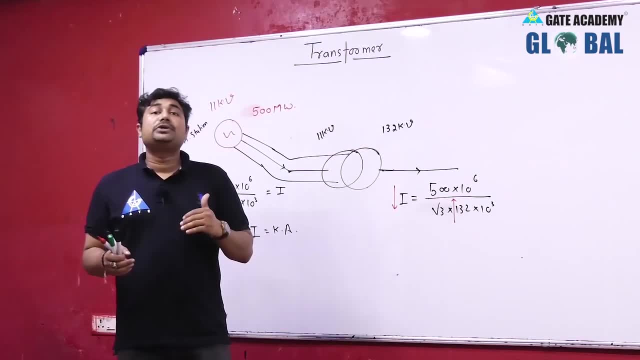 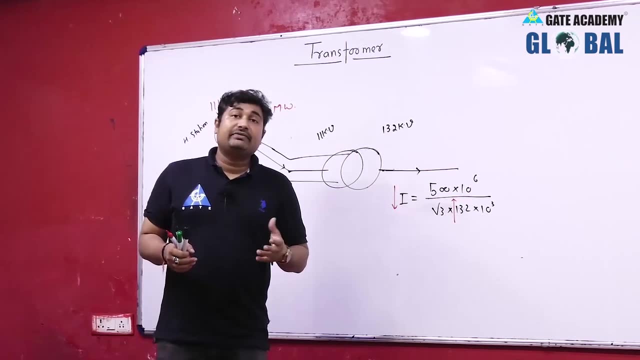 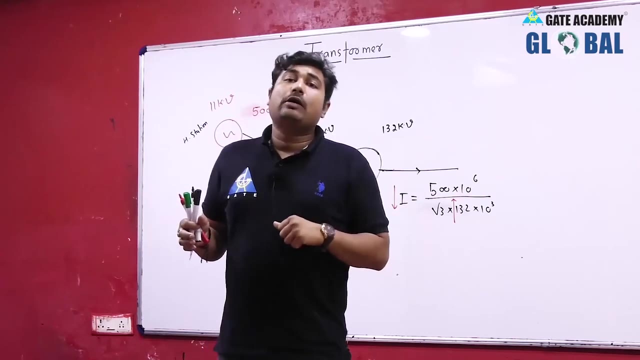 machine to ground and for that we need to use more and more thicker insulation. for 132 kV insulation level we need very thick insulations and that thick insulations again causes the insulation- you can say dielectric loss, and also, sir, the thick insulation will create a very the machines. 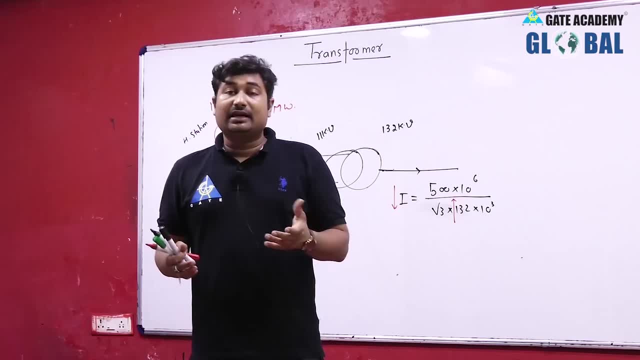 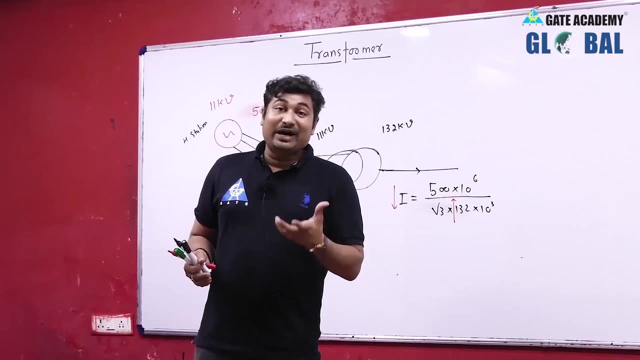 size to be very large. so very large it means, let us suppose I am using a fan and that fan is of 132 kV. so think about the insulation provided in the fan windings needed to be 132 kV, and for that the size of the fan is very big. so 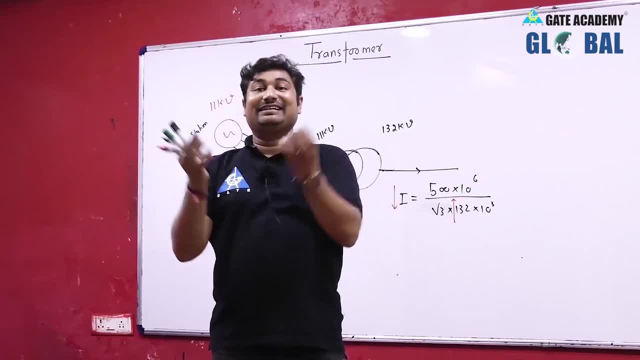 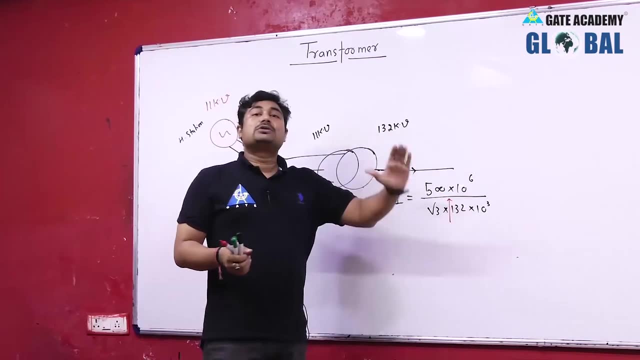 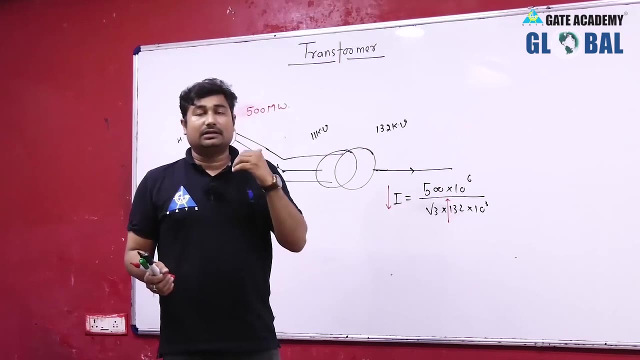 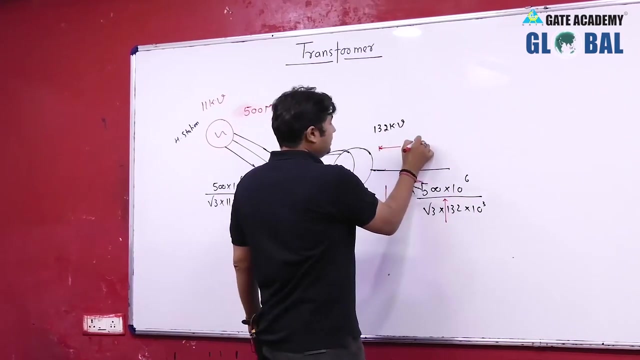 it may be bigger than our house. so how we can commission on a very small space? okay, so that is not possible. so again, we need to step down so that we can easily manage the our domestic or industrial machines at proper insulation level. ok, So we again use transformers. now you can easily transmit this to 600. 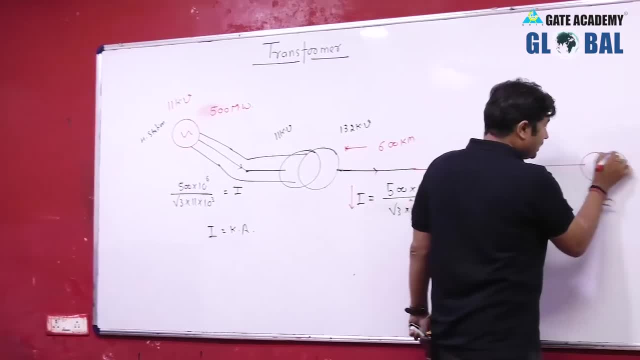 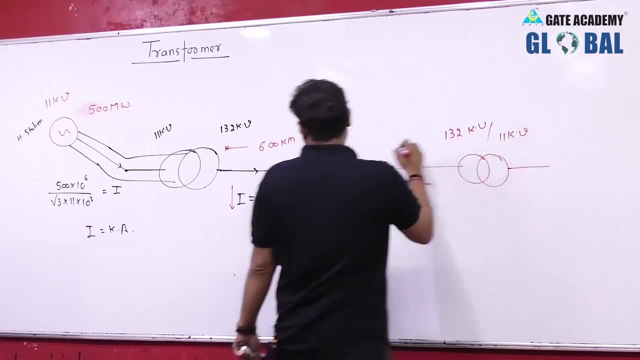 kilometers. you can say, and we can use some other transformer again to step down the voltage again from 132 kV to 11 kV. again the voltage is a step down. So by step down in this voltage again the current on that side is again increases. 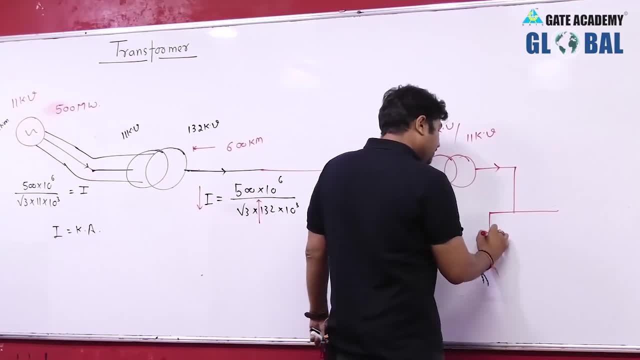 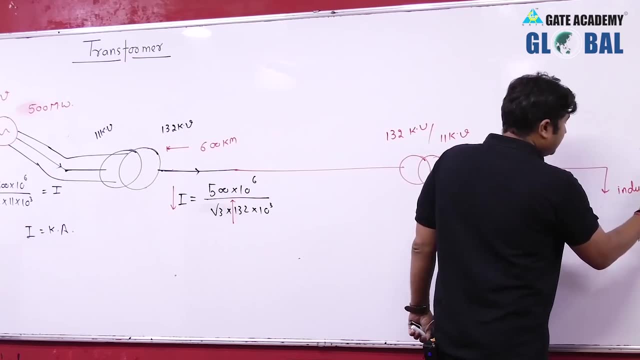 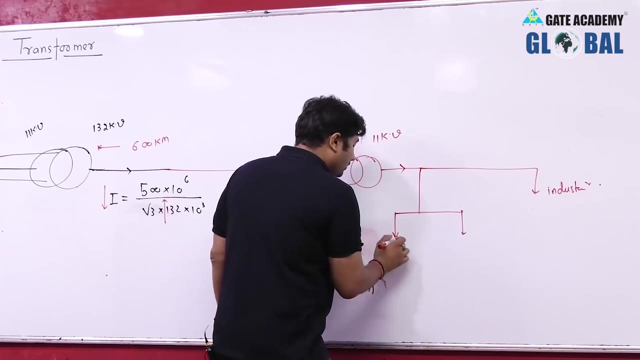 You can further reduce. you can further reduce this. you can say, sir, I have to use the multiple users. some are the industrial users. they may take the power at this particular voltage level, that is, 11 kV. some of them may be using 6.6 kV, So you can use another transformer at the. 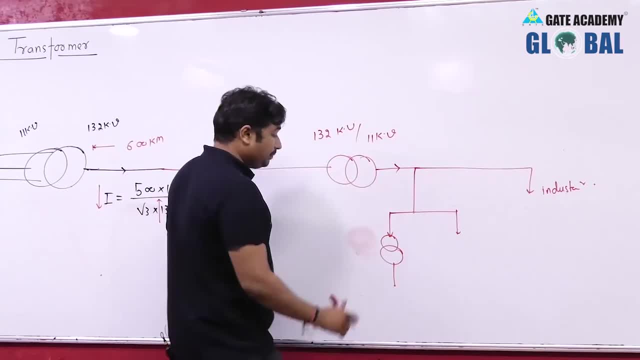 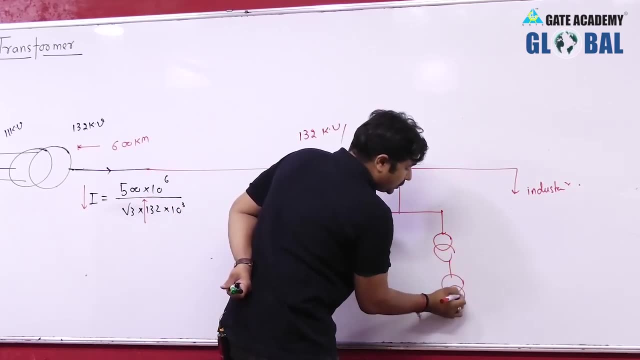 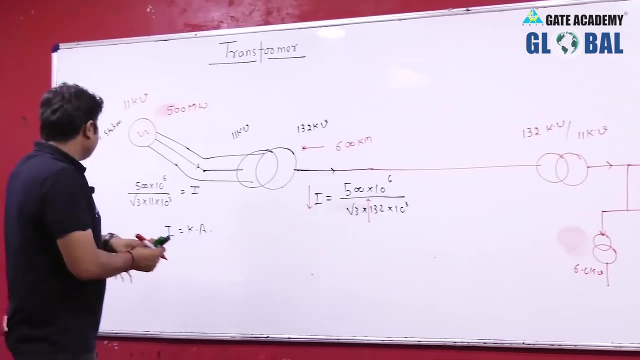 substations to again further lowering down this and this will become 6.6 kV. now You can say, sir, for domestic user we can further step down to 440 volts. that is line to line, is it ok? So this possibility that power is generated far away from the consumption? 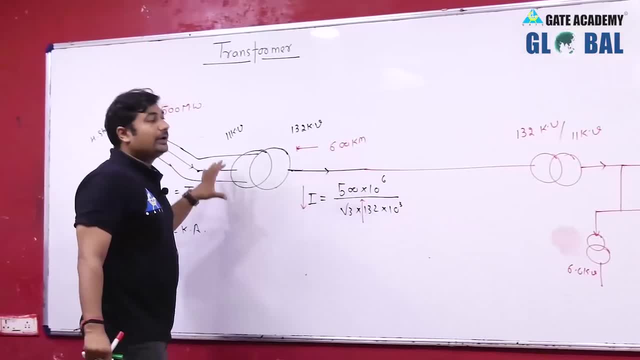 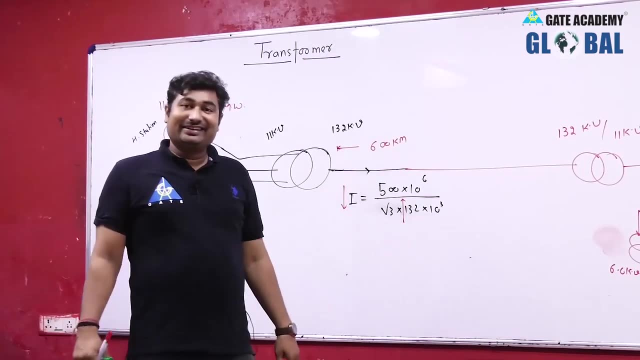 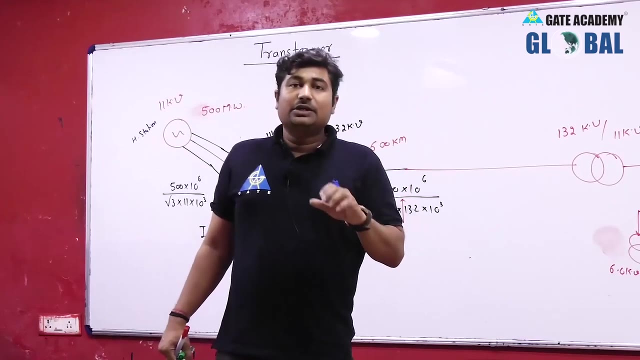 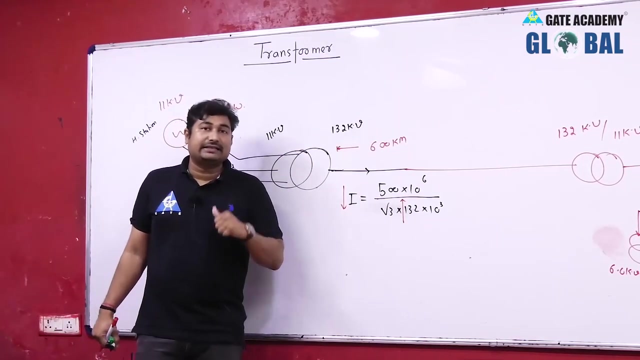 end is only possible because of the transformers. without transformer, we cannot even think about the electricity. Why we can? we can create electricity. yes, of course, we can easily transmit the electricity to from our diesel engine to our house, But that is not the proper way to get the cheaper electricity. In order to get the cheaper electricity, we must have. 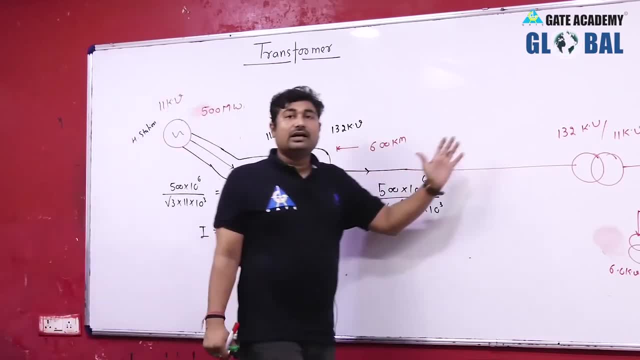 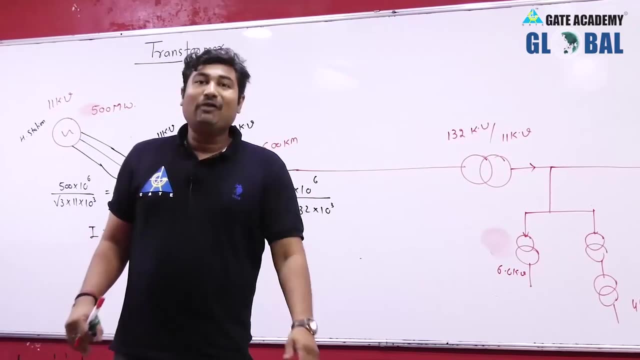 to go with the base plants, and the base plants are far away from the load ends. We cannot make a hydroelectric power station in Delhi. However, we can make it in somewhere in you can say, Tihari, that is Tihari bandh. We can easily create the power station in Delhi. 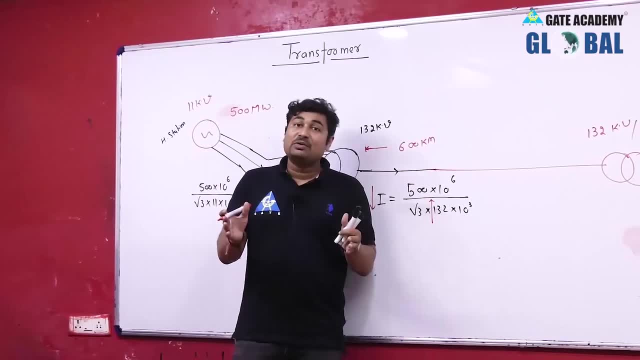 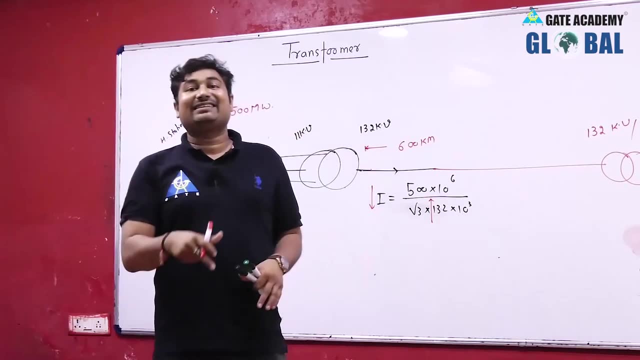 We can easily create the power station in Delhi. However, we can make it in somewhere at Delhi. We can easily create the bandh. you can say dam only on that area where the natural boundaries are a present. However, we are generating there and we are using at. 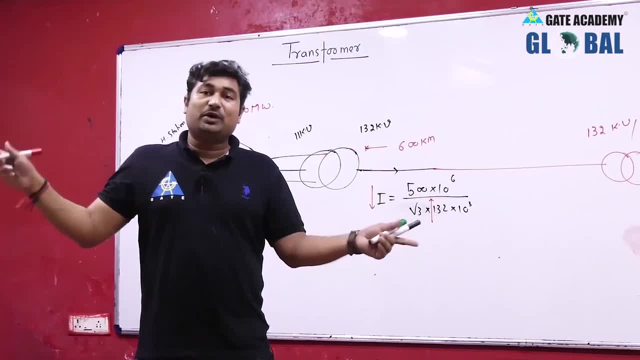 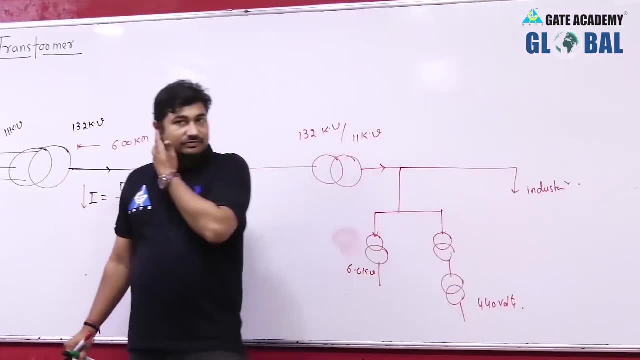 Delhi. and this consumption is only for this. transmission is only possible with the help of transformers. Without transformer, we cannot even think about the power transfer, Is it ok? So I am now. I can say: you well know about the insulation. The insulation depends upon. 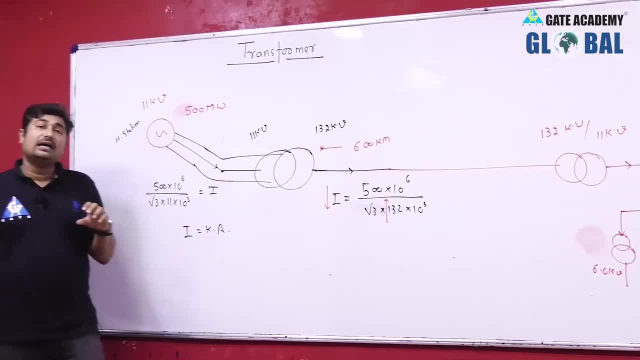 the exclusions for what is SARAH valley? Yeah, sorry, I donot have any counterfeiting option. This is 진수ляются. Maggie has a dliga near zumelle, Are they? gin clock will make bill paper Which you can place themselves. 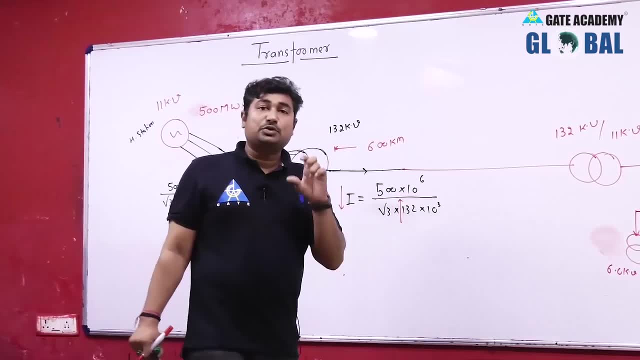 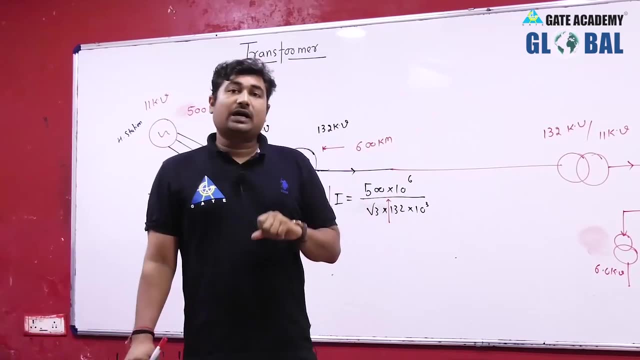 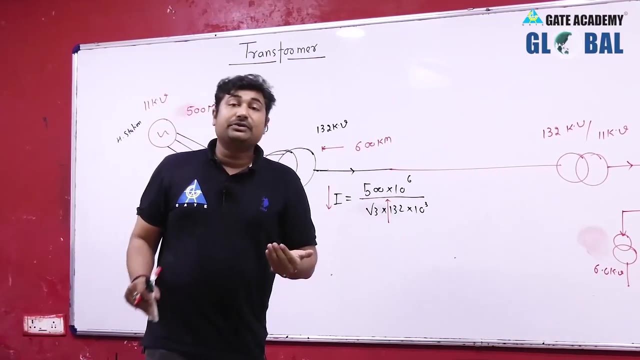 insulation voltage level depends upon the insulation level and you can say the wire thickness current depends upon the thickness of wire. So for higher current rating you need thicker wire and for lower current rating you need thinner wire. For high voltage rating machines you need thicker insulation and for low voltage machine we need thinner insulation. This is 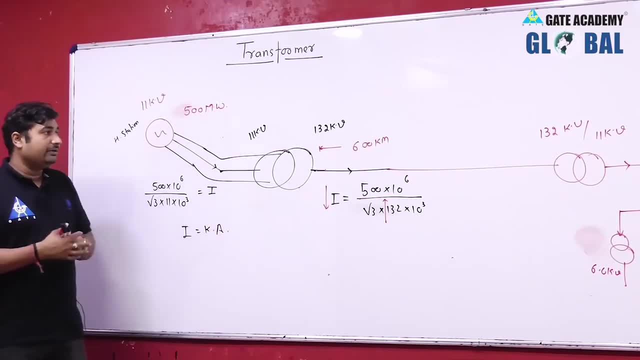 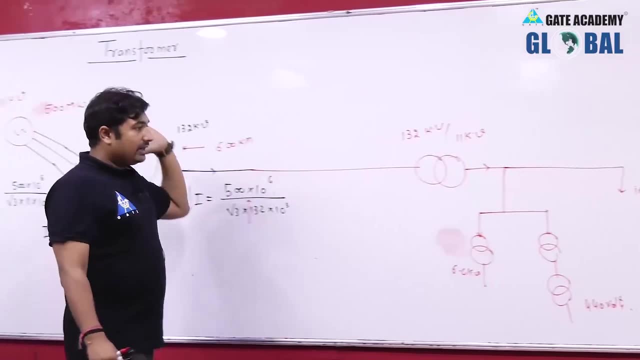 the some basic part of this transformer. I am hoping you will able to understand now why we are choosing the transformers for step up and step down in order to make the power transmission effective. Is it ok Now further observe? what are the uses? if I say 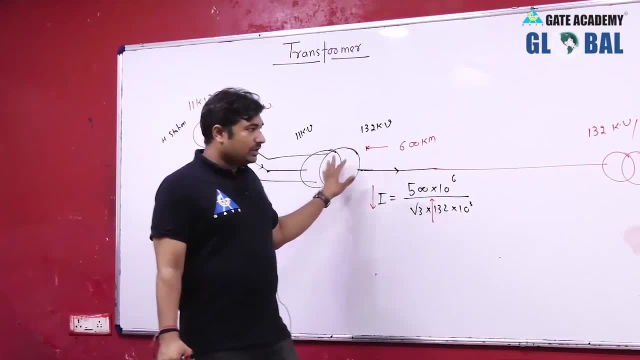 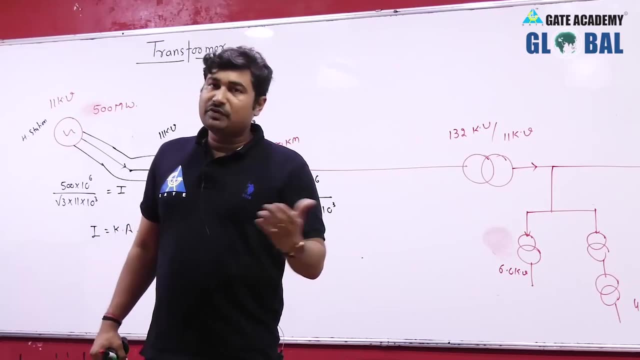 uses. though we have one use to step up or step down the voltage levels, What is another use of transformer? You can please note down uses of transformer. Transformers are used for step up or step down voltage levels. Transformers are used for step up or step down voltage levels. Transformers are used for step up or step down voltage levels. Transformers in control systems are used for impedance matching, so that maximum power transfers from source to load. Also, transformers- high frequency transformers- are used- you can say better to say pulse transformer- finds a wide application in 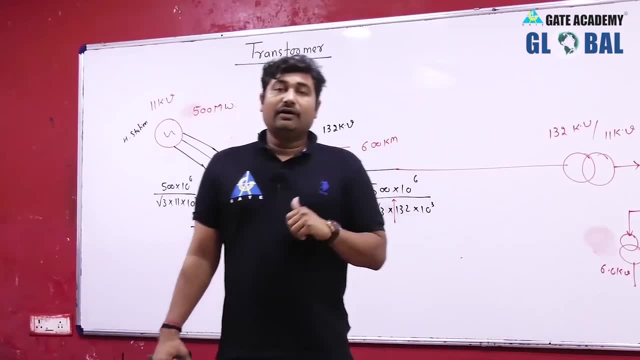 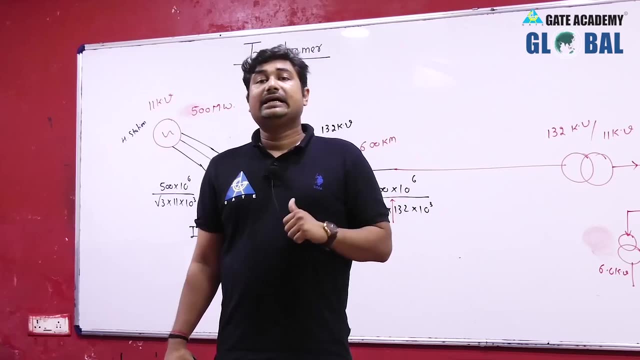 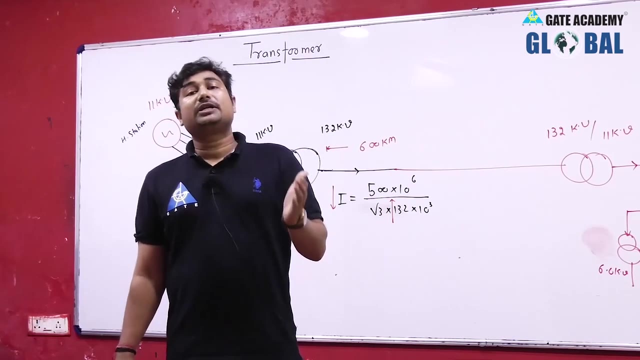 digital computers and radars. Further, you can say, sir, transformer is used to isolating DC, while it permits the flow of AC. Transformer can only pass AC. So transformers are used for isolating DC, while it permits the flow of AC. Before going to the transformer, we need to 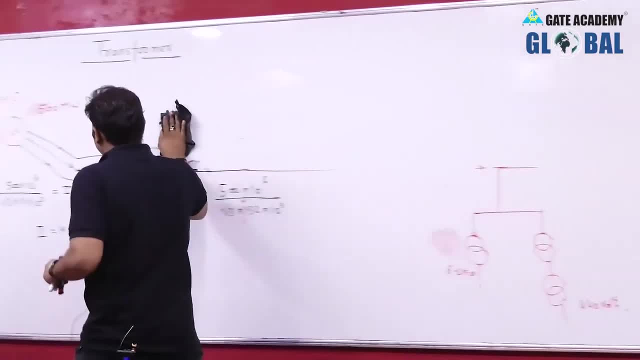 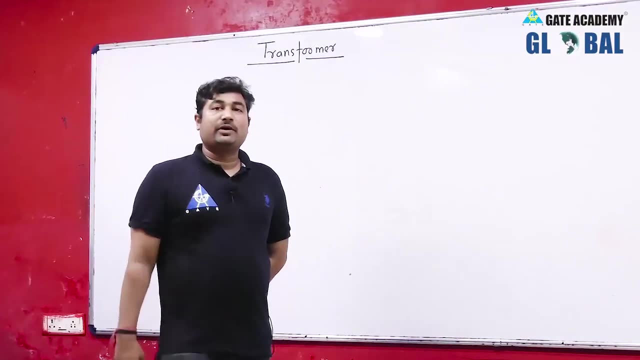 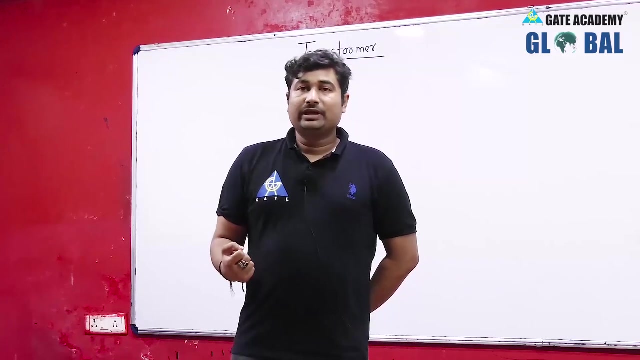 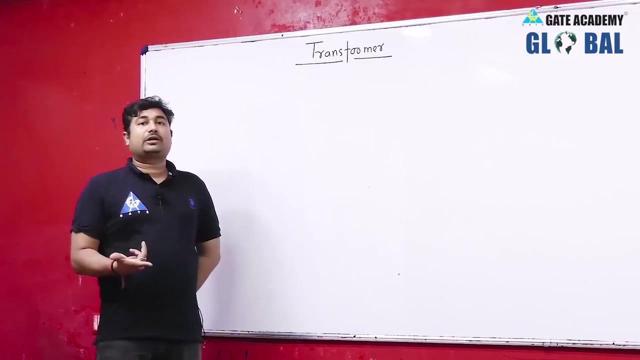 understand some basic concept of magnetic circuits. So for that I am representing some important conclusions. Before going to transformer we need to understand some basic laws like Faraday's law for electromagnetic induction, Lenz law and also right hand curled rule. So first of all, Faraday's law of electricity magnetic induction. this law makes 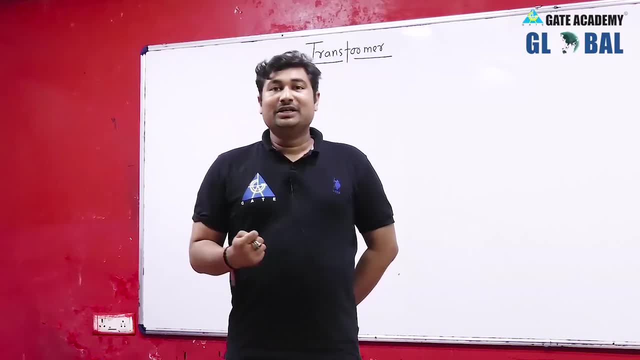 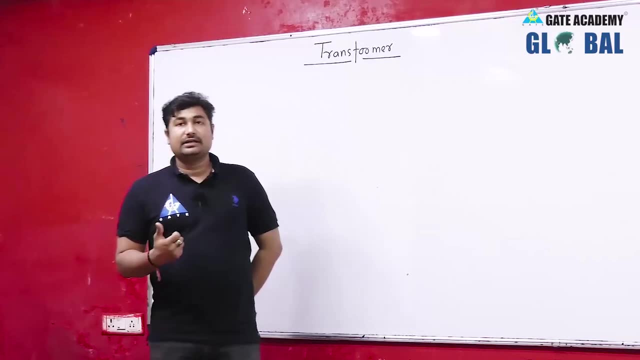 possible for all the electrical machine to work Faraday's law off electromagnetic induction. Faraday's law off electromagnetic induction, you can see it states that whenever fluid oil is kill by media. So here you can see that is where your power is going to do it, so that the energy, that is law, will be Gruberitten. course. There you went. So the電気 which we are working on is Condensate, which will, when I turn on kind of electricассay we are getting, and electromagnetic induction, you have to figure out what. if you are working c-direction, Now h, your number, you can use that over the parameters and, of course, Мы. 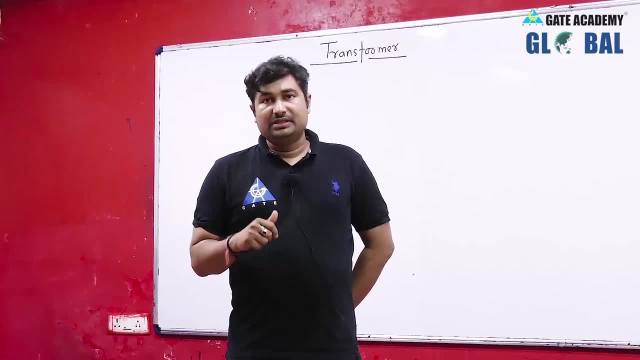 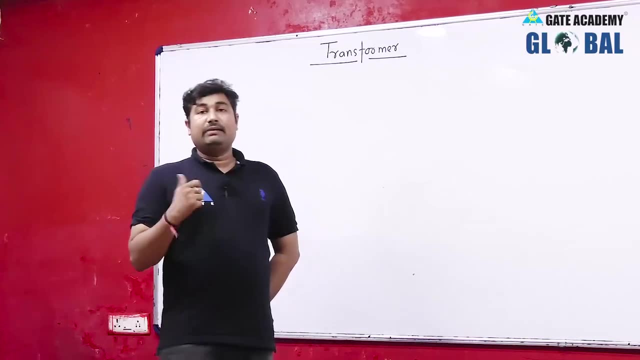 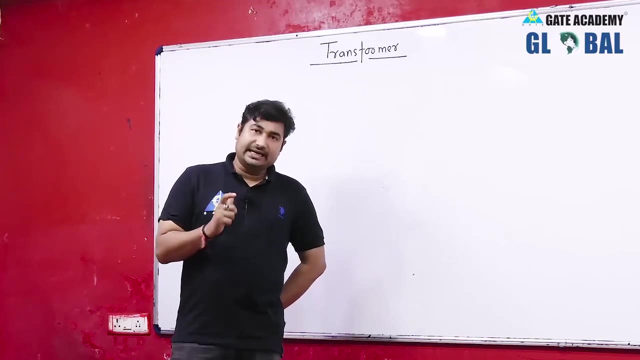 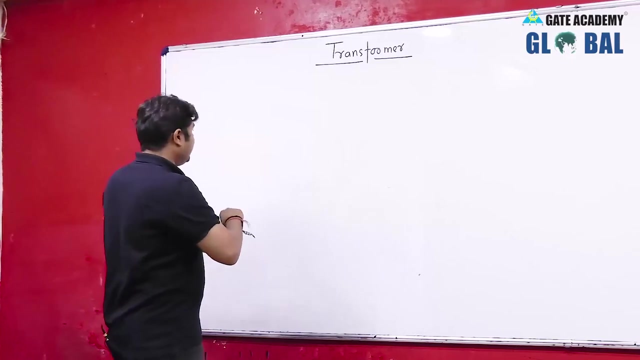 flux linking the coil changes with time, there will be a induced DMF across the coil. Again, I am repeating: whenever flux linking the coil changes with time, there will be a induced DMF across the coil And the induced DMF is expressed. as I am saying, Faraday's law of 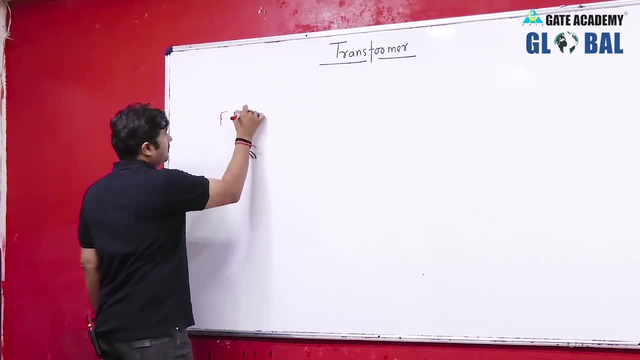 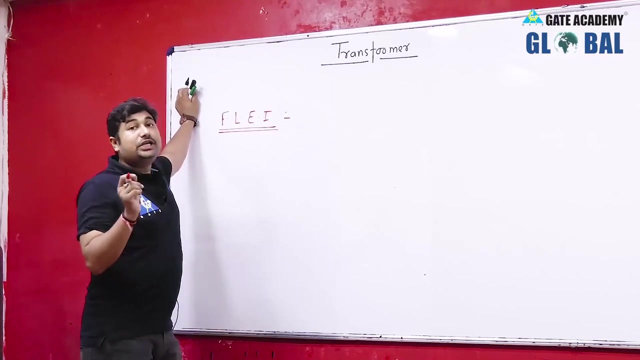 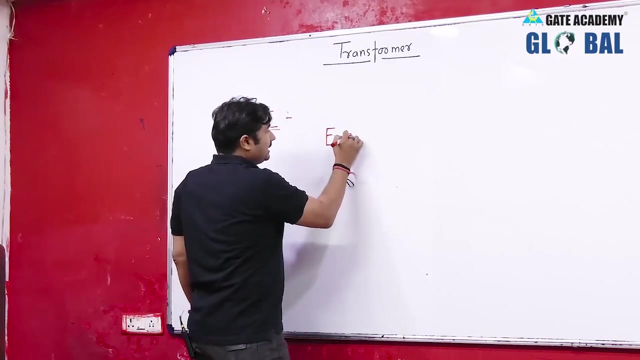 electromagnetic induction. Faraday's law of electromagnetic induction. Faraday's law of electromagnetic induction: It states that whenever flux linking the coil changes with time, there will be a induced DMF across the coil, and that induced DMF can be expressed as: E is equals to plus minus. 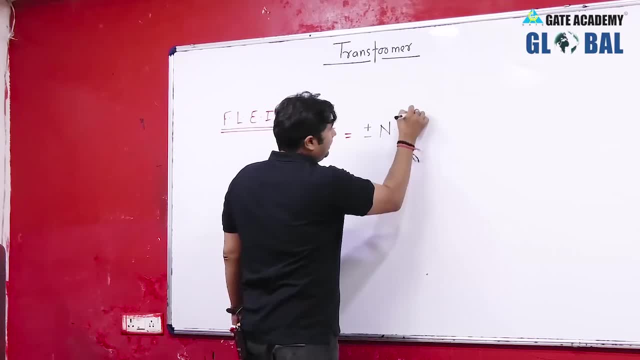 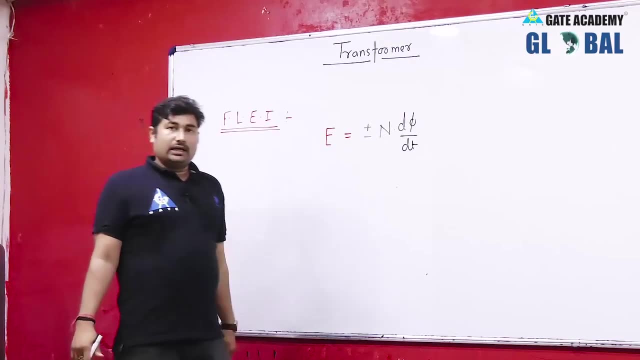 n d phi by dt. I am hoping all of you are aware with this term. So whenever flux linking the coil, whenever flux linking the coil changes with time, there will be induced DMF across the coil and it is expressed as plus minus n d phi by dt. 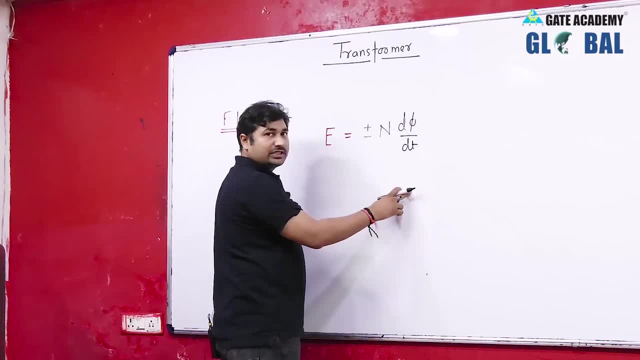 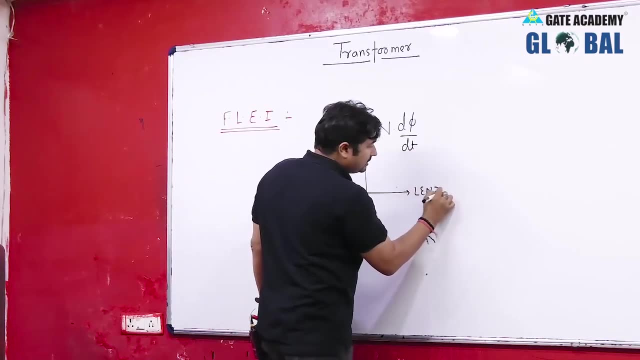 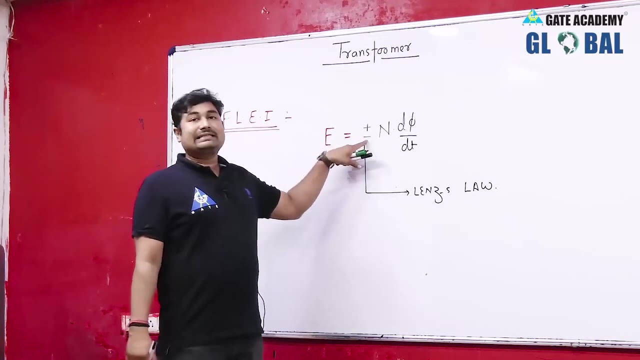 Where n is the number of turns of the coils with which this varying flux is linking, Where this sign is due to the Lenz law. You can say, sir, what is this plus and minus? Most of the books will just represented minus, n, d phi by dt. However, it may be plus or it may be minus. 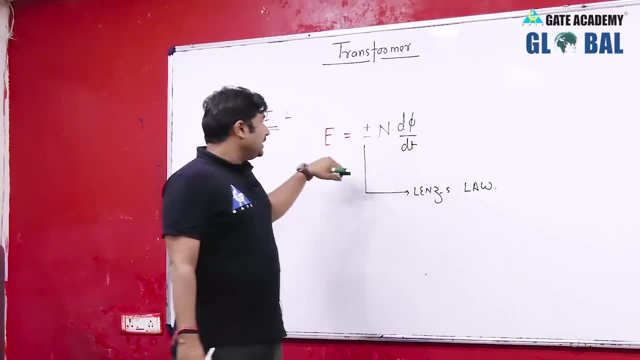 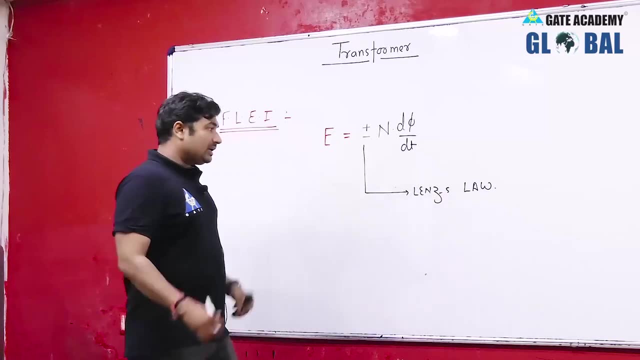 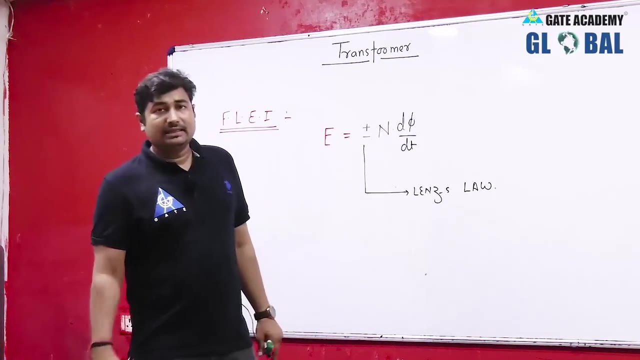 it totally depends upon the our side of consideration. So induced GMF is plus minus n d phi by dt. where this plus and minus sign is due to the Lenz law. What Lenz law says? Very simple: every in each action there is equal and opposite reaction, and it is in electrical domain explained: 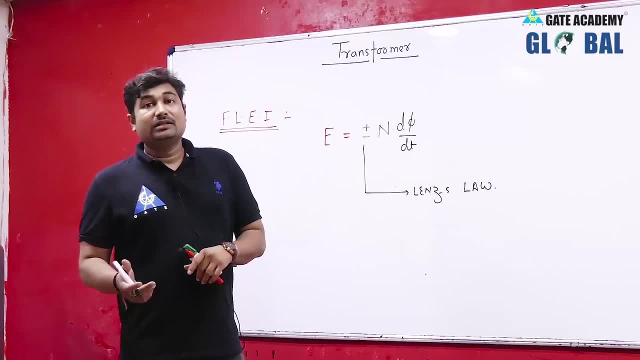 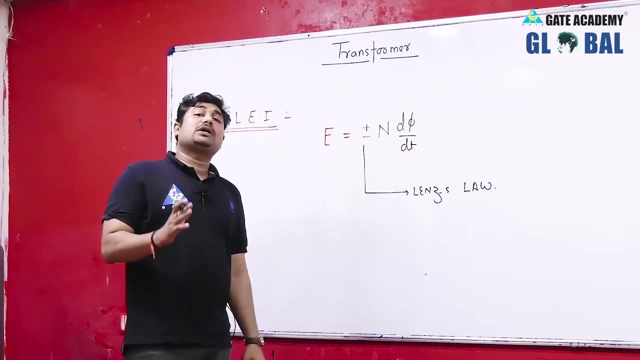 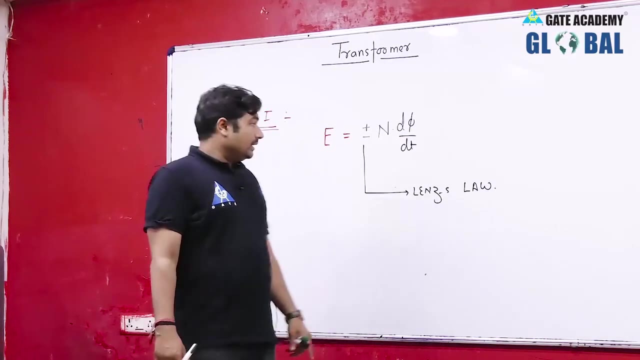 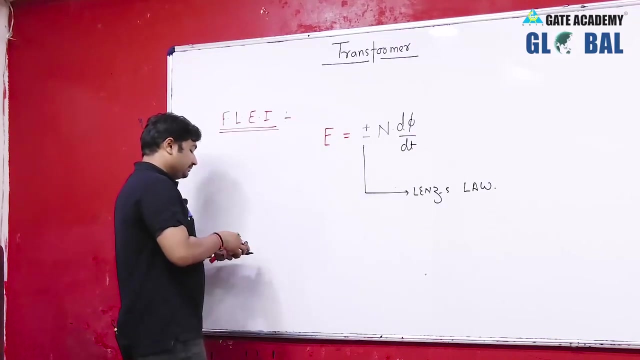 by the Lenz law. Lenz law says the polarity of induced GMF must be such that if it allow to cause a current, then current so produced must oppose the cause. Lenz law says that the polarity of induced GMF must be such that I am representing here. 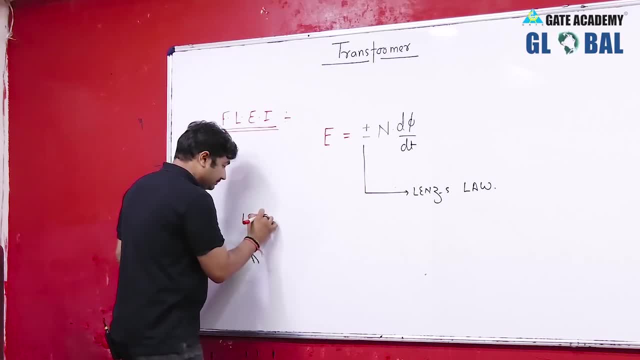 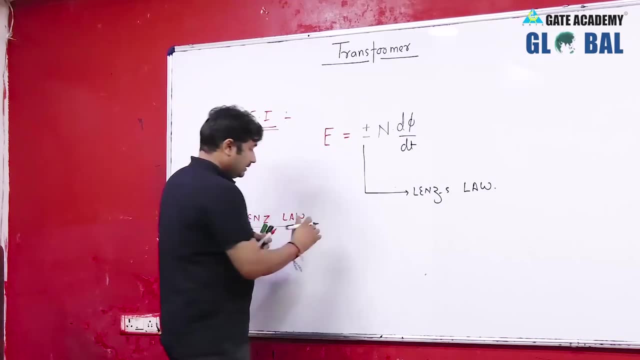 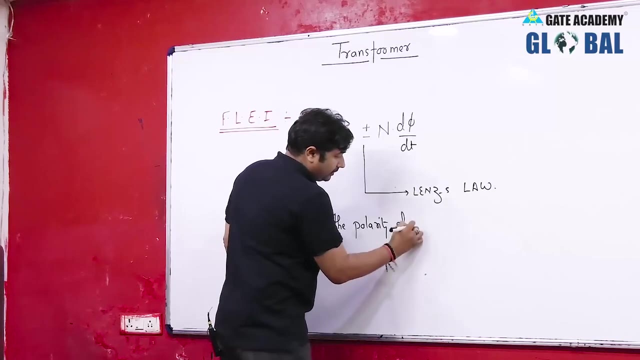 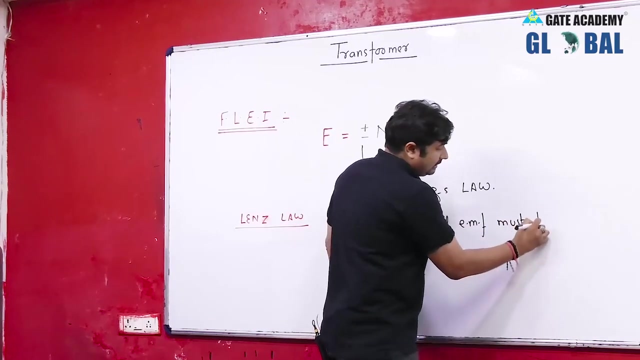 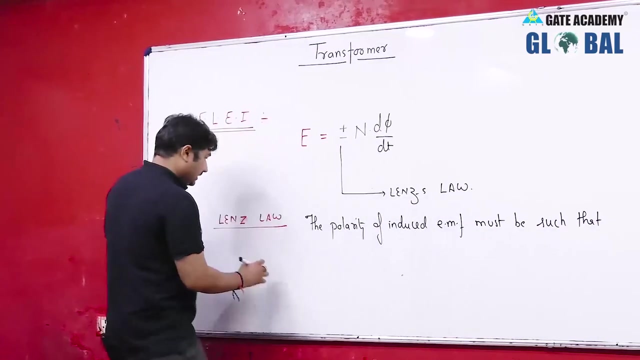 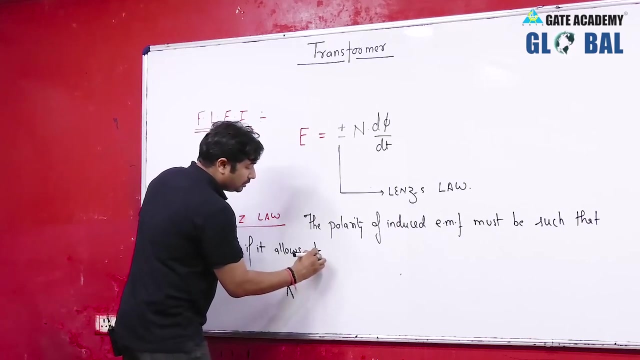 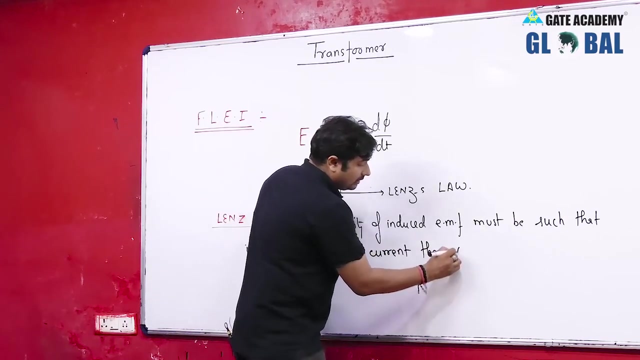 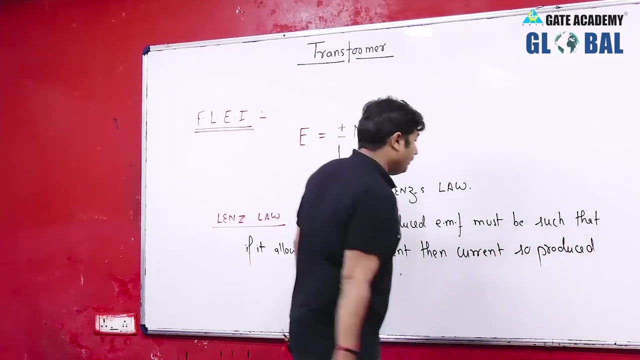 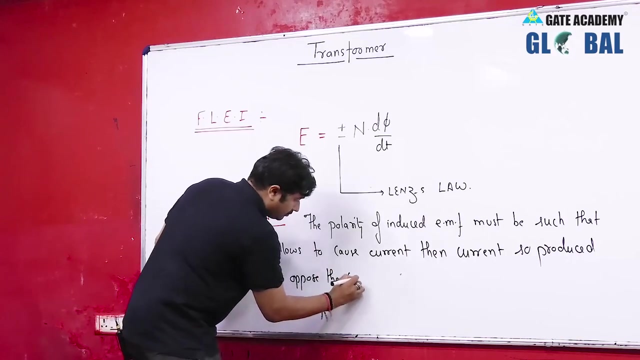 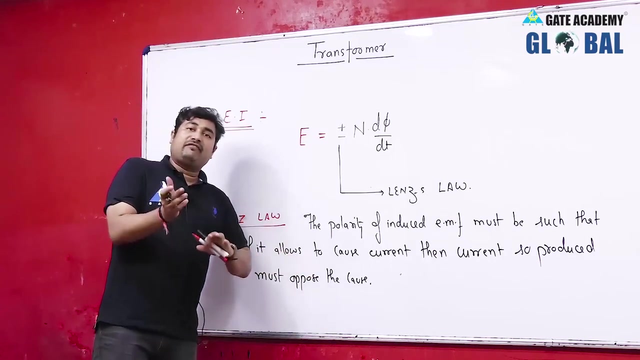 Lenz law says: yeah, you can say. Lenz law states it states the polarity of induced EMF must be such that If it allow to cause a current, if it allow to cause current, then current so produced must oppose the cause. So Faraday suggested that whenever there will be a flux linking the coil changes with 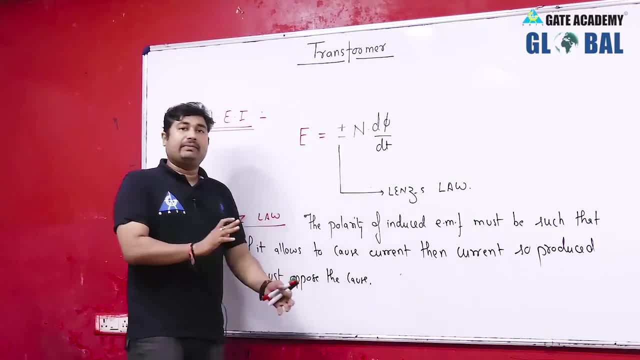 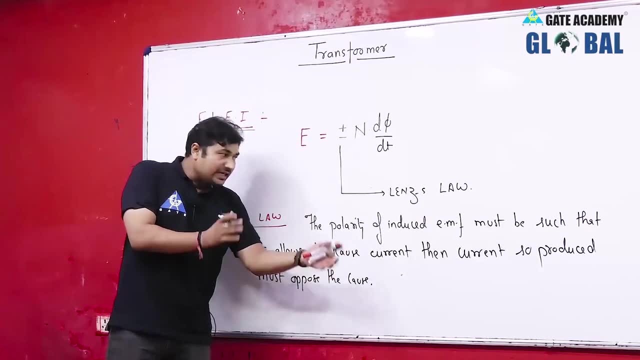 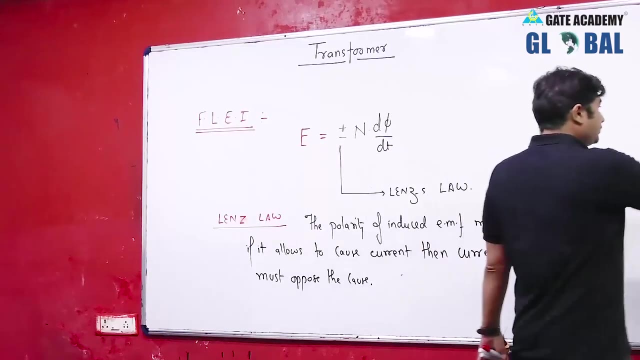 time there will be a induced GMF, and that induced GMF is n? d phi by dt Lenz suggested that the polarity of induced GMF, due to Faraday's law, is such that if it allow to cause a current, then current so produced must oppose the cause. Now see next we know to about the right hand. 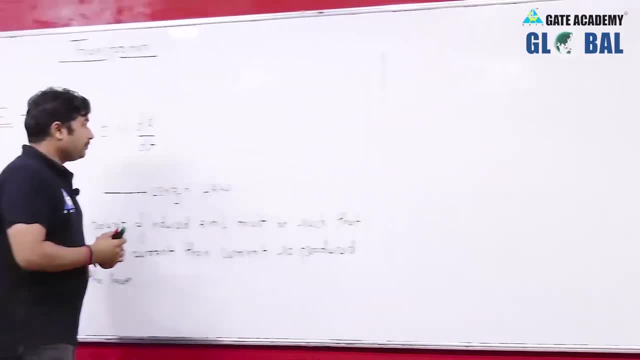 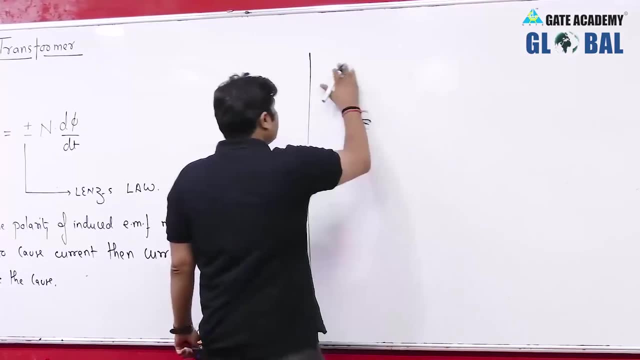 curl rule. So we can easily understand all these laws, I will give you one numerical in order to understand all these. Now please observe right hand curl rule. this is the most important rule. What is right hand curl rule? Before going to right hand curl rule, let us first 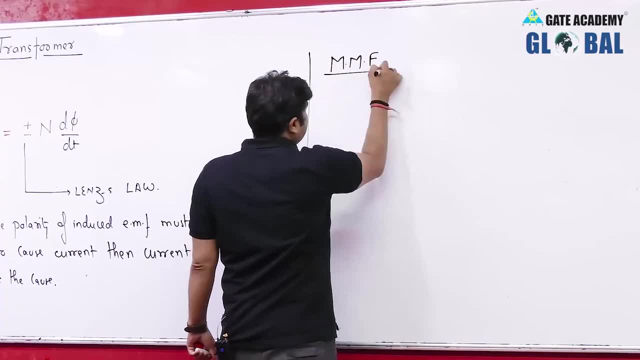 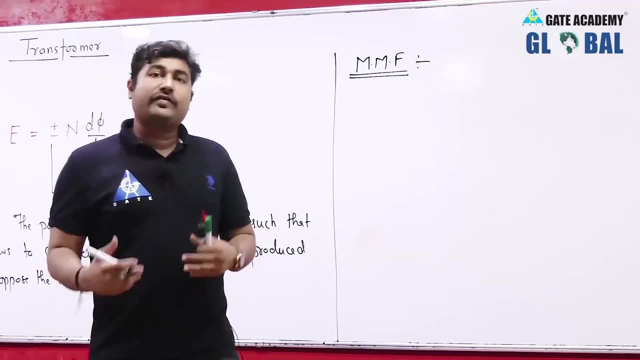 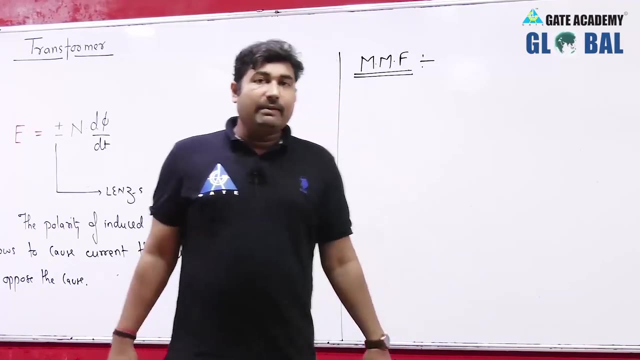 say MMF, that is magneto-motive force. What is MMF beta? It is very similar to EMF. Like EMF is responsible for the motion of current in the electrical circuit, MMF is responsible for the motion of flux in the magnetic circuit. So MMF is responsible for the motion of flux. 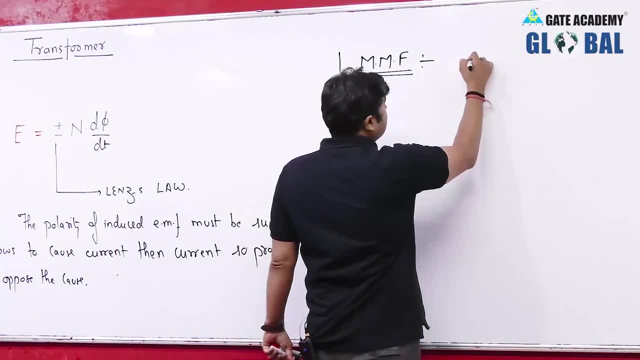 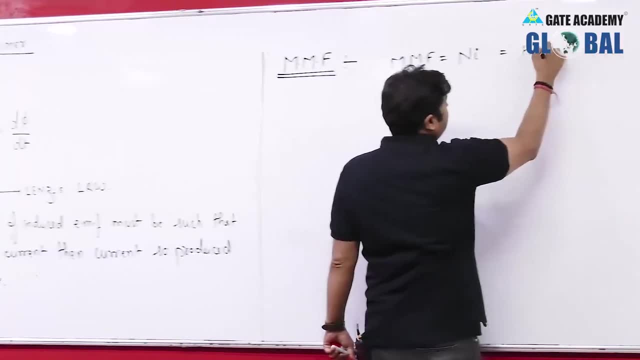 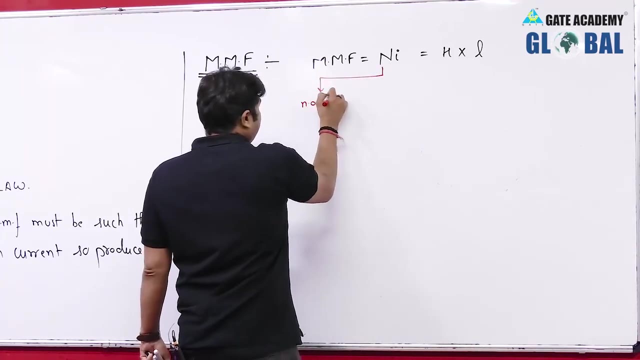 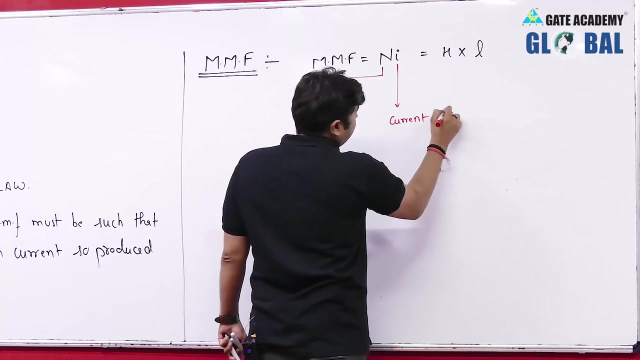 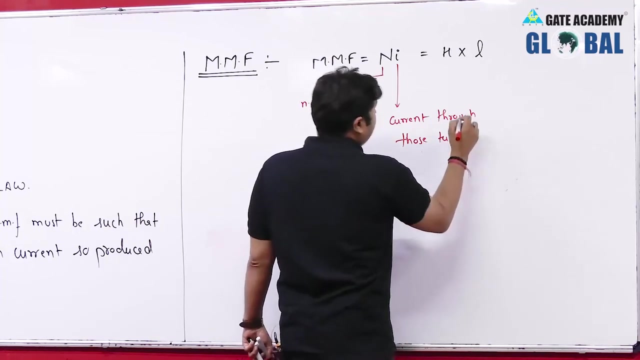 in the magnetic circuit. What is MMF? You can say so. MMF is defined as n into i. or you can say so: h into l, where n is the number of turns, where n is the number of turns, i is current through those turns, current through those turns, and h is magnetic field. 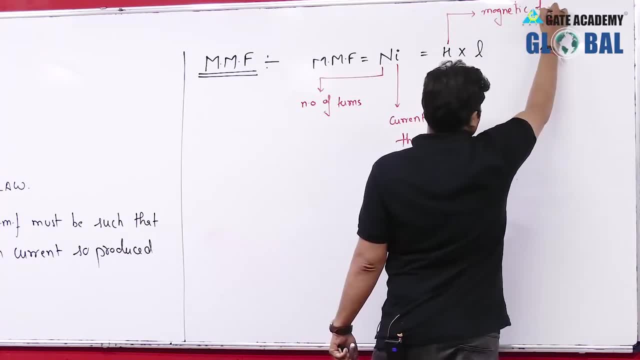 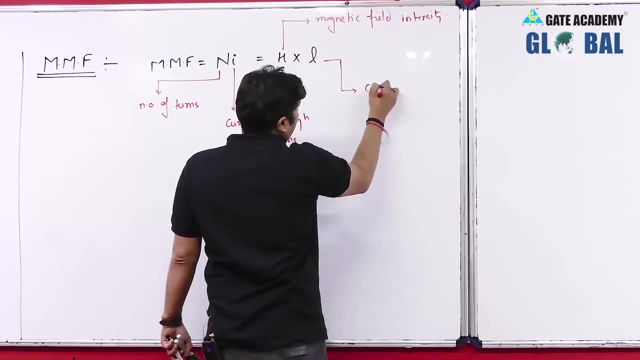 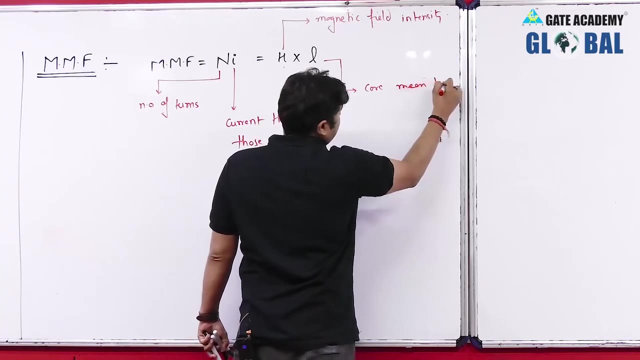 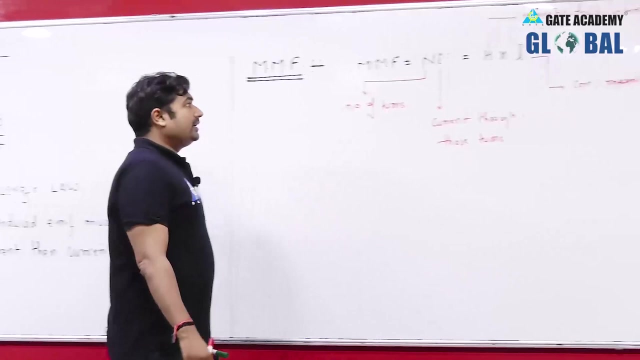 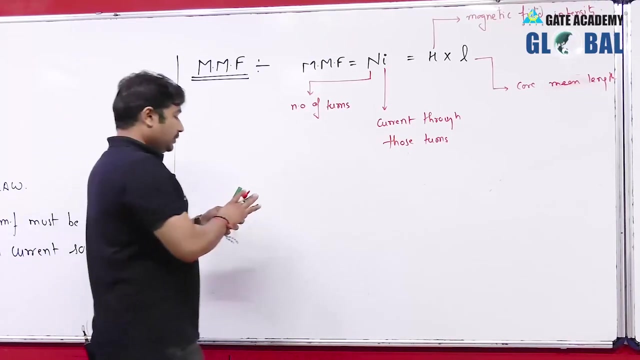 intensity, magnetic field intensity, l is core, mean mean length, So you can say so. MMF is defined as n into i or h into l, where you can say so: h is the magnetic field intensity and l is the mean core length. You can also say so. we know about. 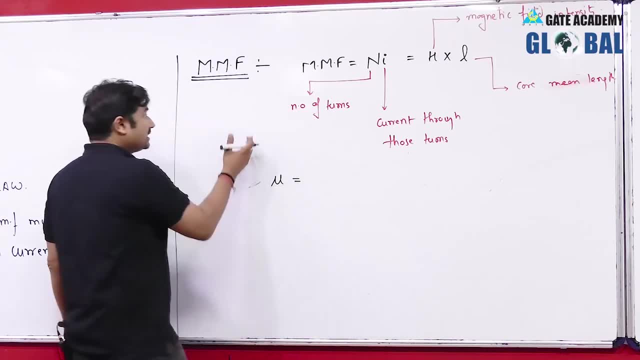 mu. that is permeability. I am just explaining the terminologies which is going to be used for this transformer, So please observe. Next is your permeability. What is permeability? Permeability is mu naught into mu r. where mu naught is the permeability. 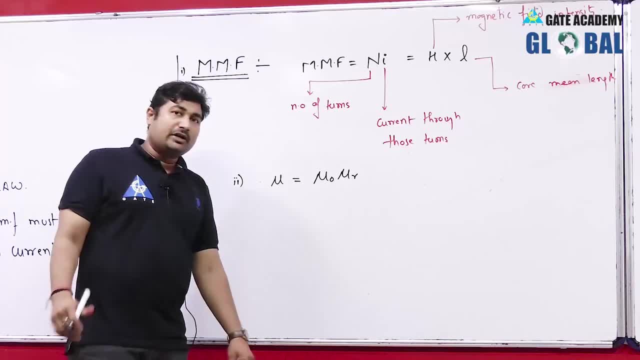 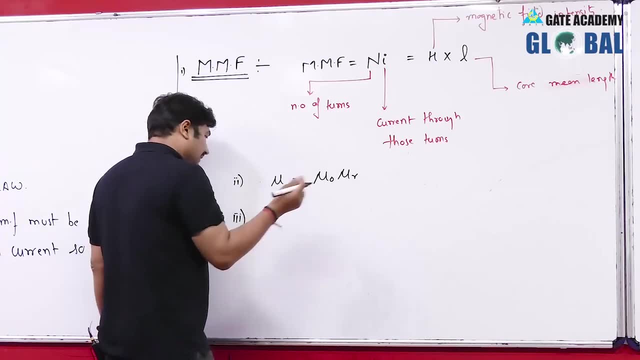 of free space. We all know that 4 pi into 10 to the power of minus 7, and mu r is the relative permeability. Further we can say so for the magnetic circuit. these are some basic relations which is needed for the transformer. Please follow all, Then you can say so magnetic. 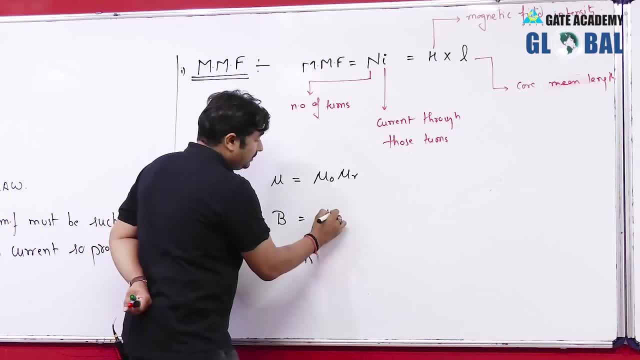 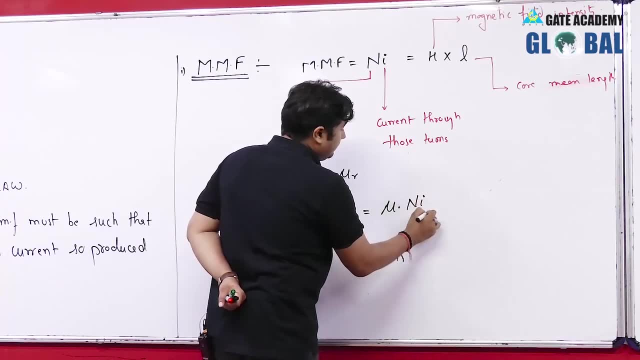 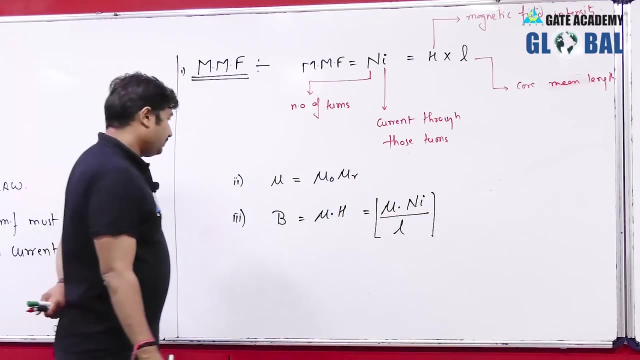 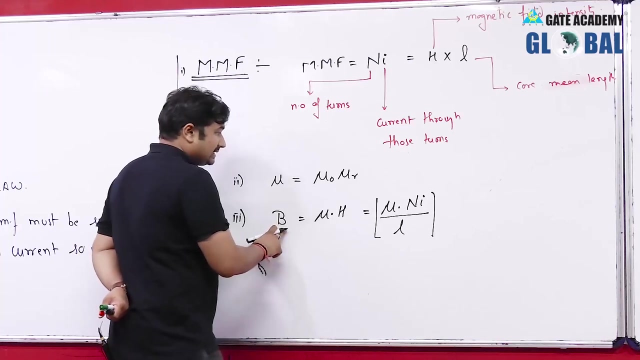 flux density is equal to Magnetic flux density is equal to Magnetic flux density is equal to B. mu into h, where h is. you can say so. mu into n? i by l. From the above I can write mu n? i by l. You can also say so. flux is flux density, B is your flux density and B can be. 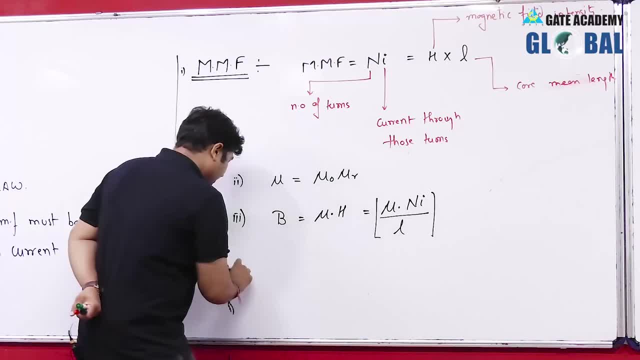 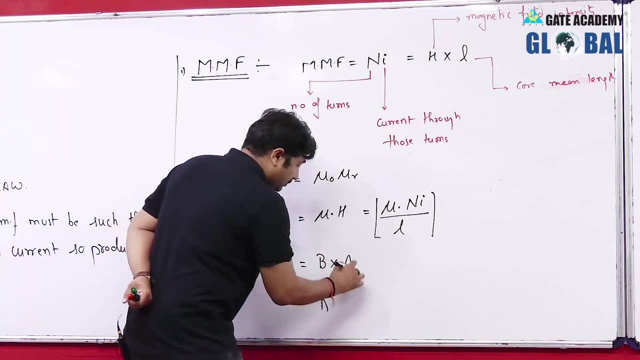 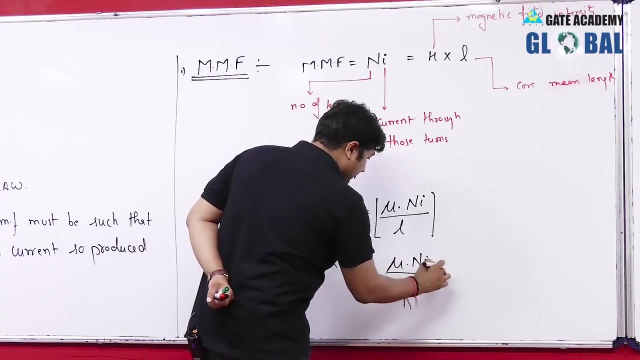 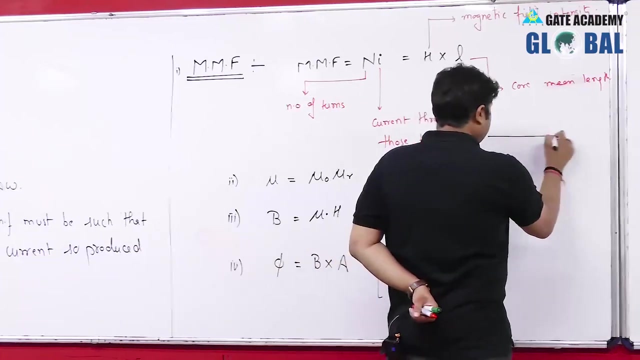 represented as mu into n i by l. Further you can say so we have flux, that flux is flux density into area of cross section of core. So one can say so mu into n i by l into a, That a is area of cross section of core. Let us suppose we have the core in. 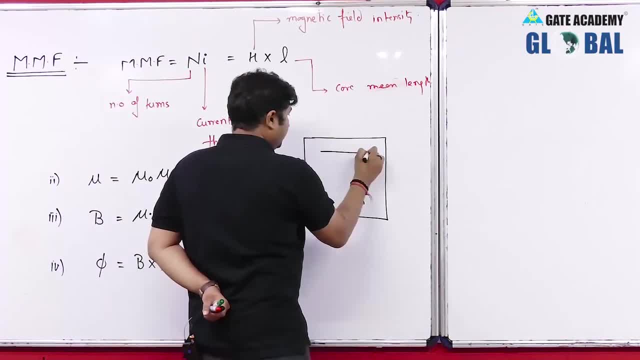 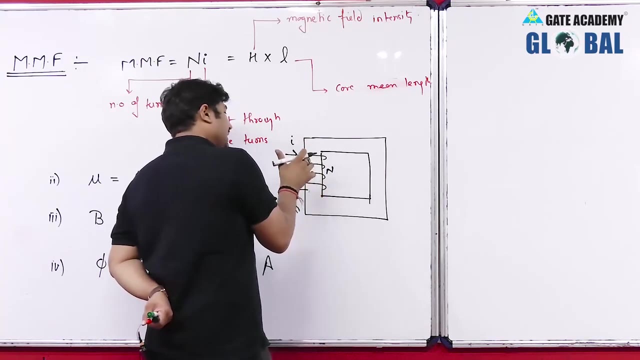 this way. So if this is your core, then n is the number of turns on this core. n is the number of turns on this core. i is the current flowing in these turns. So this MMF, this will produces MMF, or you can say this is responsible for the motion of flux. Let 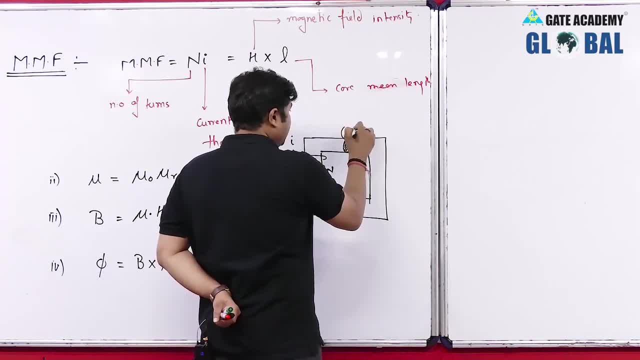 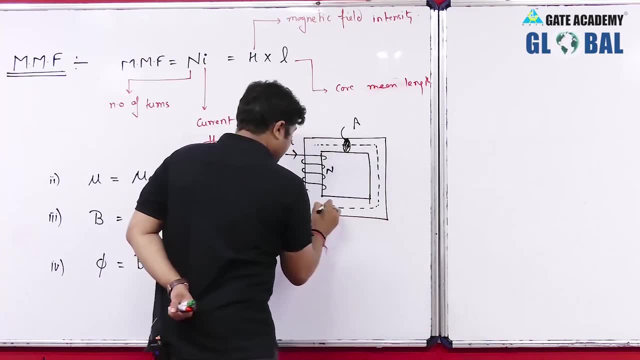 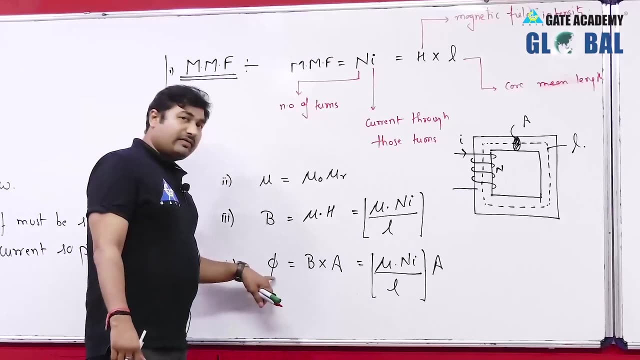 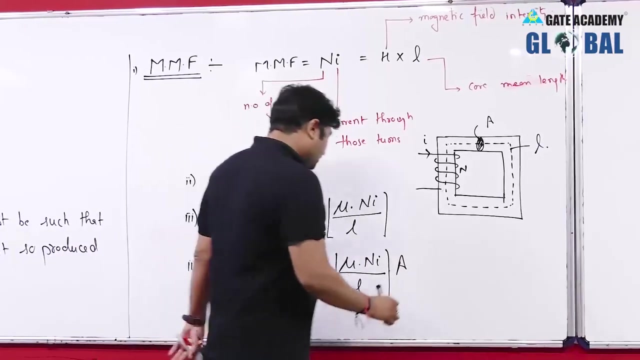 us suppose this core will have area of cross section a and this core will have mean core length of l. So I am representing this to be the mean core length l. So one can say: So let us suppose this is ați. 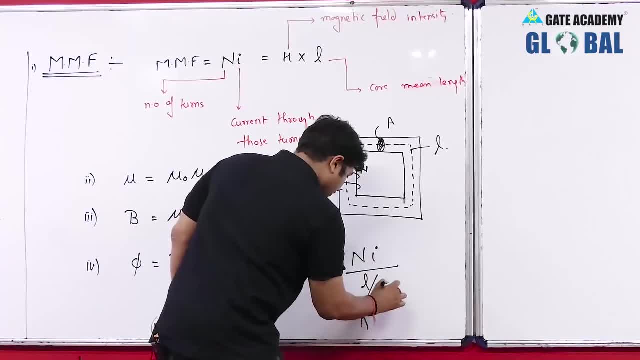 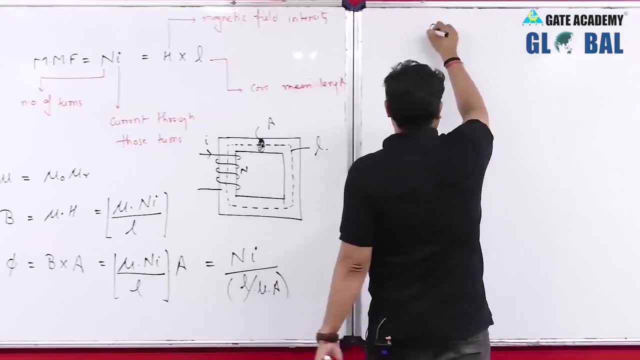 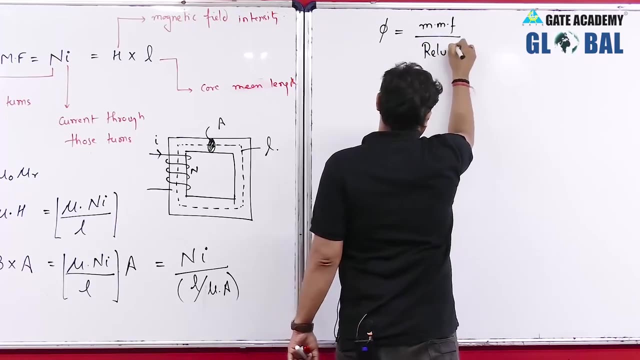 So if, let us suppose that you flowing in thecje of corridor, let us suppose for e i, mu fc, now this operation will be stretched here. So if, if you like, you can go and identify that out, then to separate m fc and to find this out so that, as you can see, or 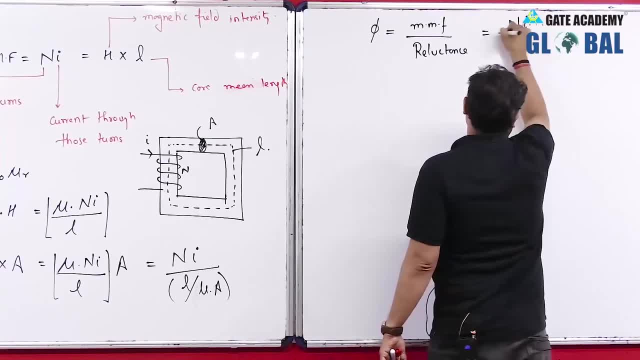 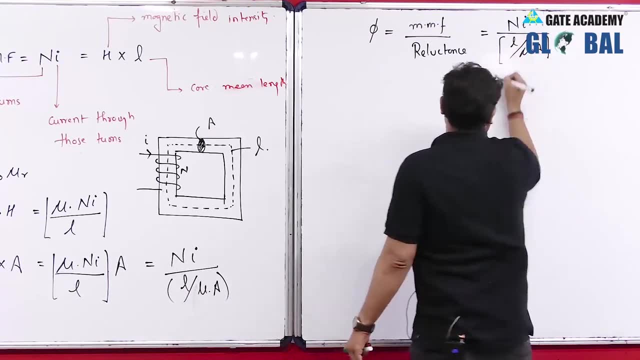 let us say So you can choose whatever you want From here. That means this is actually. this is little bubble. If you set it, let us assume that if this is the can flow this methods N into I by reluctance is L upon mu into A. Reluctance is very similar to resistance, like 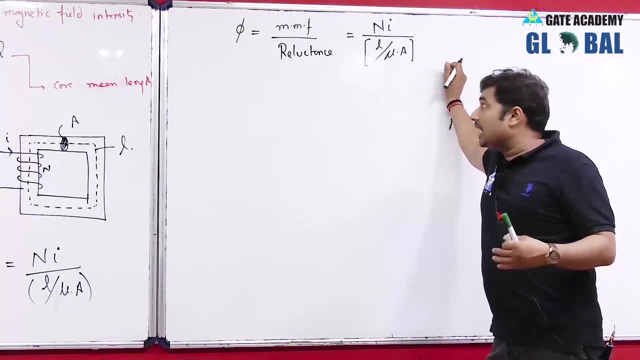 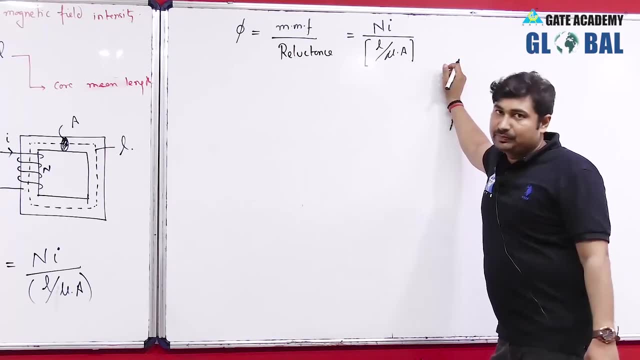 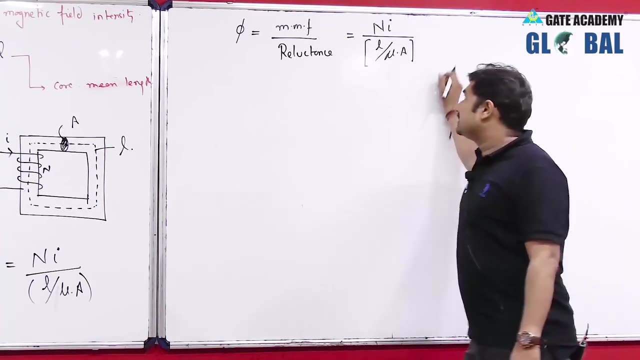 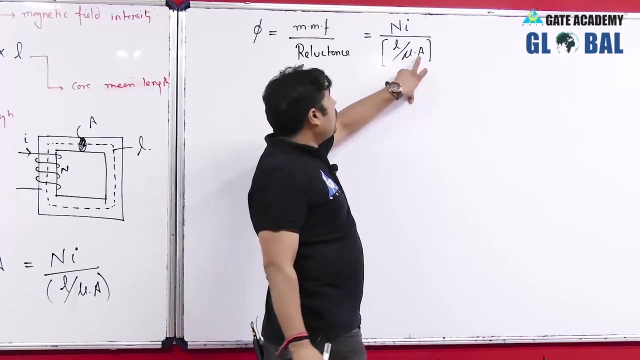 in electrical circuit, resistance does not allow the flow of current through them. Similarly, in magnetic circuit, reluctance opposes the flow of flux. You can say, sir, lower reluctance means higher the motion, higher the magnetic flux. You can say, sir, reluctance can be decreased by either increasing the area of cross section of core or by increasing the relative permeability. 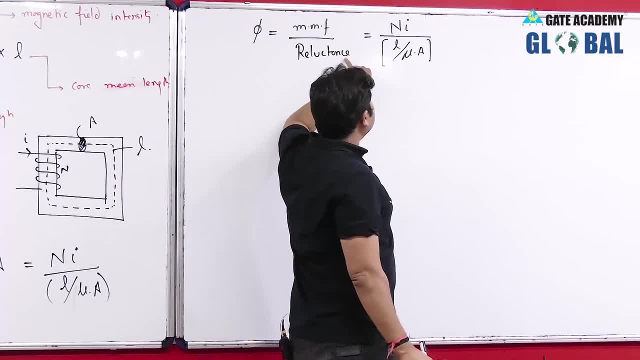 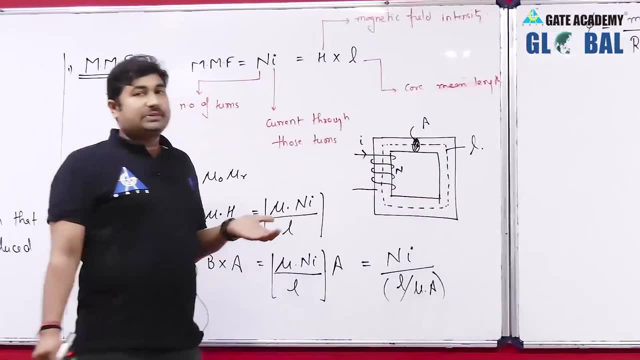 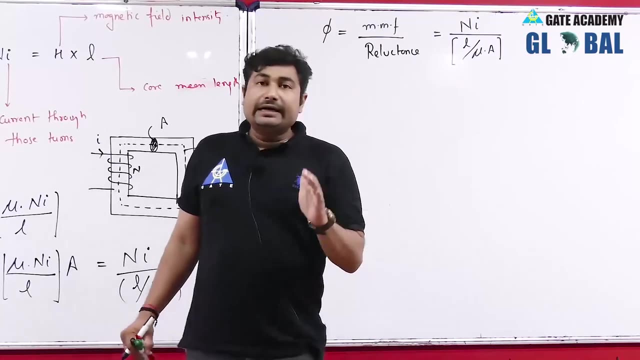 or you can say, sir, reluctance can be, reluctance can be decreased by decreasing the mean core length. So you can say, sir, reluctance can be increased by increasing the relative permeability or area of cross section of core. Lower reluctance means what: Like current, always likewise current, always try to flow. 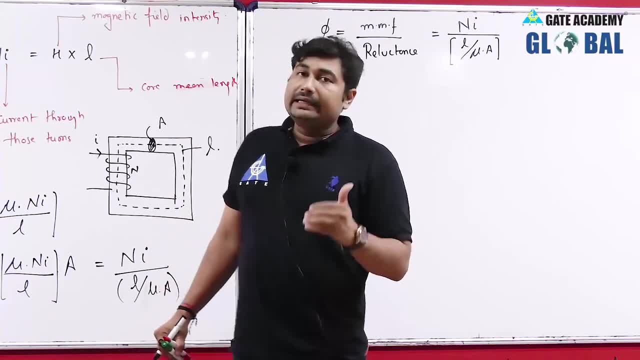 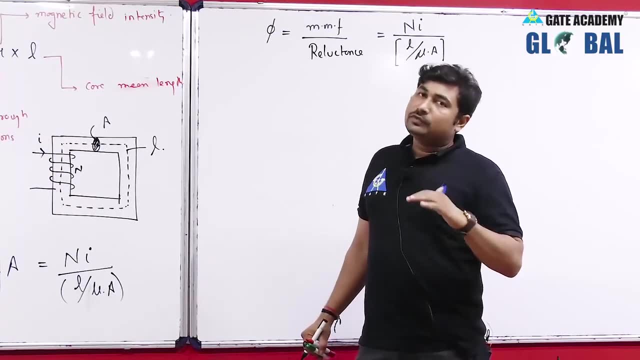 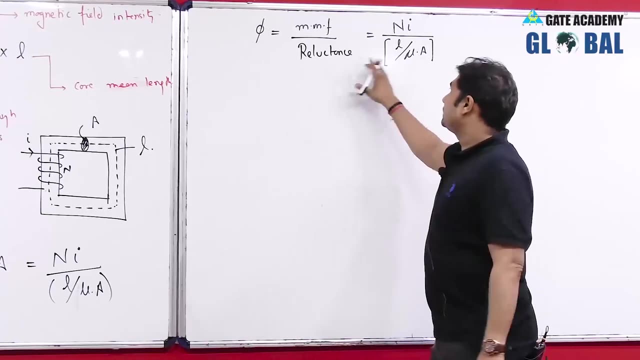 through the low resistance path. magnetic line of forces always try to flow through the minimum reluctance path. Current try to flow through the minimum resistance path and flux try to flow through the minimum reluctance path. So reluctance lower means you can say the motion of the flux is easier. So we have: flux is equals to mmf upon mu. 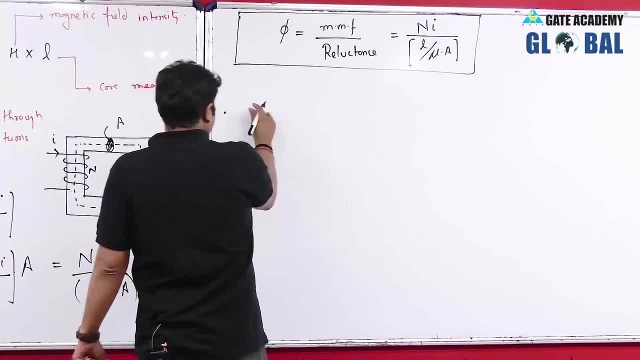 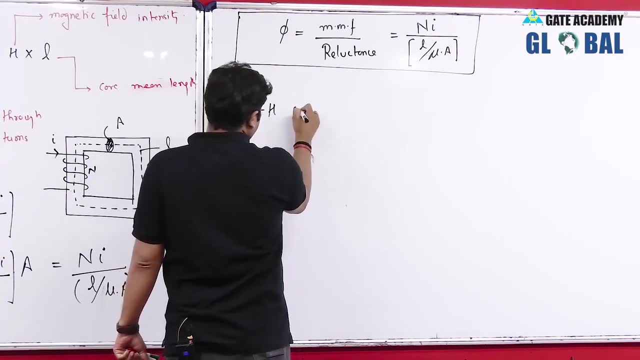 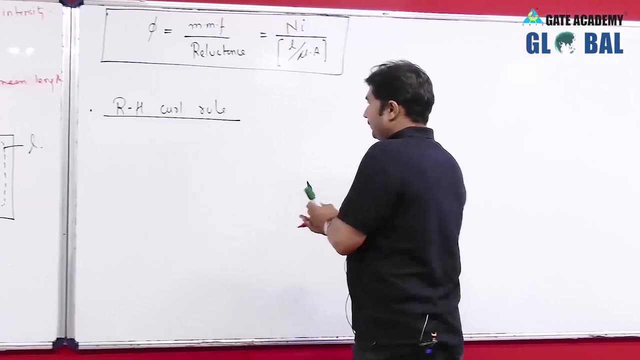 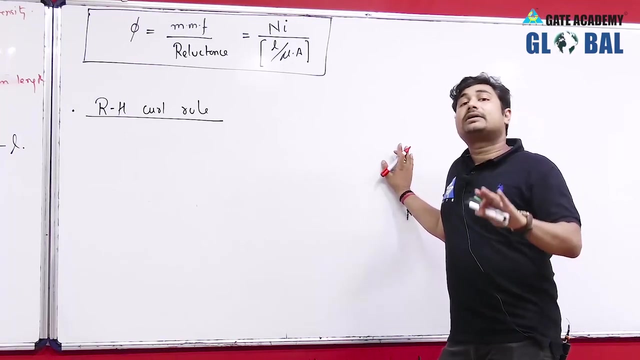 Now please observe the next one, that is, your right hand curl rule. Now, right hand curl rule, right hand curl rule, please observe. We all know that whenever a current carrying conductor, whenever a current carrying conductor, then that conductor will always produces a. 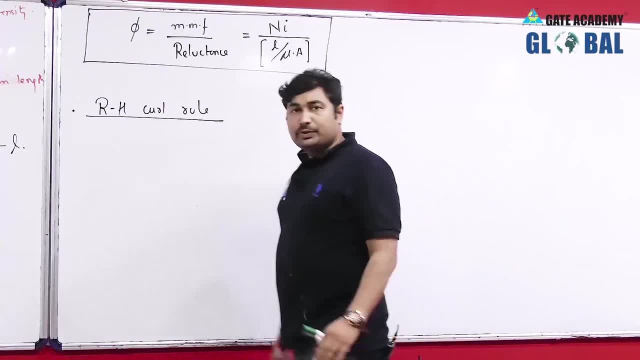 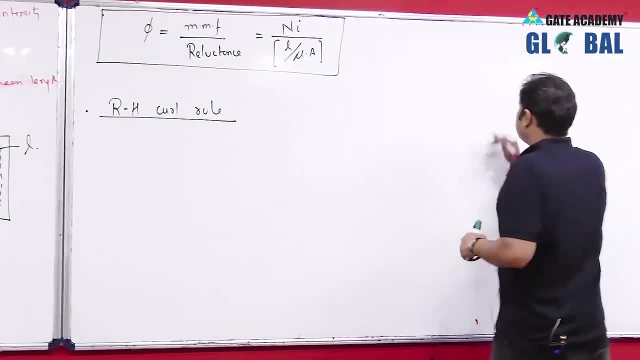 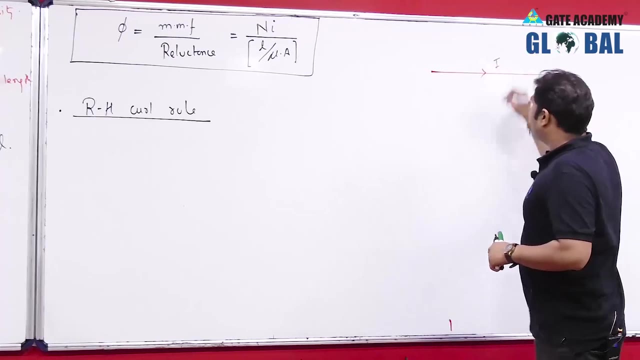 magnetic field. A current carrying conductor always produces magnetic field and the direction of field is found by right hand curl rule. So please observe, let us suppose we have one wire and in this wire current is flowing in this fashion. So whenever current flows in this fashion, whenever current flows through the wire, it 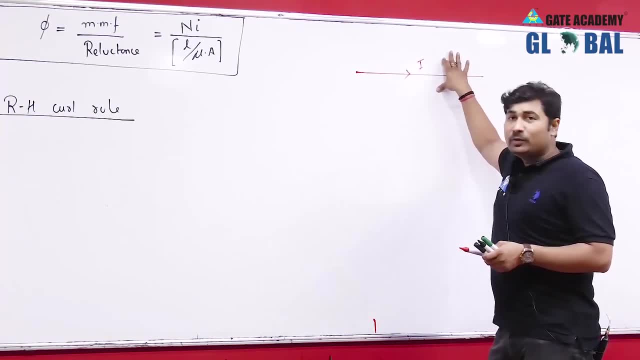 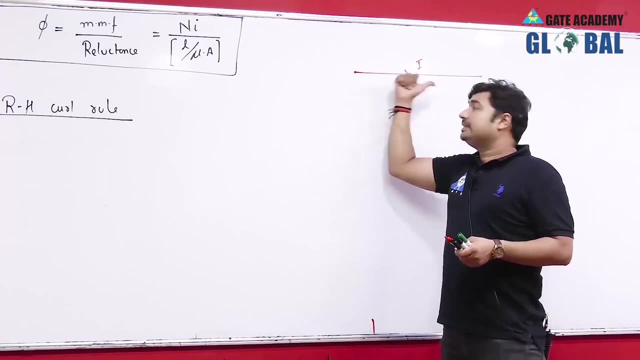 will, produces a magnetic field, and the direction of field is found by right hand grip rule. So if I want to know what type of magnetic field this wire, this current in the wire, produce, we can use right hand grip rule. What is right hand grip rule? The current is flowing. 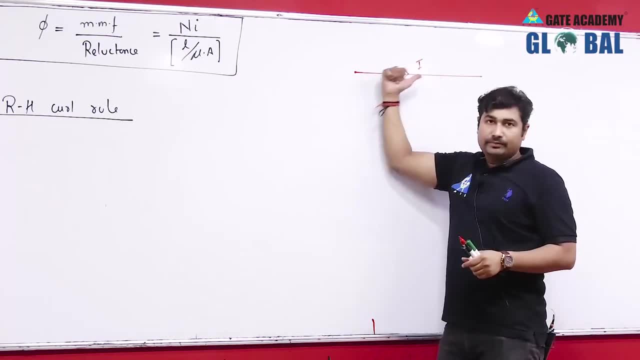 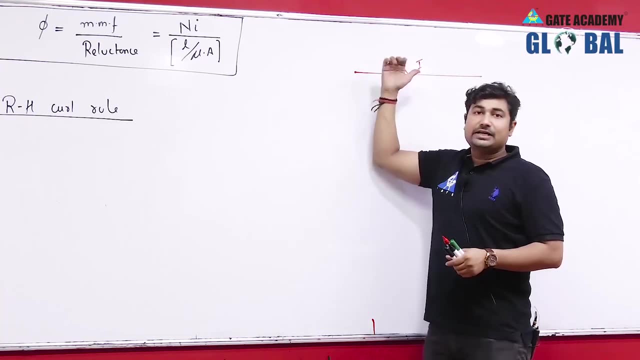 please observe, If the current is flowing in the direction of my thumb, if the current is flowing in the direction of my thumb, then you can say: right hand curl will represent the direction of flux. So you can say, sir, right hand curl will represent the direction. 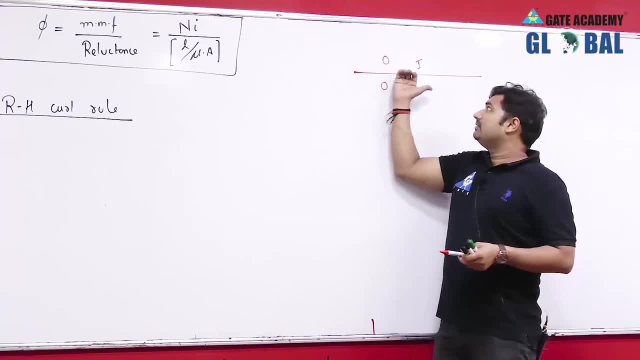 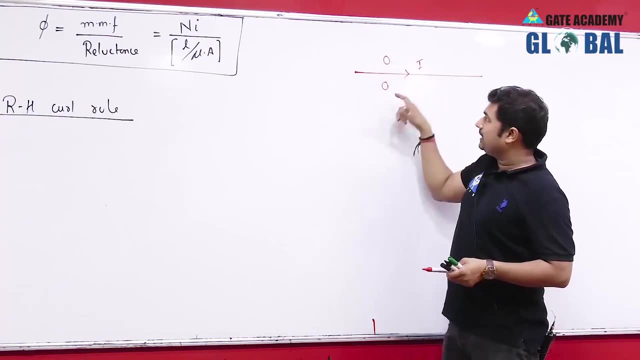 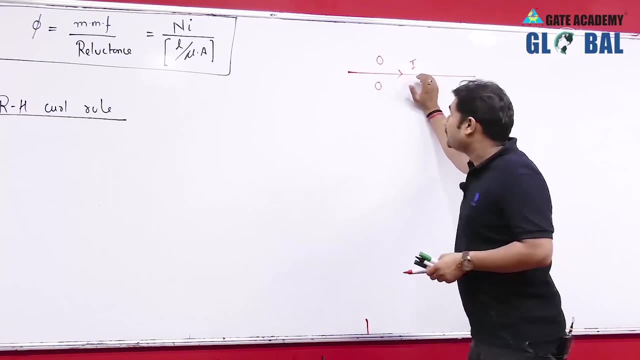 of flux. The right hand curl will represent the direction of flux. It means magnetic line of forces are appearing to be coming out from this port and going into this port. If I am observing from this section, that is from the front side of the board section, So it appears that magnetic line of forces are coming out from. 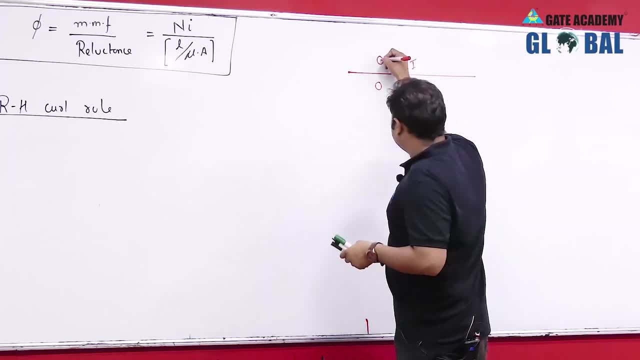 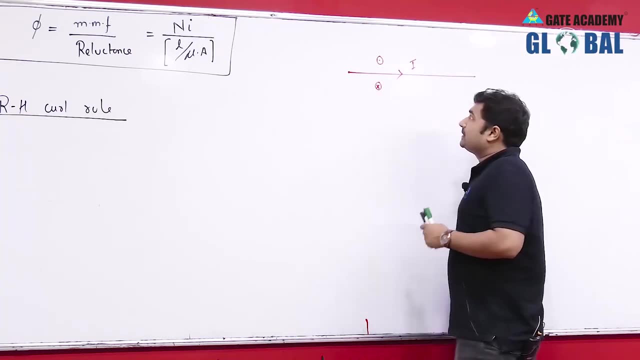 this section and going into this section, You can say: magnetic line of forces are appearing, coming out, can be represented as dot, and magnetic line of forces going into this can be represented as cross. So one can say, sir, that terminal of the magnet is said to be north, which releases. 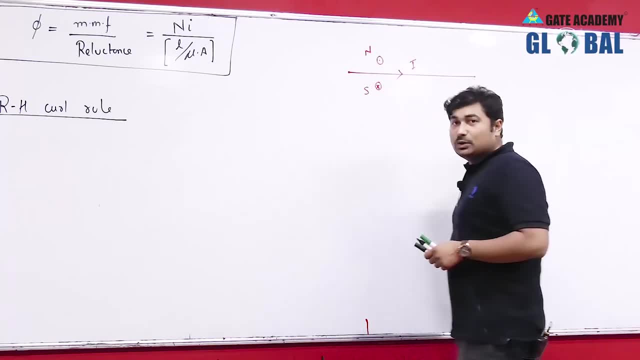 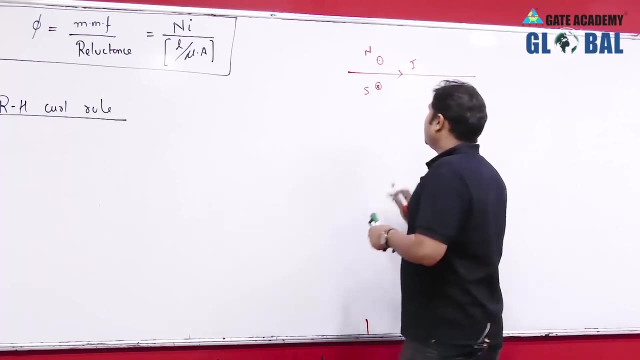 the flux And dot terminal of the magnet is said to be south, which absorbs the flux from the air. So one can say: if the current flows in the direction of thumb, then this will be the direction of magnetic field produced by the current flowing in this wire. You can say, sir, let, 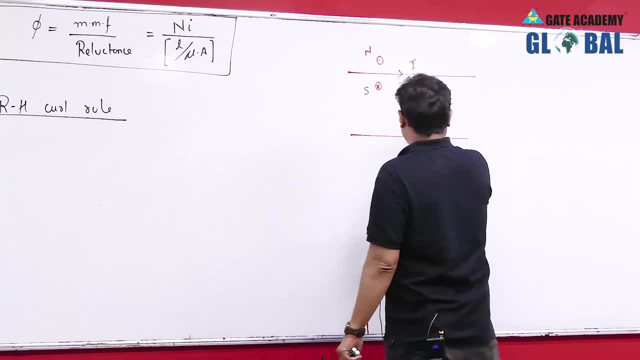 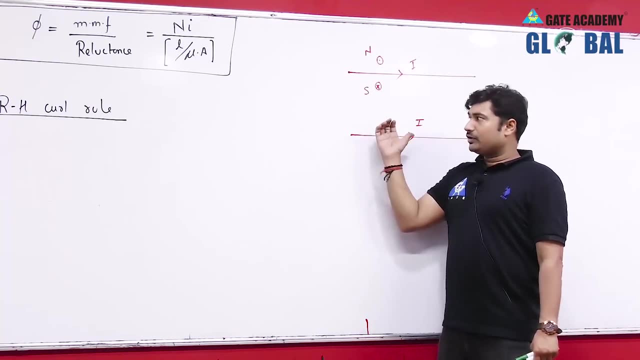 us suppose if we have one more wire and the wire will have the current in this direction. Now please observe, If the direction of current is thumb, then one can say the direction of curl will represent the direction of curl will represent magnetic field. So the direction, 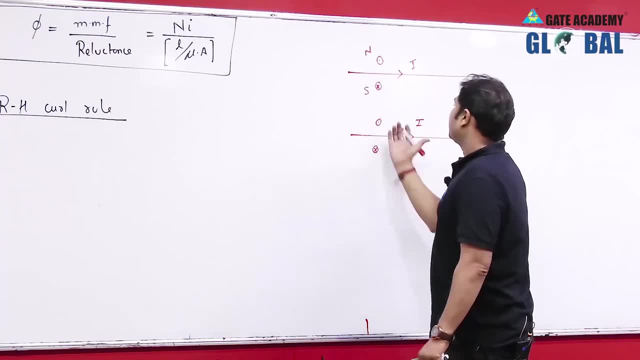 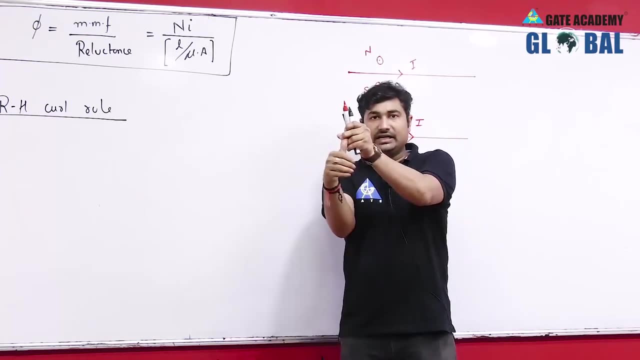 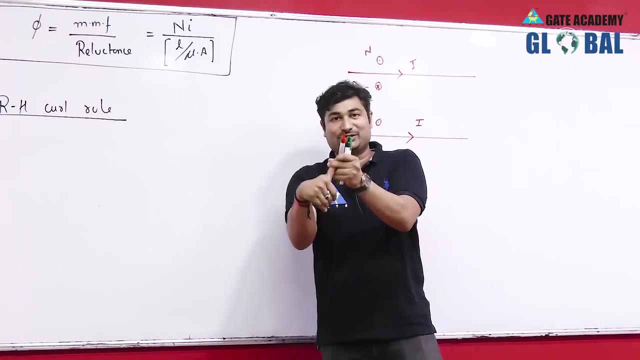 of field can be represented in this way. coming out from this section and going into this section, This is my thumb and this is the curl. the fingers are representing curl, So you cannot make the curl in this way. you can only make the curl in this way, So that 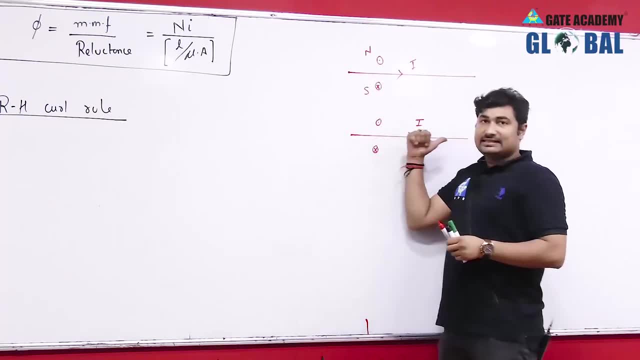 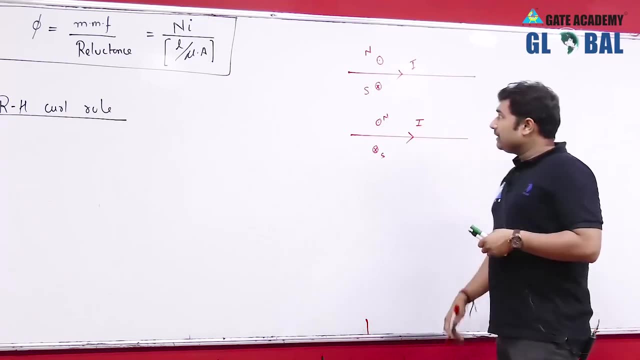 is why it is right hand curl rule. So if the current is in this direction, then the direction of field must be in this way. So this is going to be the north and this is going to be the south. One can also say, sir, from this we can lead to the conclusion that 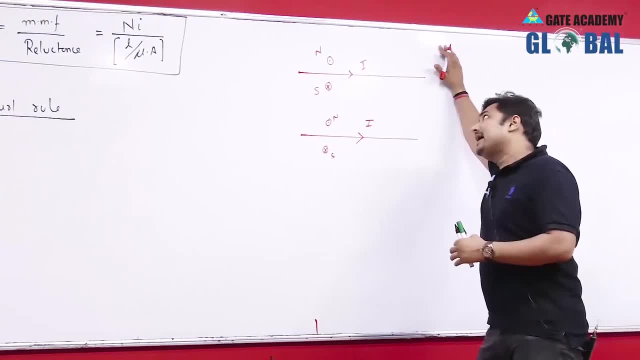 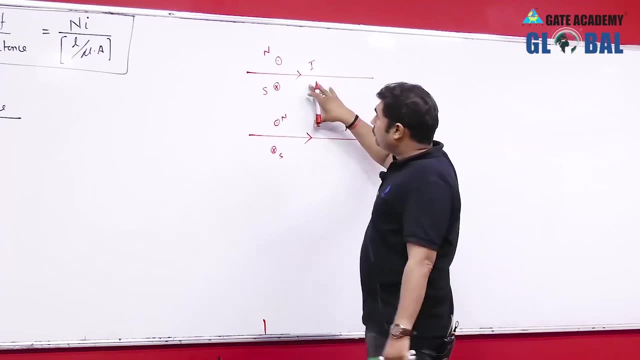 if two wires are carrying current in the same direction, then definitely they. there will be attractive force exist between them. If the two wires are carrying current in the same direction, then there will be attractive force exist between these two wires. Again, please observe. 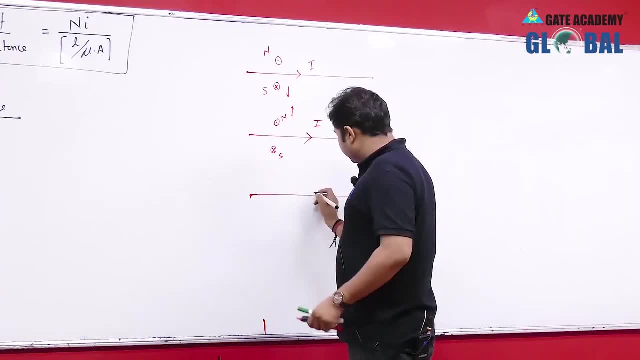 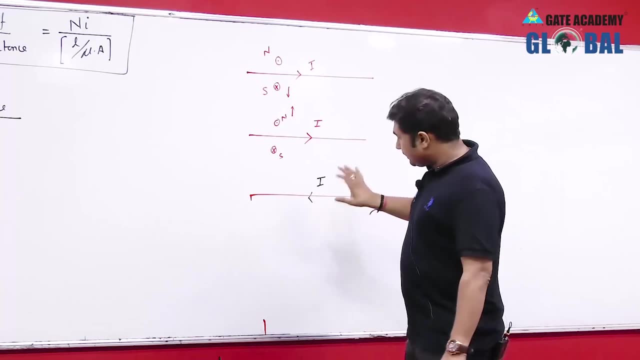 Let us suppose we have another wire and the current flowing in this wire is in this way. If the current flowing in this way, then by right hand curl rule, or you can say right hand grip rule, right hand curl rule, we can find the polarity of magnet. or you can say: 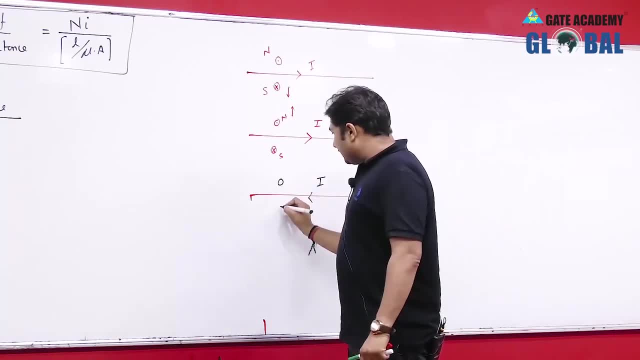 we can observe the magnetic line of forces. If the direction of current is represented by thumb, then right hand curl will represent the direction of field, and the direction of field is appearing in this fashion. So you can say this to be the north and this is the 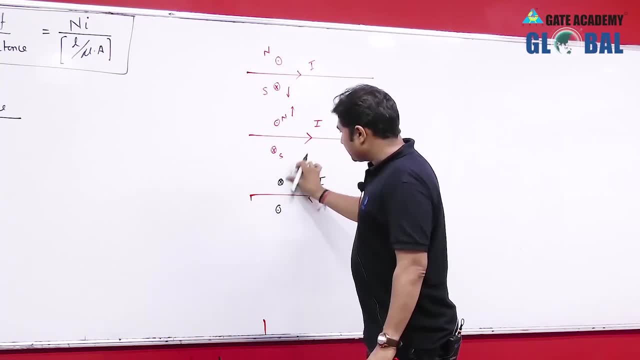 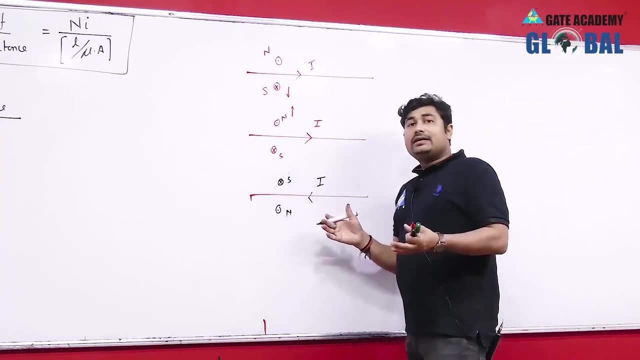 north and this to be the, this to be the north. flux lines are coming out from this port and this to be the south. So one can say, sir, if the two wires carrying current in the opposite directions are placed nearby, then they will faces the force in. 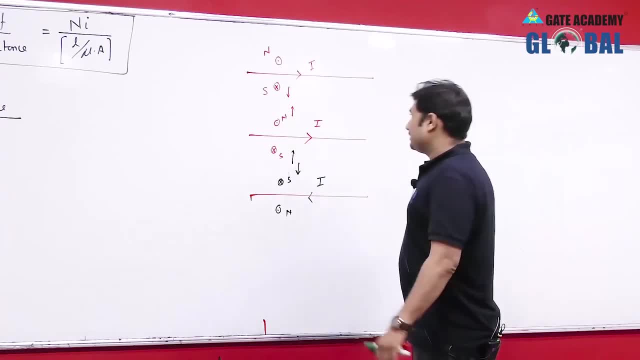 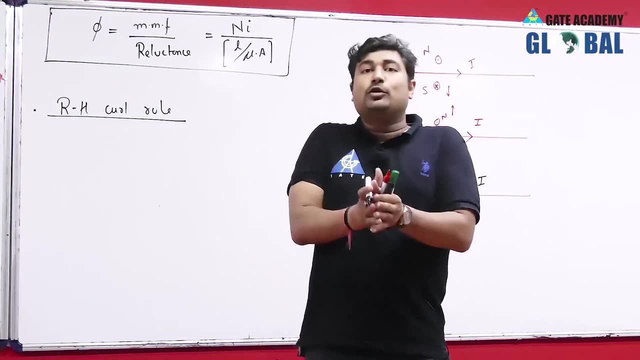 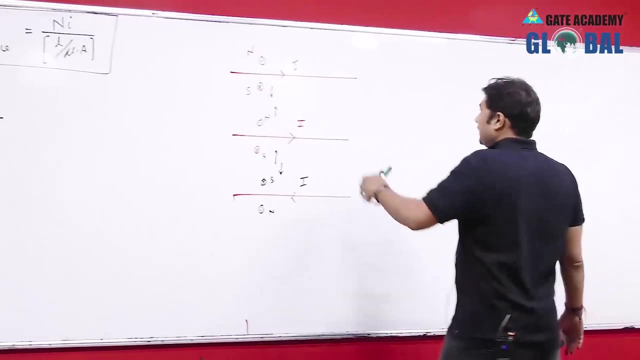 a repulsive manner, Is it ok? So that is very interesting- that two wires carrying current in the same direction will appears attractive force, while two wires current in the opposite direction appears repulsive force. Now please observe, Let us suppose we have a wire and that wire is bounded on some core. 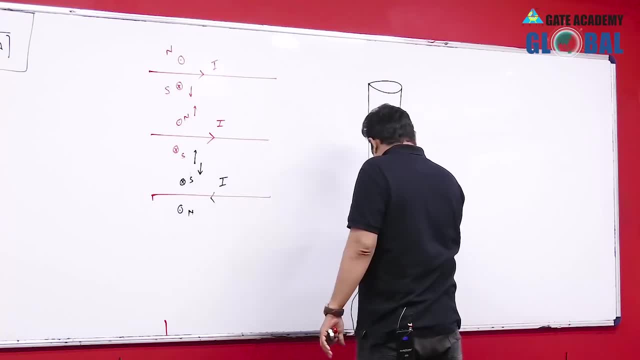 in this fashion. Let it be a iron core, and on this iron core we have a wire and that wire is bounded in this fashion. If the wire is bounded in this fashion- and let us suppose I am giving some DC source to this- Let it be in this way. I am, I supplied this wire. 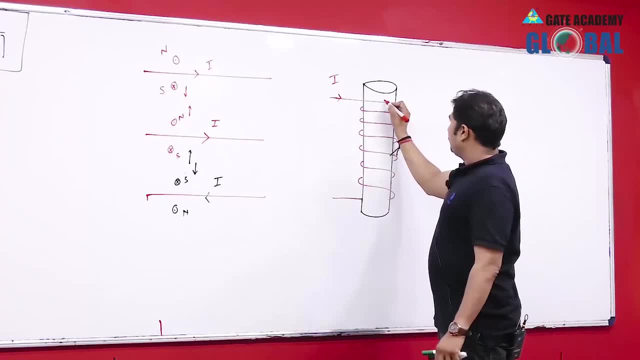 by this current I in this fashion, So the current will flows in this way. that means it will goes in this way to the wire. So if the current is flowing in this fashion, it will produces a field, and the direction of field is found by right hand grip rule. 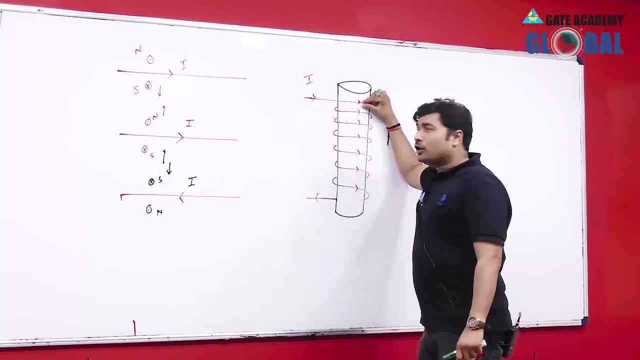 So right hand curl rule suggest that if we observe each of the wires separately, then we found that each of the wires are going to produce some north and south. Please observe, if the direction of current is this, then the right hand grip you can say is representing 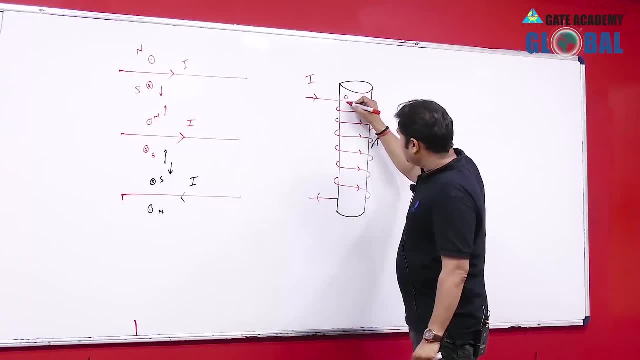 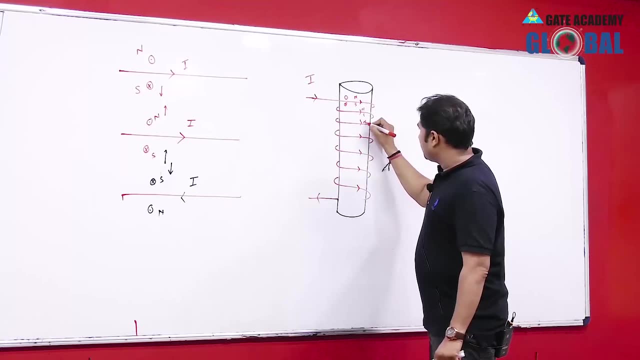 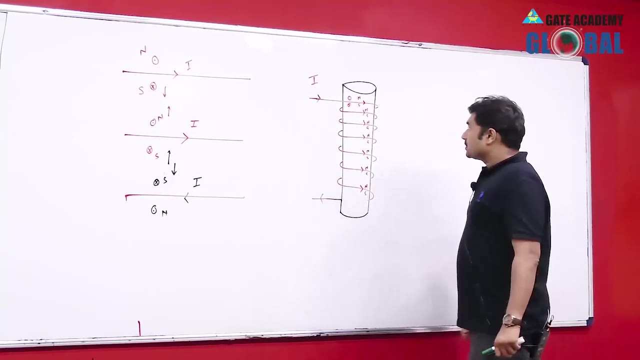 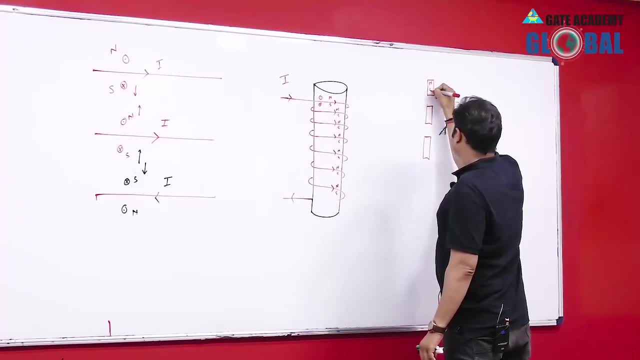 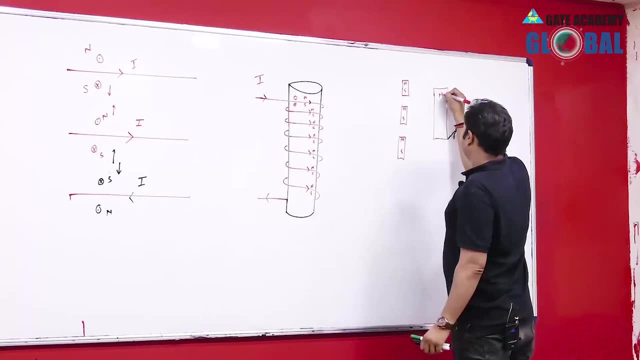 and that magnets will have a polarity of this fashion: north, south, north, south, north, south, south, north, south. If we put all the magnets together then you can say it will act as a big magnet, as north or south Magnetic line of forces always flows from north and it enters. 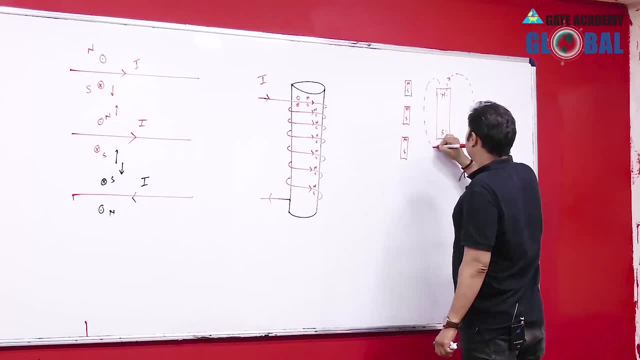 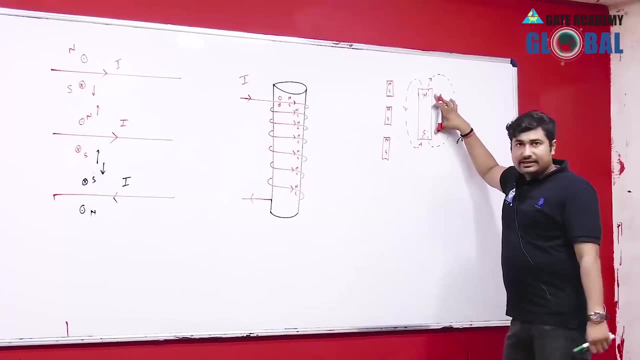 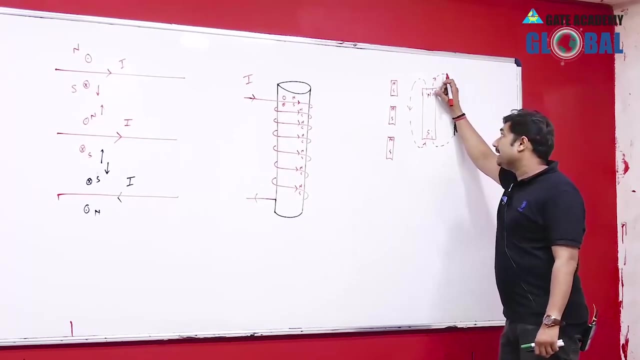 to south. It always leaves from north into the air and always receive from air to south. If this is a magnet then you can say this terminal is north. From the north terminal of the magnet flux releases into the air and from the south portion of the magnet. 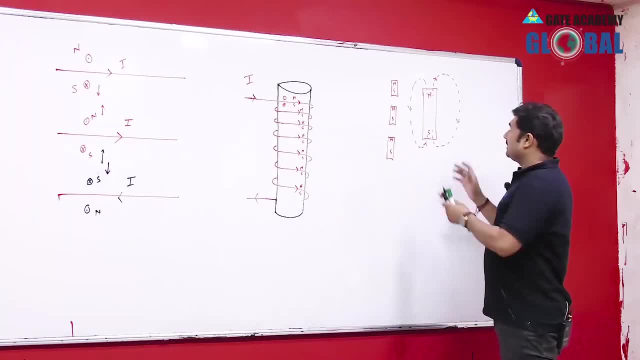 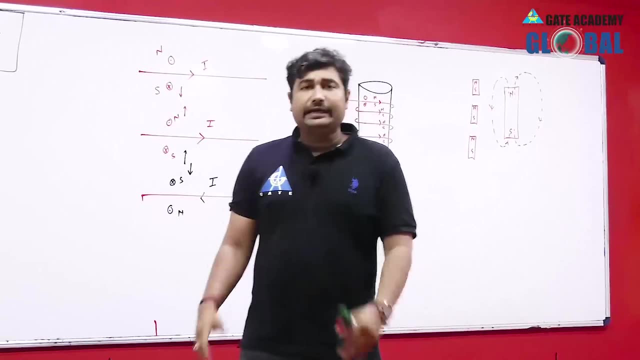 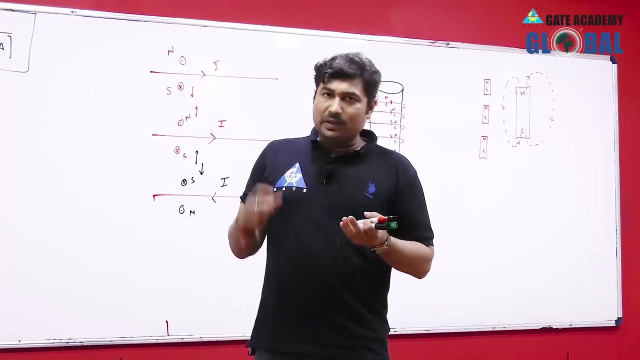 flux enters from the air. You can say, sir, why always the magnetic line of forces are represented in this way? You can observe these magnetic line of forces physically. How, sir, This is possible? Take a plain paper, use one magnet, take iron powder and spread all around. You found. 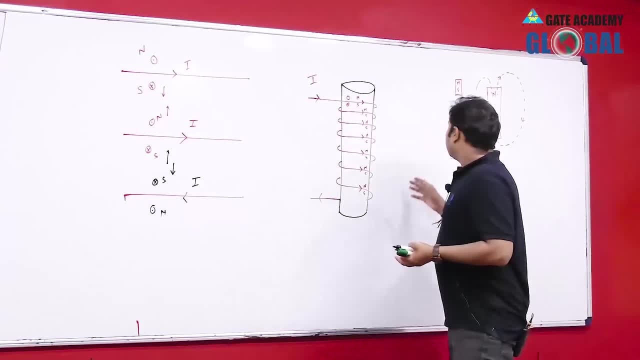 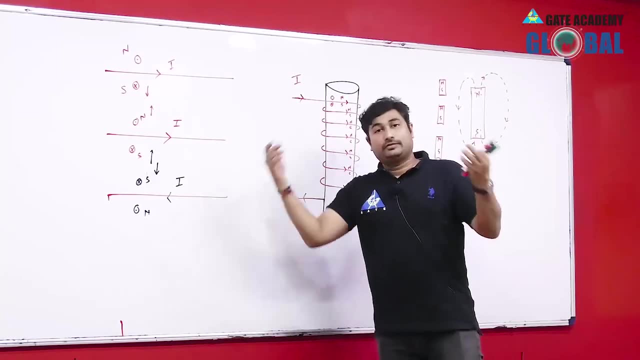 them to be Both magnet and magnetic. If you have the magnetic line of forces, they touch that, the iron powder is going to take this path. The iron powder is going to take this path and you can clearly see the magnetic line of forces, how the magnetic line of forces 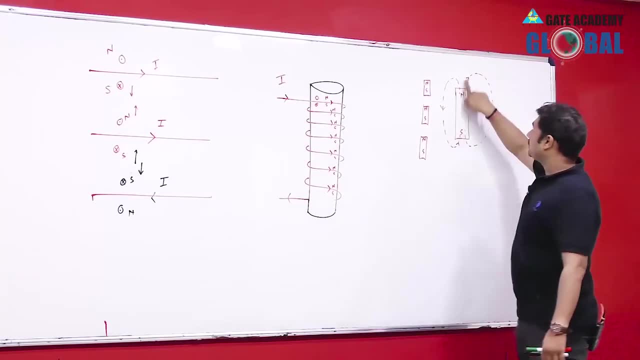 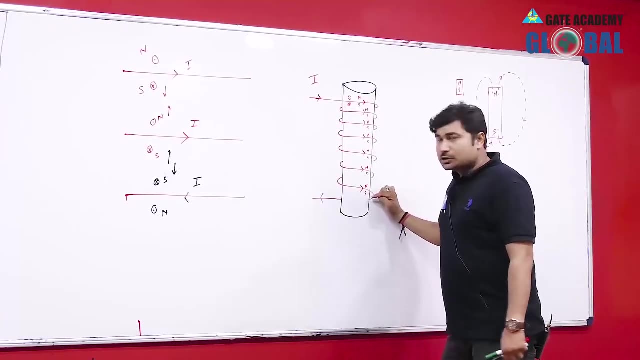 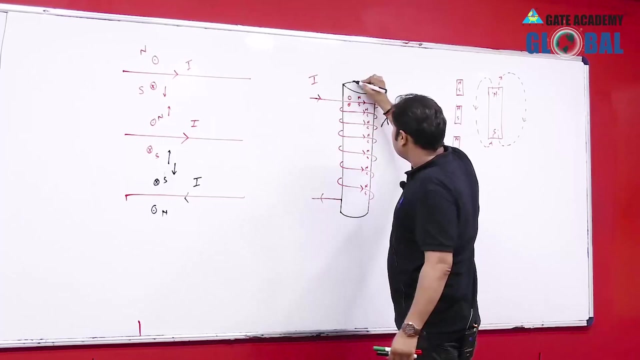 are going, Is it ok? So magnetic line of forces always flows from north to south. You can say, sir, these are all small magnets So combinedly they can act as a magnet. this entire core will going to act as a magnet. now This portion of the core is going to. 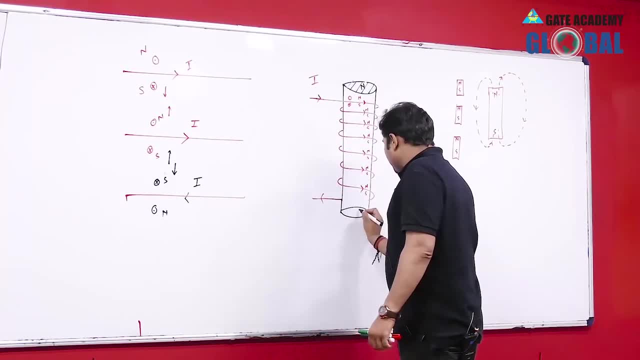 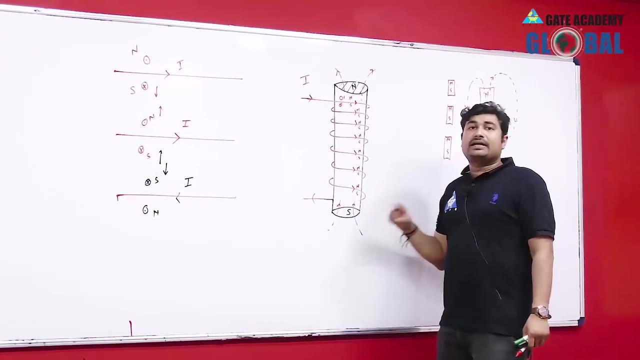 act as a north and this portion of the core is going to act as a south and the magnetic line of forces are appearing in this fashion: coming out from the north and again receiving from the south. So one can say, sir, the current flowing into the wire will produces a magnetic 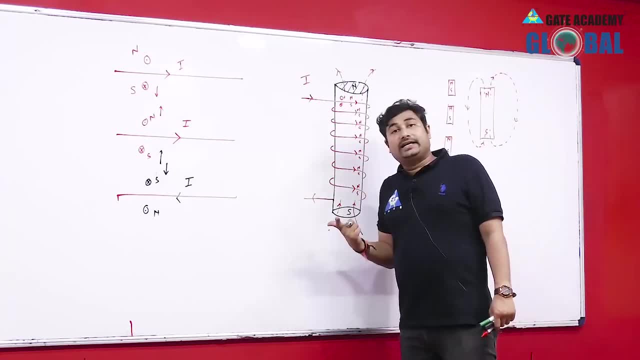 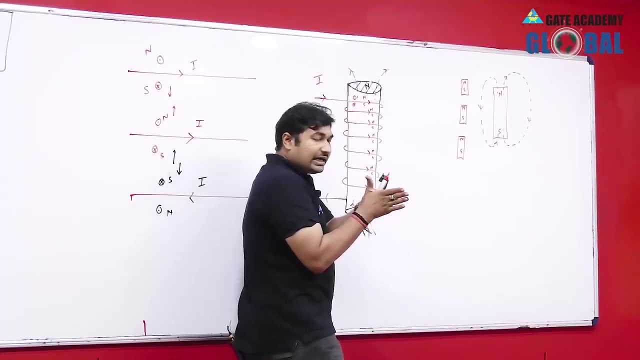 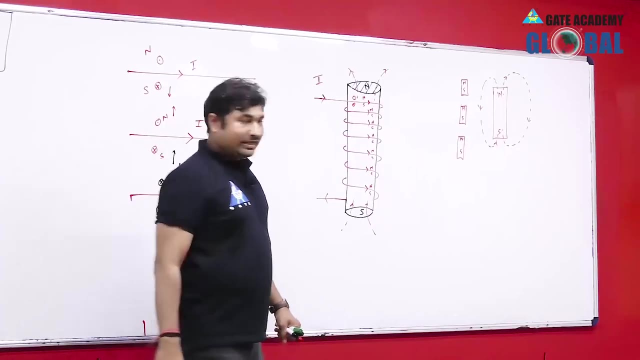 field, and we can also find the magnetic field by the right hand grip rule, Instead of going each of the wire separately. we can use in this fashion: If the direction of current is represented by curve, Then one can say thumb will represent the direction of flux, If the direction of curl. 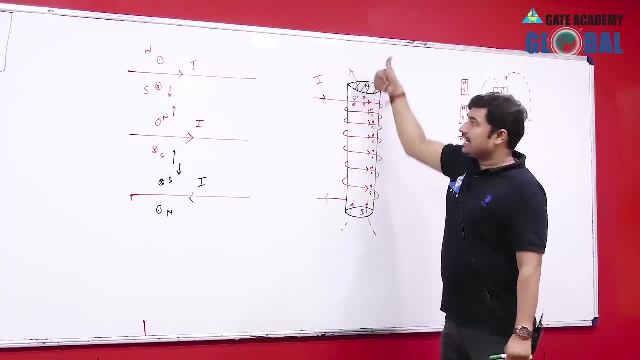 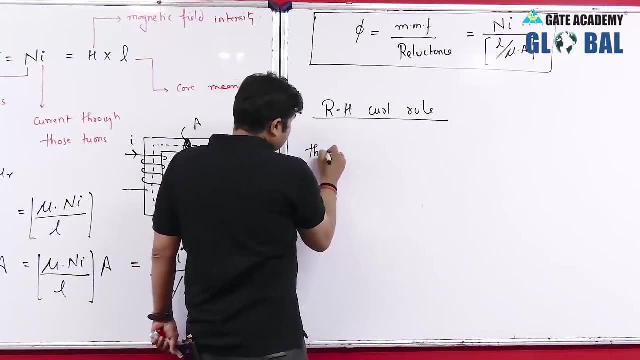 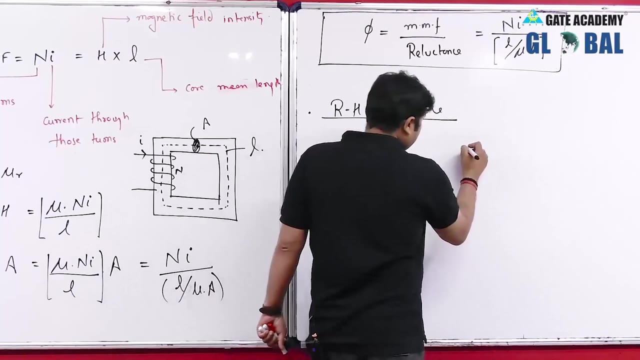 is represented by the current, then thumb will represent the direction of field. So this lead to the conclusion that, sir, if thumb is representing the direction of current, then right-hand curl will represent- Let us think and see- apartments in the room. 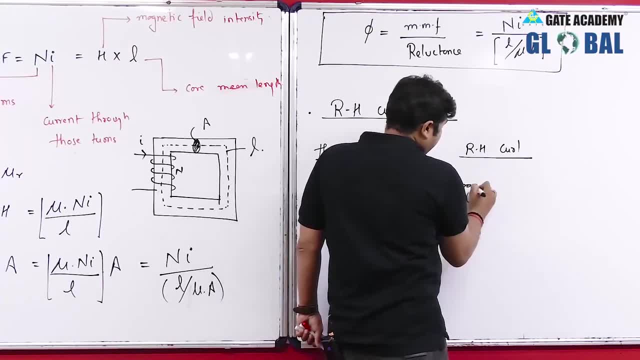 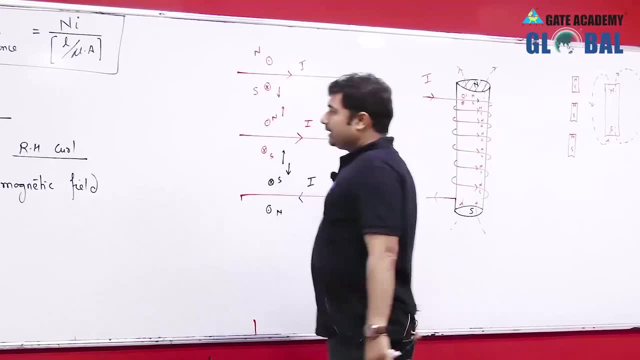 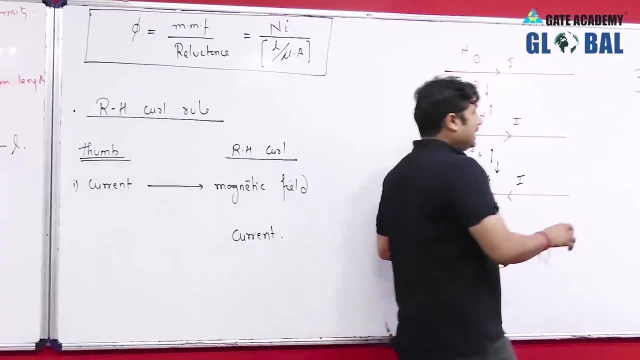 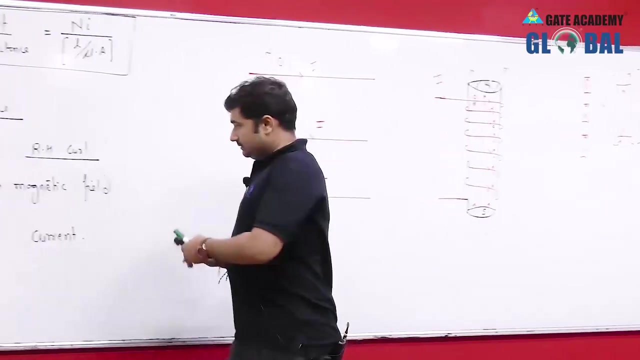 represents direction of magnetic field, as I explained in this section, And if the right hand curl is current. if the right hand curl is current, as I explained in this section, if the right hand curl is current, then thumb will represent the direction of field. 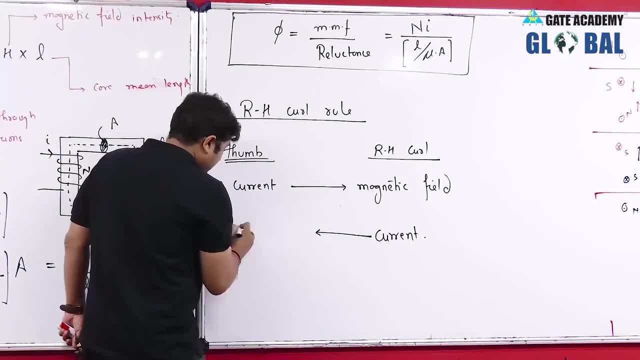 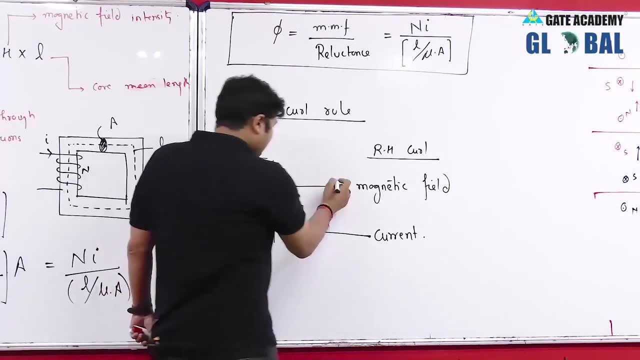 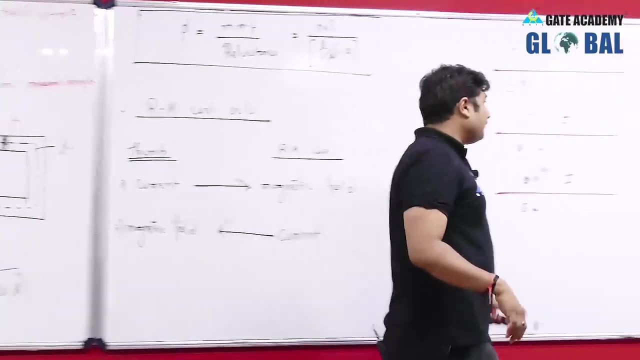 Then thumb will represent the direction of magnetic field. Both time I have represented the arrow towards the field side. So if you know about the direction of current, you can easily find the direction of field. One can say, sir, it also going to be affected by the way how the windings are going to be. 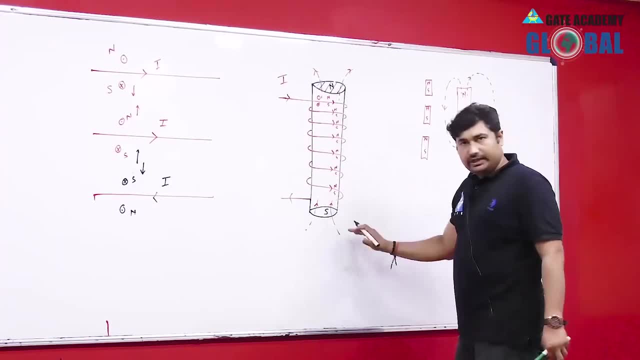 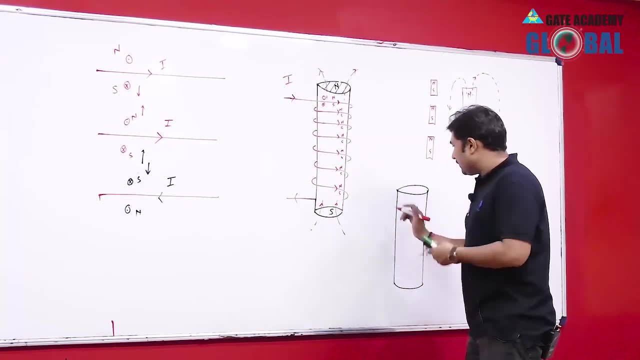 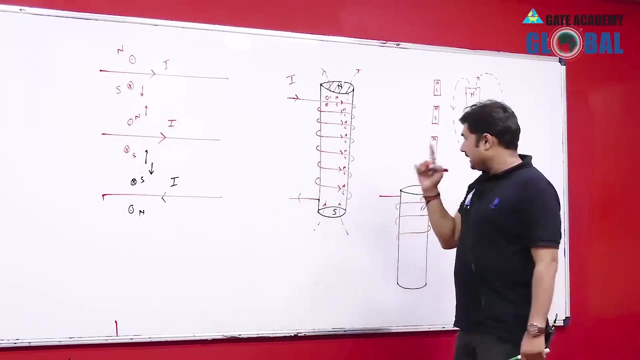 bounded onto the core. Let us suppose the same core. We have the same core. Let us again suppose we have same core And on the same core the wires are bounded in this fashion. It means previously I have bounded the wire in this clockwise fashion. 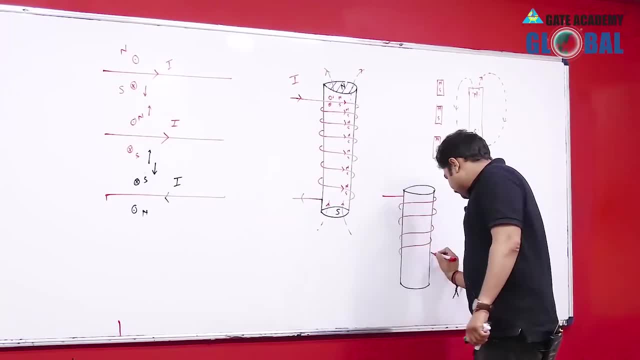 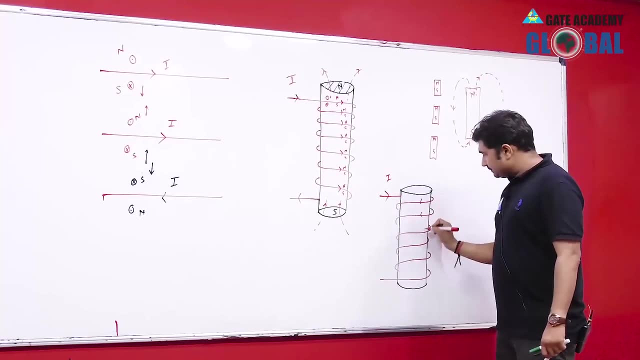 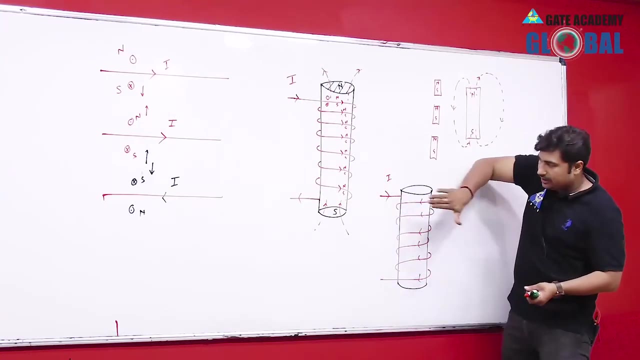 And now I am going to bound the wire in anti-clockwise fashion. If the wires are bounded in this fashion and current I is supplied, then the current will flows in this way. Now, please use right hand grip rule. If the direction of current is curl, then you can say thumb will represent the direction. 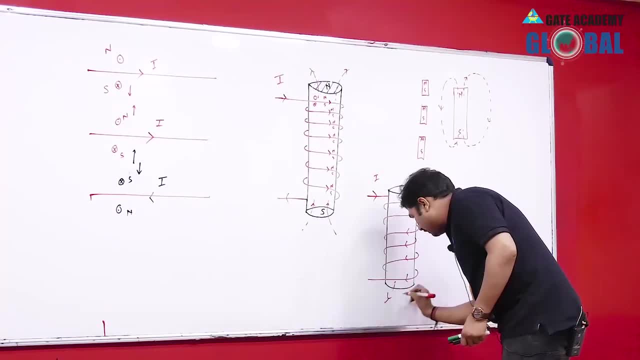 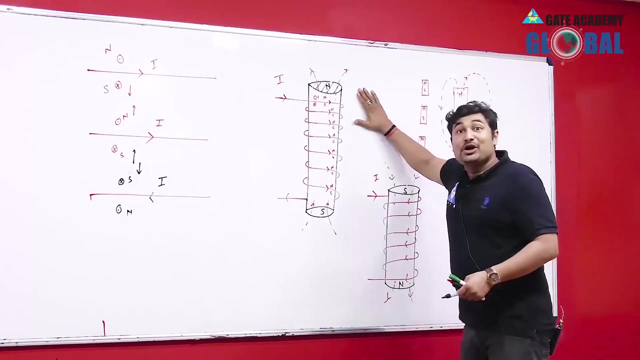 of field And one can say magnetic line of forces are appearing to be coming out from this portion and going into this portion. So this will going to act as a north now and this is going to act as a south now. It means not only the, it means not only the direction of flux is dependent to the direction. 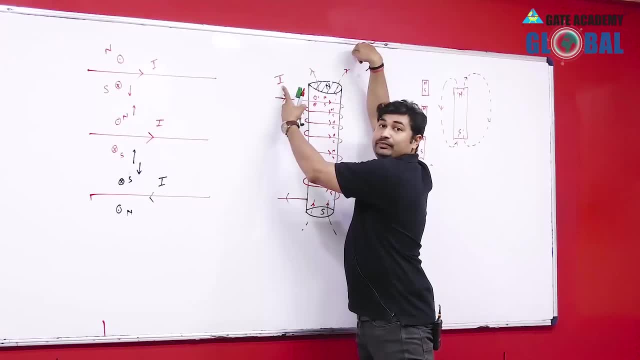 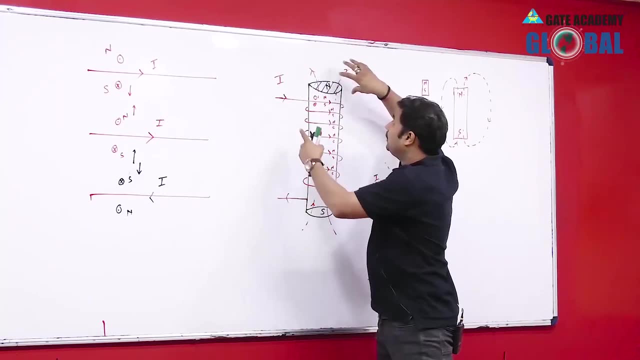 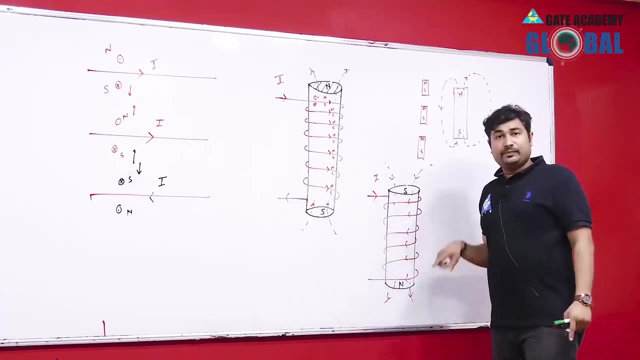 of field. It is dependent to the direction of current. Not only the direction of flux is dependent to the source, current direction, but the polarity of this. polarity of this magnetic field depends upon how the windings is bounded onto the core, Whether the windings are bounded onto the core in a clockwise fashion or whether the 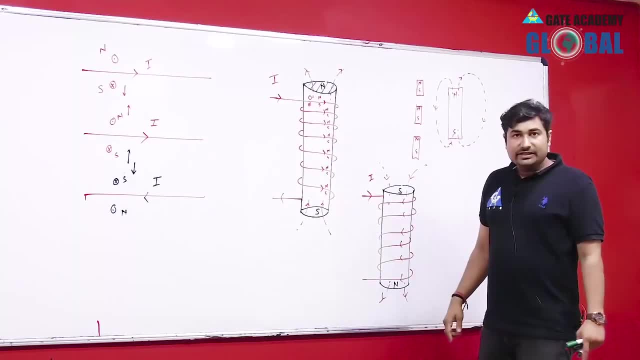 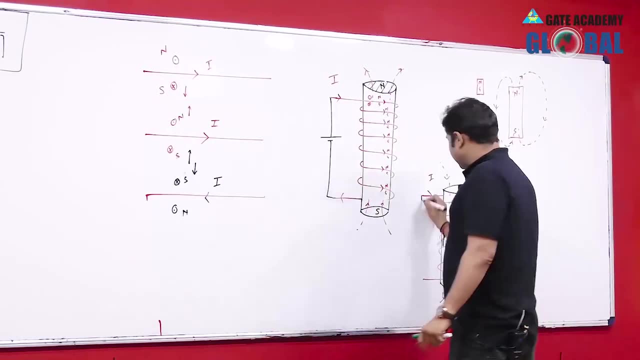 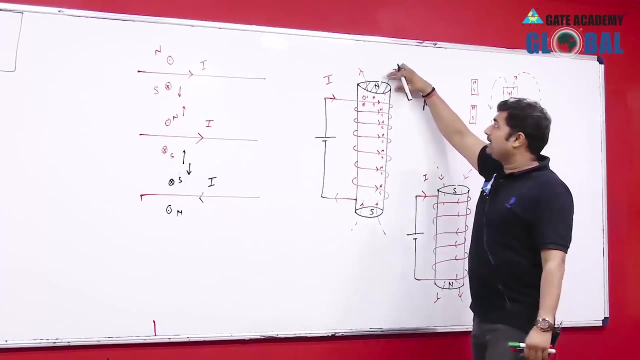 wounding windings are bound onto the core in an anti-clockwise fashion From the same source. both are supplied From the same source. You can say: sir, Let us suppose we are supplying DC, So we have this as a electromagnet of permanent polarity of this of permanent. you can say: 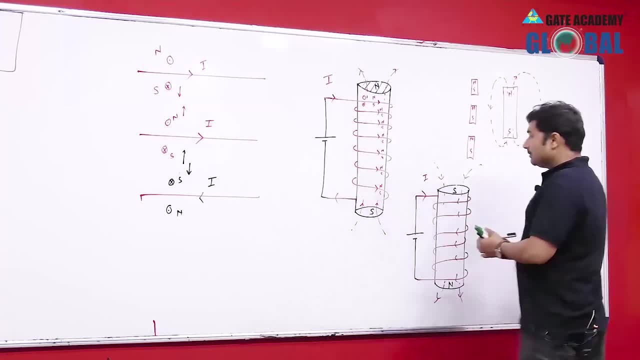 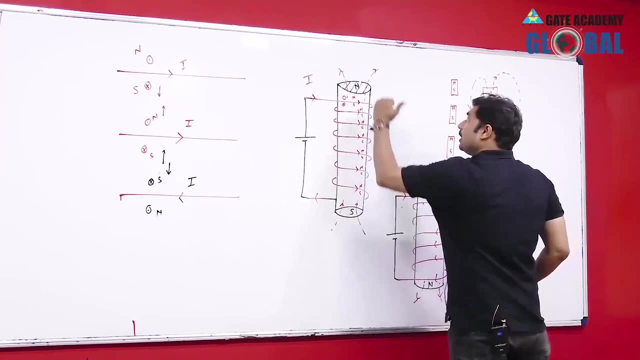 unidirectional polarity, this to be north and this to be south. From the same source, from the same polarity, we are supplying to both, But in this case, the top one is acting as a north and this case, the top one is acting as a south. 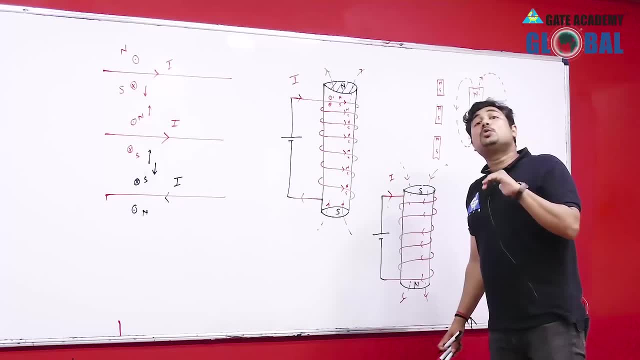 It means the MMF direction is not only dependent on the polarity of the current. It is acting as a north. It is acting as a south. It is acting as a south. It is acting as a north. It is acting as a north. 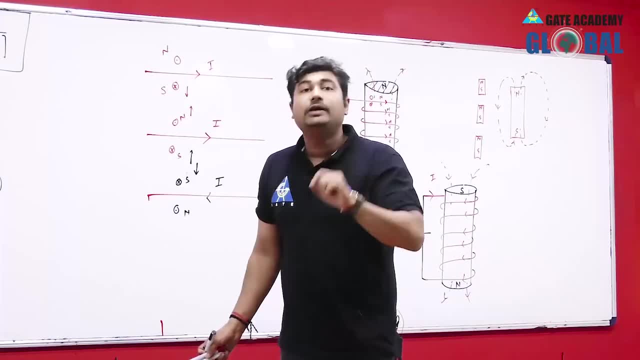 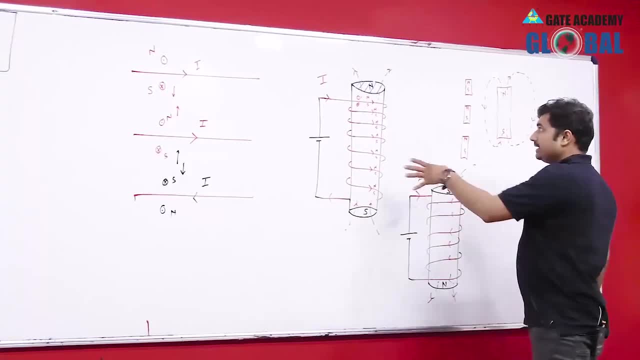 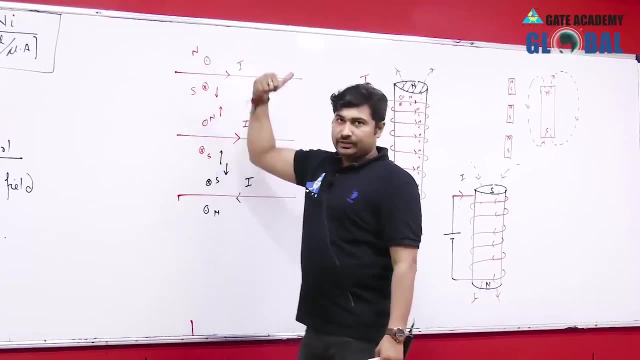 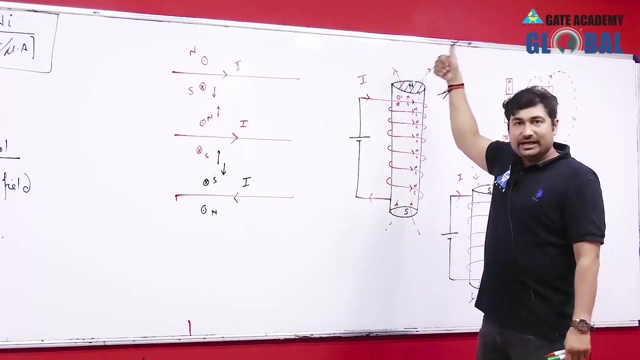 Now I am hoping key this concept is delivered to you- that right hand curl rule: If the direction of current is thumb, then curl will represent the direction of flux. If the direction of current is curl, then thumb represents the direction of flux. Is it ok? 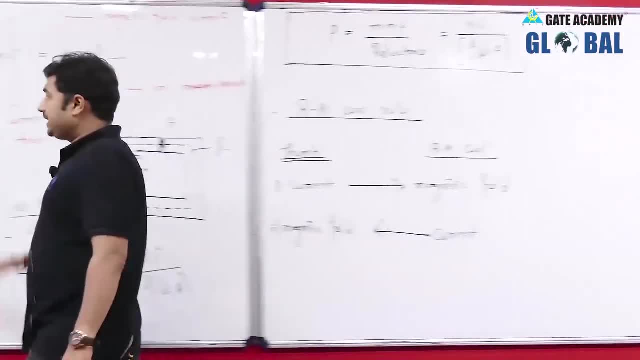 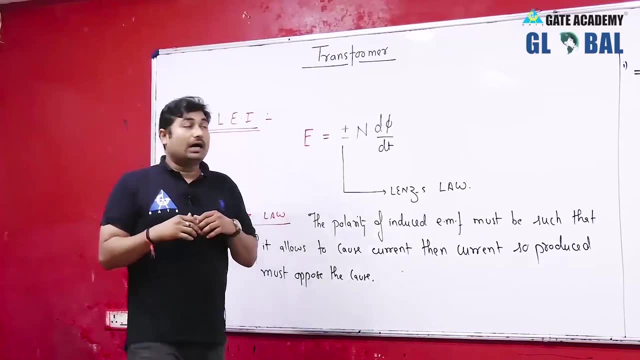 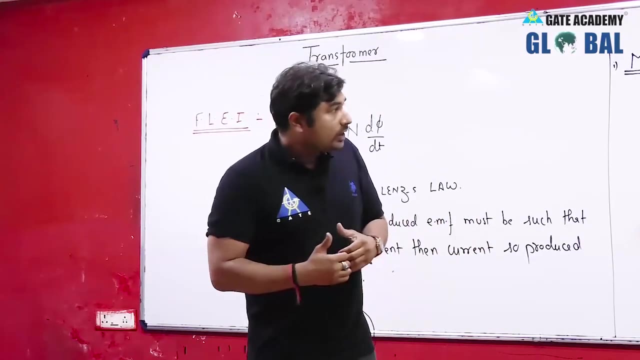 Ok, So we have the concept. It is a basic concept is needed to understand the working principle of the transformer. Now we know how the windings wound on to the core is going to affect the polarity of magnet on to the core also from.